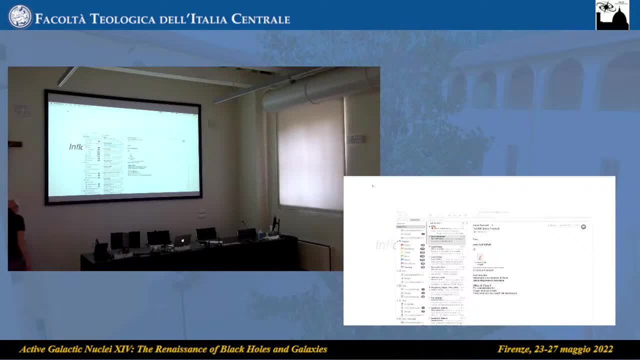 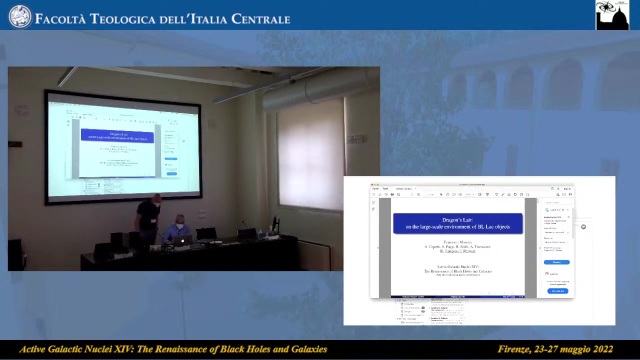 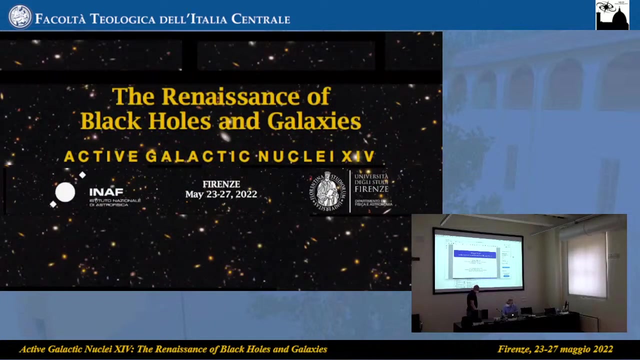 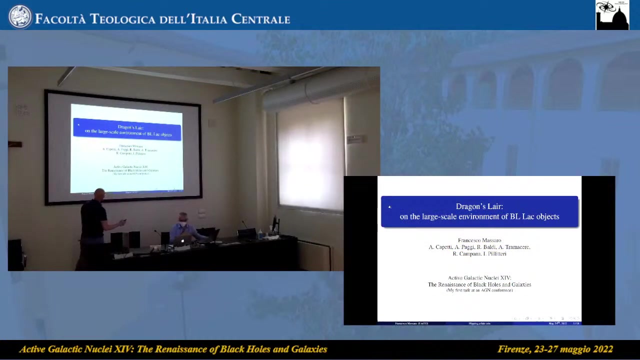 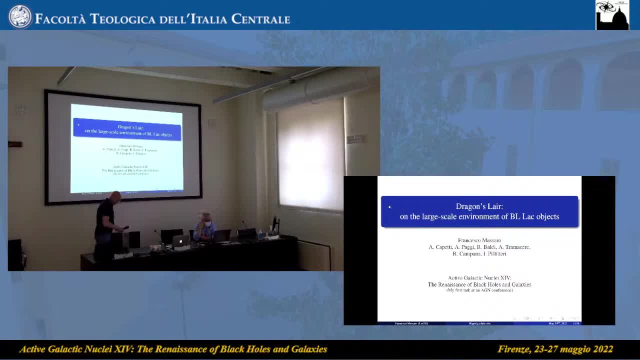 The first talk is by Francesco Massaro, Dragon Slayer, on the large-scale environment of BLG. Okay, Does it work? Yeah, Okay, great Thanks. So thanks a lot. Thanks to the organizer for the very nice conference. I just arrived. 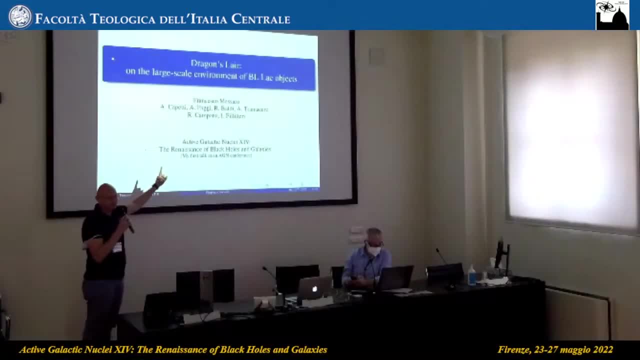 And I wish to start thanking all the collaborators. I mean, without their help, I would have never done this. This is the story of a discovery that took me about three years- Sorry, 10 years- to carry out, And actually this is my first talk at the NGN conference. 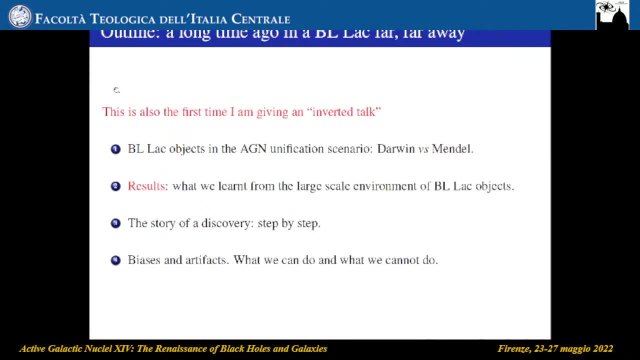 And see: Okay, This is also the first time I'm giving a sort of inverted talk. Okay, I will tell the question we want to answer, I will tell the answer And then I will try to convince you about the analysis we carried out. 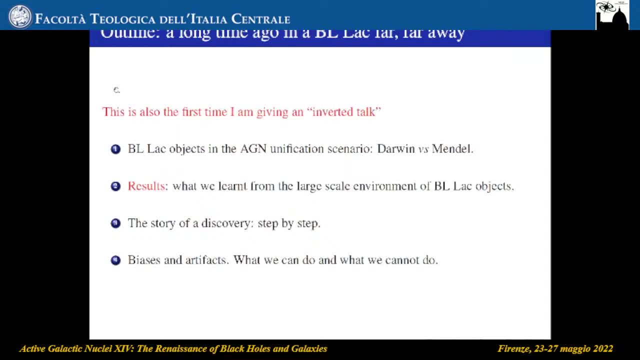 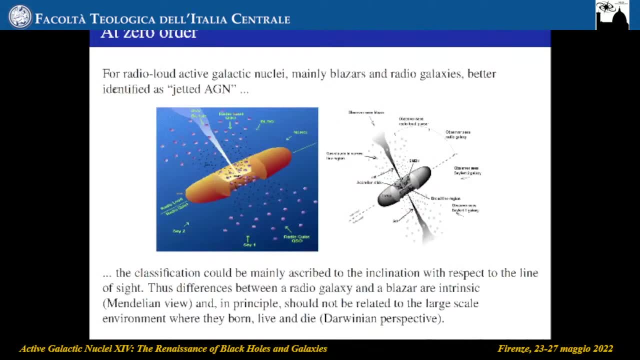 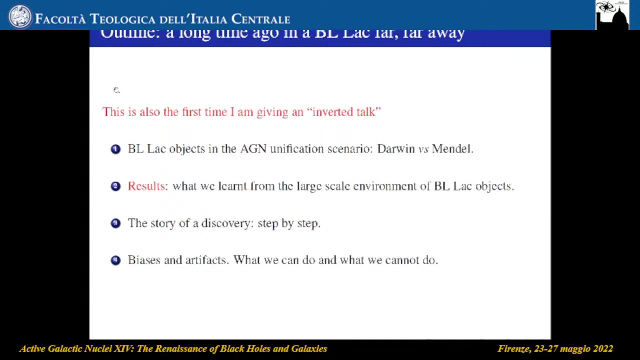 Probably I suffered too much the influence of one of my collaborators that was pushing me, That was pushing me to make things very neat. Okay, Sorry, The outline of the talk is this one And of course I mean I will just briefly overview the BLH in the NGN unification scenario. 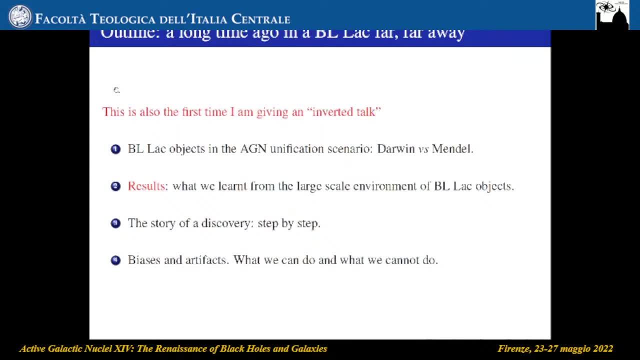 talking about environment and intrinsic properties, Then I will give you the results, what we learned from the large-scale environment of BLHs, a sort of test for the NGN unification scenario- And then, step by step, some of the biases, the artifacts we have been found during the analysis. 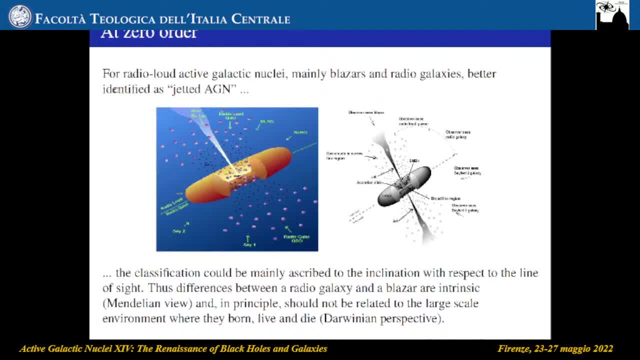 I couldn't start the talk without the classical plot of the NGN unification scenario And I mean I just want to focus on blazars and radio galaxies, so only on radio-loud AGNs, And in particular I want to focus on BLHs and radio galaxies FR1 type, the edge darkened ones. 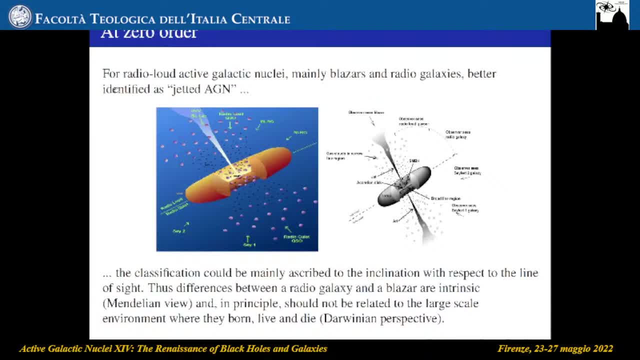 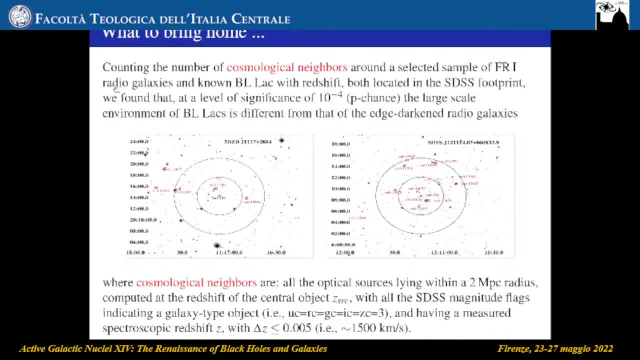 And they at the very very end. you're going to see a radio galaxy. And they at the very very end. you're going to see a radio galaxy, actually in environments that are richer, And this is the result. 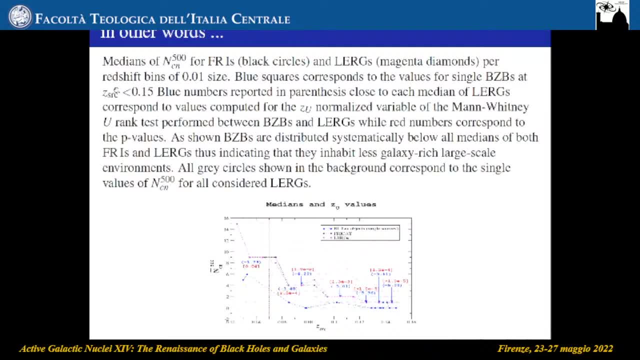 So in this plot you're going to see a measurement of the richness. This is the number of cosmological neighbors. that means galaxies with the same redshift of the central galaxy. This is the median value within 500 kiloparsec, And we did this in 500 kiloparsec, 1 megaparsec and 2 megaparsec. 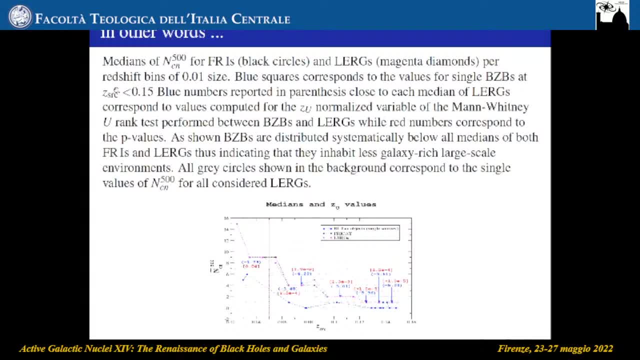 This is the median value as a function of redshift. The blue dots here are the BLX and they are systematically below the radio galaxies. These are these other dots. They are for one radio galaxy. We also did a test for the LERCs. 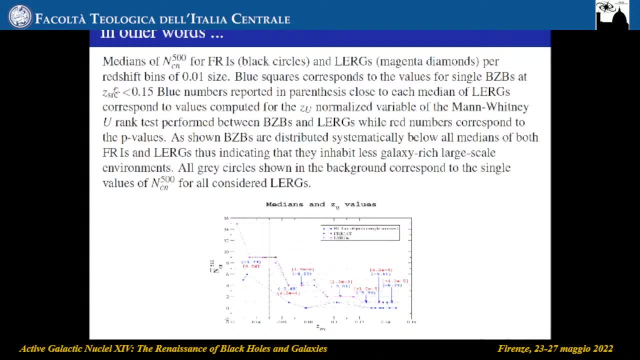 so for the low-excitation radio galaxies- And I want to highlight this- plot must be seen from this direction. So it must be seen redshift point per redshift, redshift bin per redshift bin. You can see this. You cannot compare this systematically. 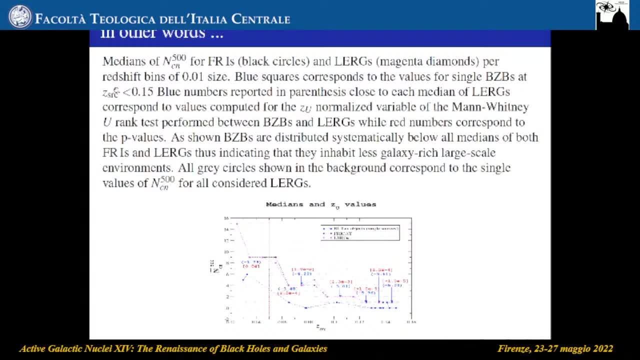 You cannot compare the entire sample because the richness when you estimate a certain redshift is completely different from the one that you can estimate direct shift. So the solution of the problem if the BLX are not the counterpart of the FR1 radio galaxies- 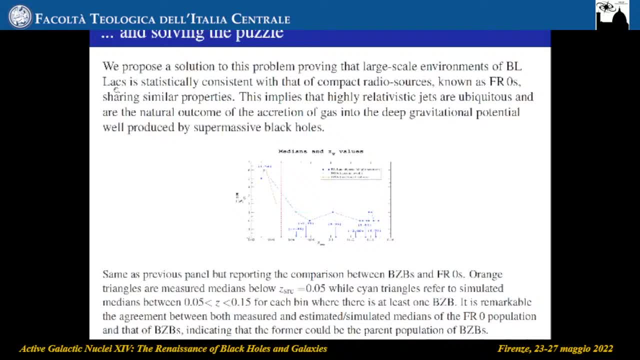 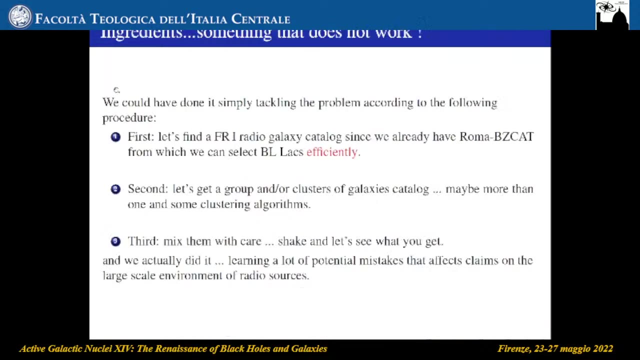 then what are their counterparts? And the solution is they are very, very similar to the FR0s. So radio galaxies lacking extended emission of the order of 10 kiloparsecs, just bright spots in the radio And sorry pointing out. 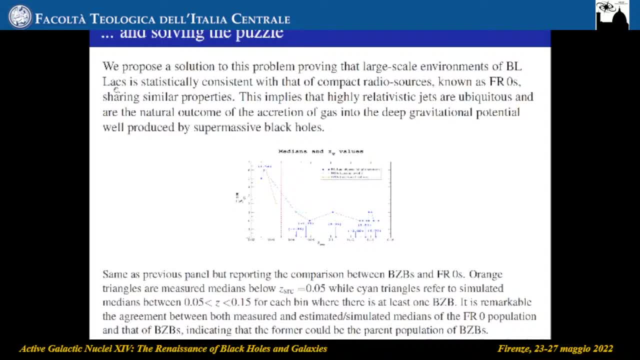 this is the same plot before and this is BLX and almost the same line. For the statistical analysis, we carried out a man-with-na test in order to compare the medians. It's a non-parametric test, a rank test. 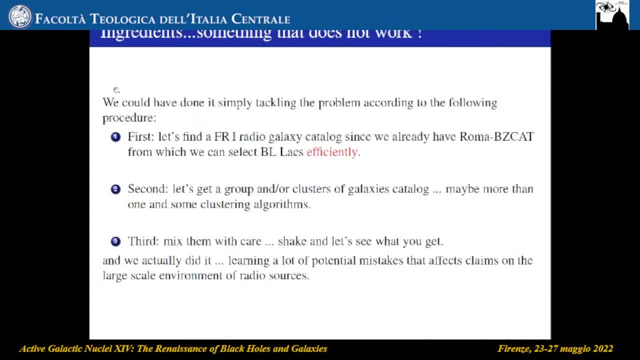 Okay, now how to carry out the analysis. A friend of mine a long time ago suggested to do this. You take a radio galaxy catalog, you take a galaxy cluster catalog, you shake them, you make the comparison between radio galaxies. 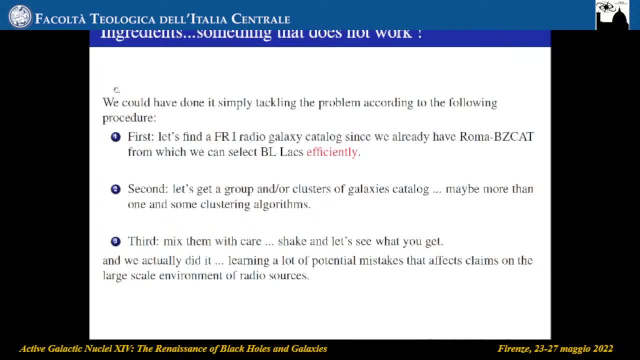 how many radio galaxies lie in galaxy cluster. then you repeat the same for BLX and then you can find an answer. This is not possible. First of all, the main problem we found is there is no radio galaxy catalog on FR1s. 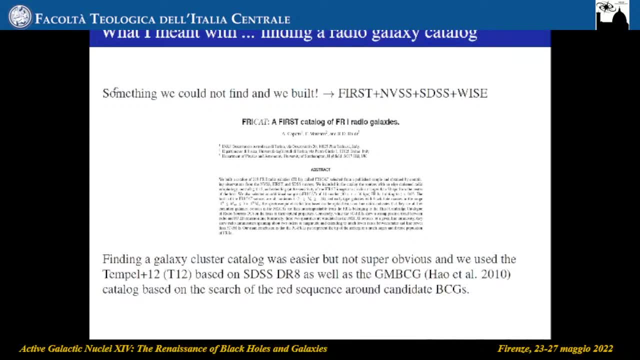 So a long time ago we had to build the radio galaxy catalog. Then we need to find a galaxy cluster catalog and there are several in the literature. And this was another another problem, Because the radio galaxy, the galaxy cluster catalogs. 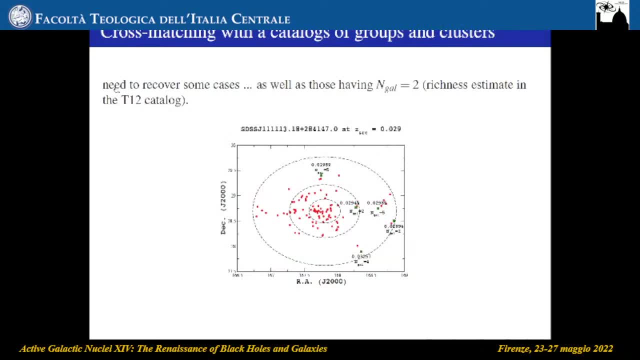 they can have uncertainties and they can have biases. they can have artifacts in the algorithm used to draw the galaxy clusters. This is one of the worst examples Actually taken from what I believe is the best catalog of galaxy clusters I found in the Sloan footprint. 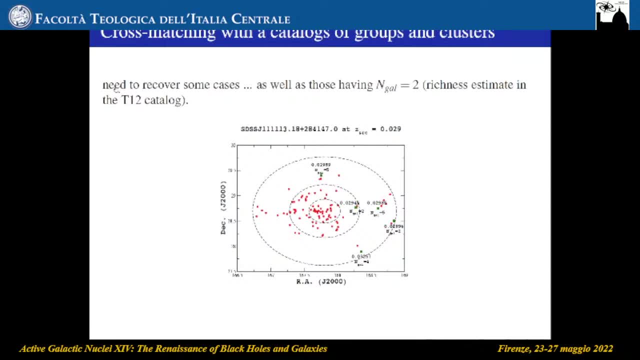 So the red dots that you see with the redshift at the end, are just the galaxy clusters found by the automatic algorithm and the angle is the richness given in the galaxy cluster catalog, While the red dots that you see, the red dots- are just the source. 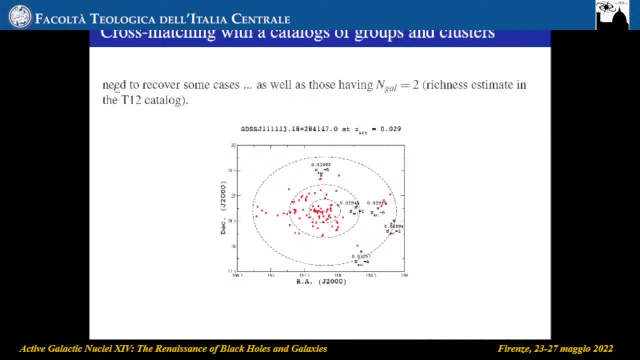 the cosmological neighbors. So the source is with the same redshift of the central objects within five, 10 to the minus three in redshift difference. So you see completely different position and the cluster is basically broken. okay, So you need to recover this before you can do this. 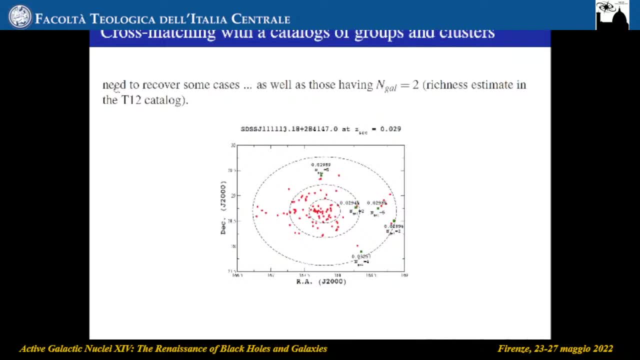 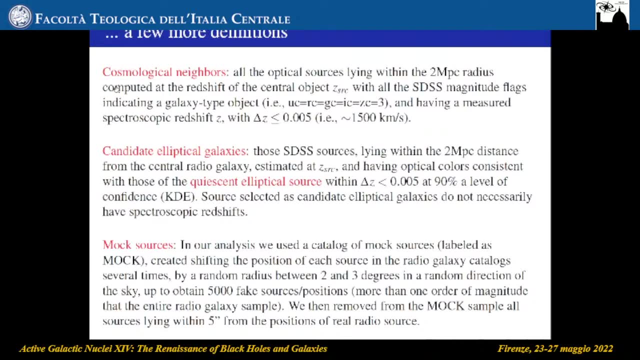 So you need to recover this before you can do this Before using the catalog And you need to check source by source. That's what we did. Let me skip this. So we have been building this kind of plots, So central radio galaxy or central BLH. 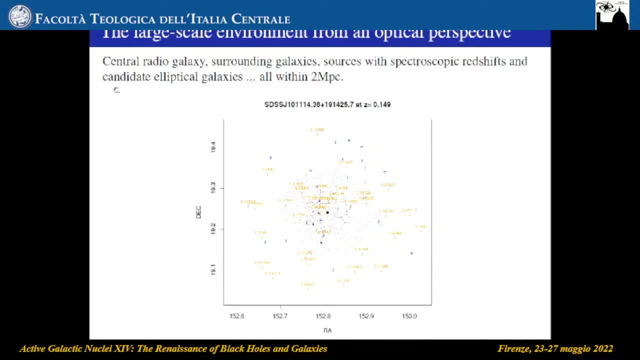 all the sources with the redshift and we have been checking all these plots for all the radio galaxies and all the BLHs in the sample we compared. In addition, even if I'm not gonna show this, we also test the red sequence. we also test the different. 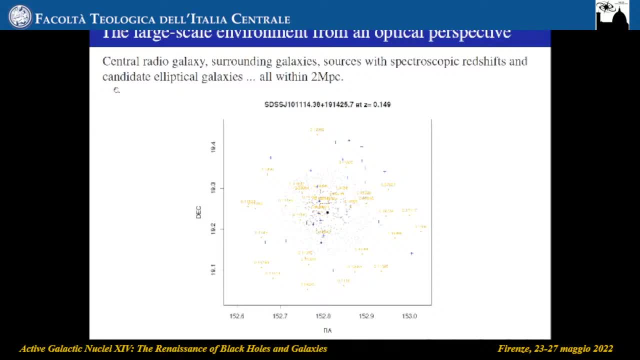 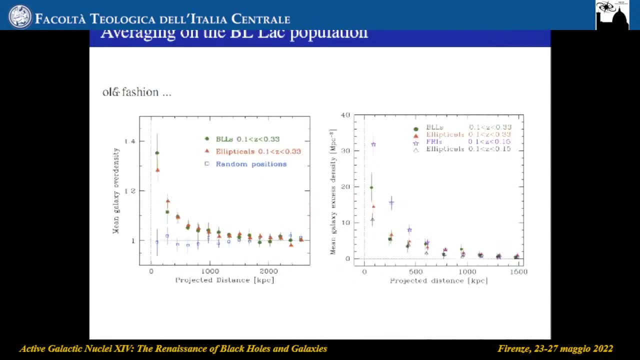 we also test the different clustering algorithm, like the BSCAN, MST, all the same results. This is something that you cannot do and people did in the literature, old fashioned. You can count the magnitude, you can measure the magnitude of the central galaxy. 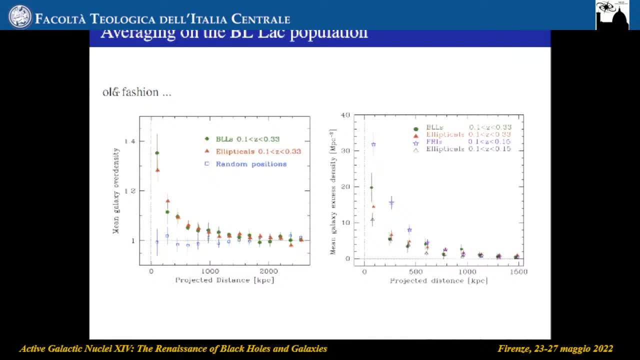 and say something like plus two and then count all the galaxies around within a range of magnitude and then you can average an excess or an overdensity of galaxies around the central object. Okay, this cannot be done, especially if you wanna take the entire population. 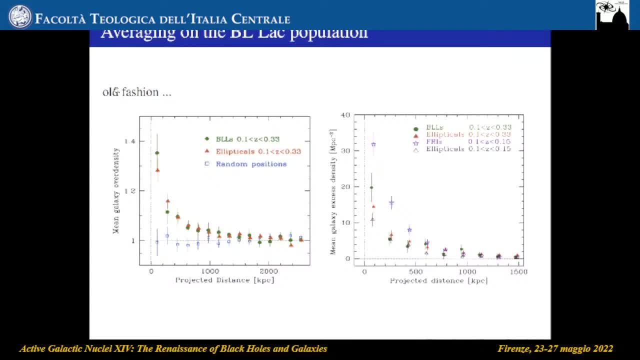 and claim a systematic excess, as they've been doing. In the y-axis there is the projected distance. this is the excess of galaxies around BLHs or radio galaxies. This cannot be done. The reason is this: if you compare objects, 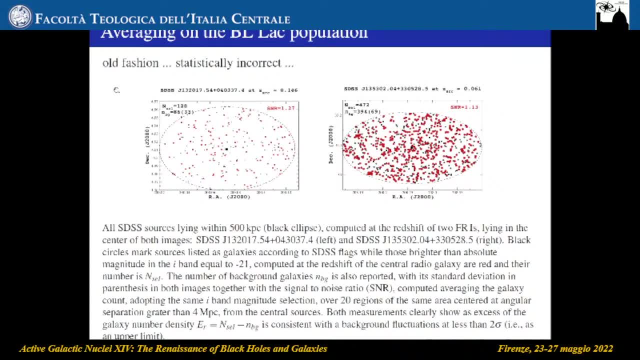 the central objects. they have a different magnitude, a different redshift range. this means that the signal too is not the same. The signal-to-noise ratio is different. So you are comparing objects, a different signal-to-noise. 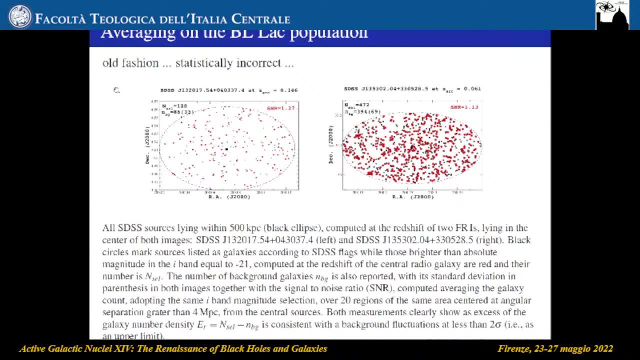 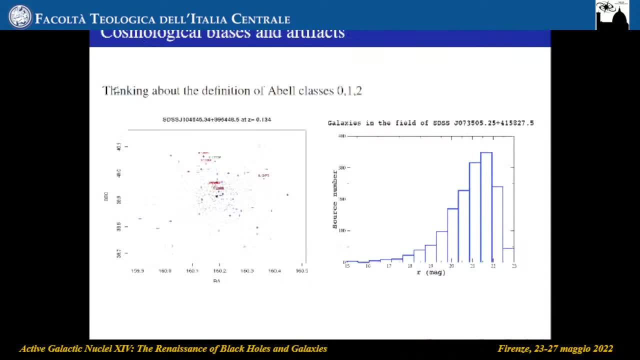 So this is statistically incorrect. Something else that cannot be done, something like classes for the richness: If you take the central object and you change the magnitude of the central object, the number of the galaxies around will follow that magnitude and the magnitude is changing. 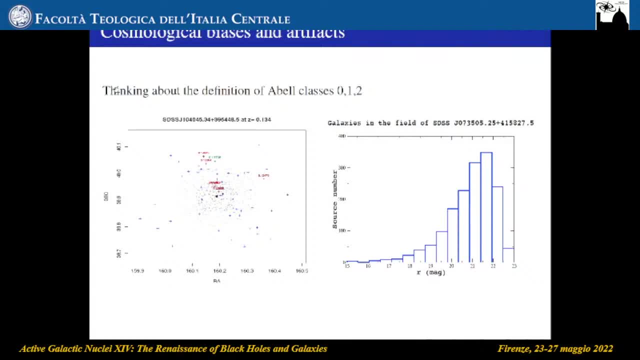 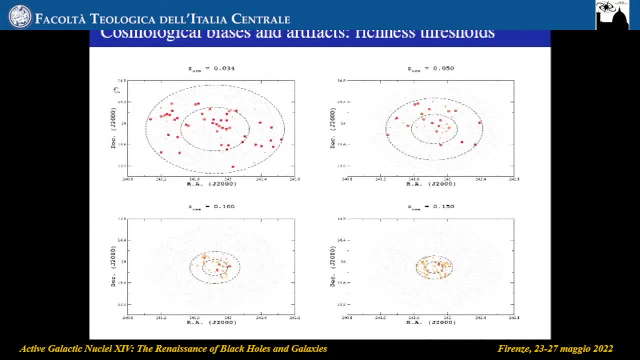 So you cannot compare objects in this way. You can only do this per redshift bin. And this is my last slide, This is something else. If you take a cluster, a redshift 0.034, all the red dots are the cosmological neighbor. 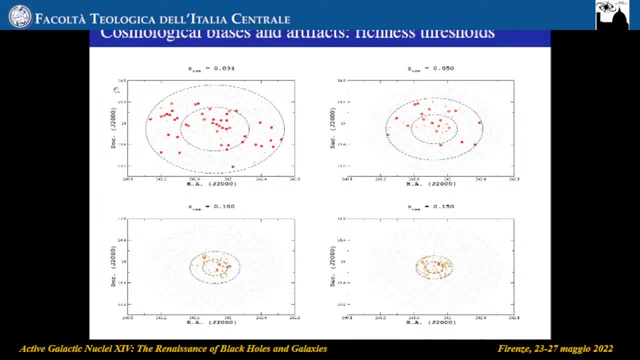 sources with the same redshift of the central objects and then you move a redshift- 0.15, and you take into account the cosmology fixing the luminosity. this is what is happening: Just one source within a central region of 500 kiloparsec. 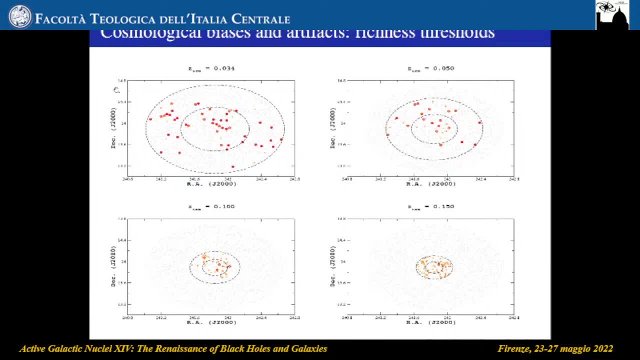 This is why you need to take into account a redshift, And you can do it, but you can't do it in the same way. You can't do it in the same way that you did in the first place And you can't do it in the second place. 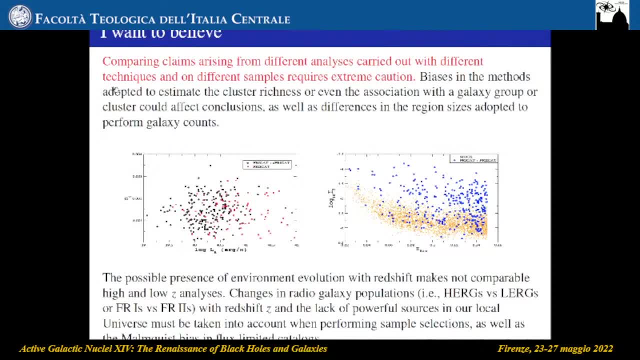 which is why you need to take into account a redshift, And this is why you need to take into account a redshift, And it's not just a redshift. And in fact, for example, this is an estimate of sigma-5, one of the usual parameters to account for dark matter halos. 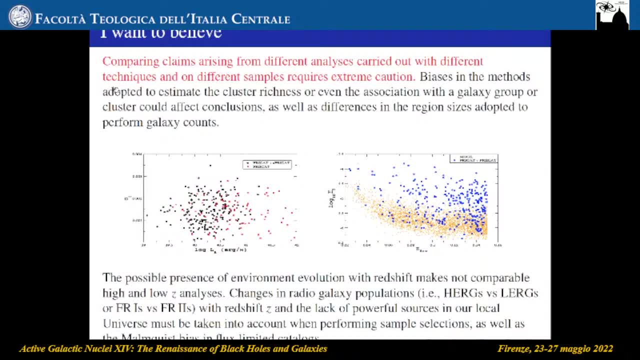 This is redshift dependent, so you cannot compare sources unless you do this in the same redshift bin. If you compare the entire population, it makes no sense. This is why you cannot compare FR1 and FR2 radio galaxies, because they have different luminosity. 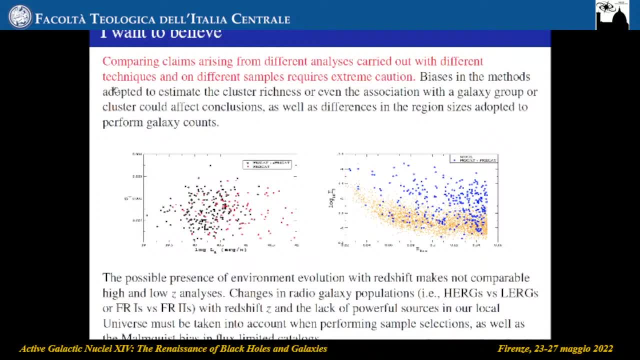 If you take a survey of the sky, then you will find that all the FR2s will be higher redshift, higher luminosity, and so you will always see a dichotomy in the plot: These are FR2s, these are FR1s. 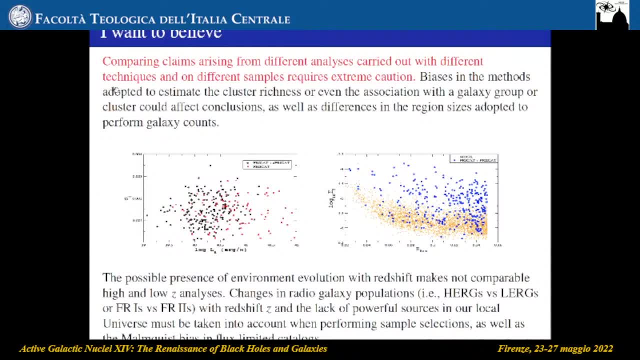 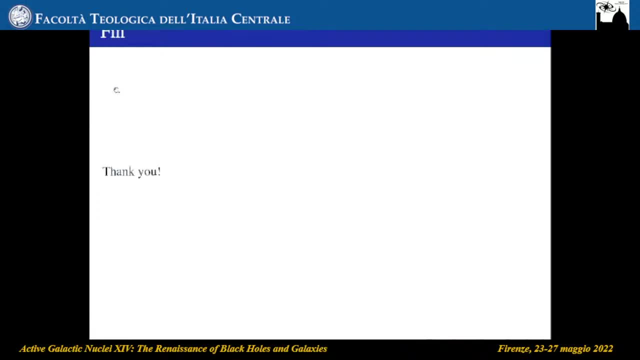 So the only way to do it is really counting sources with a spectroscopic redshift. That's it, Thanks. Thanks, Francesco. Perfect in time. So questions for Francesco. Hi. so the question is: why didn't you just compute the cross-correlation function between galaxies and your radio sources and do the halo model? 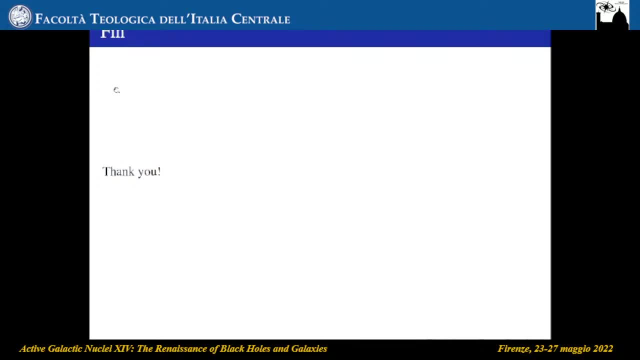 So you got the occupation number as a function of the halo mass and so you would probably get a more complete view. You mean the two-point correlation function for clustering around. Yes, Yeah, yeah, no, we did it. We did it as the MST, as a dB scan, and we got the same result. 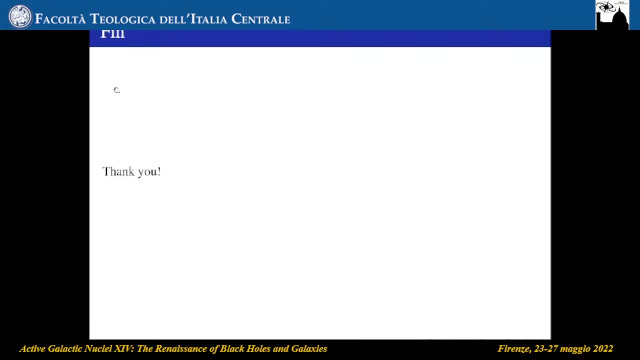 The point is that it's not as strong as using redshift, spectroscopic redshift. Well, in principle, you do right with the correlation function, with the 3D correlation function, and you also reconstruct the number of objects within the halo. 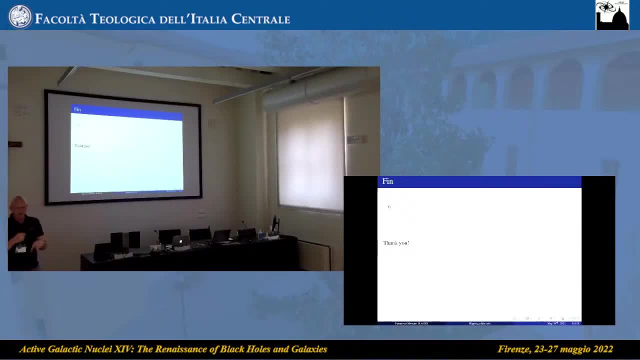 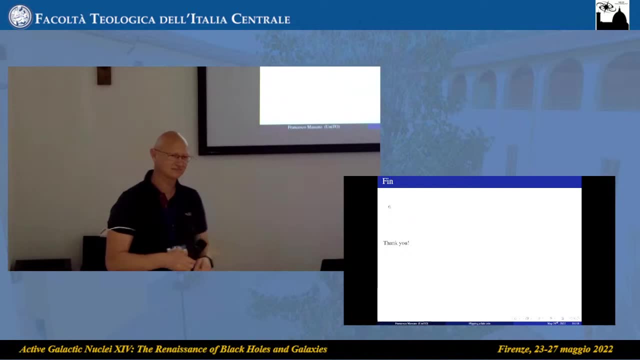 It's much more powerful, probably. Yeah, yeah, using coordinates and spectroscopic redshift. No, no, we have been trying to do this. We just did not close the analysis on that. Yeah, Other questions for Francesco? I just have a curiosity if I missed it. 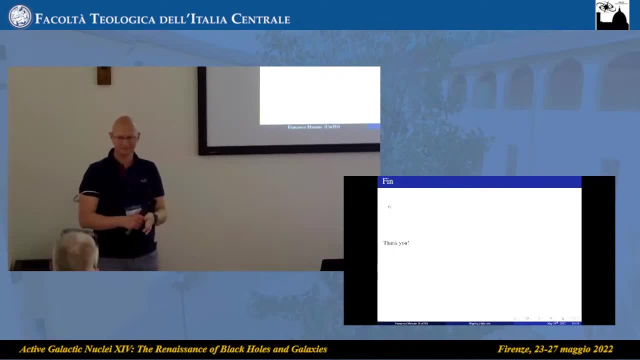 So what is the implication on the physics of the sources? if there is a difference, What is the implication on the physics of the sources? Ah, okay, no, Okay, the environment is not playing the major role. I mean on the sources, okay. 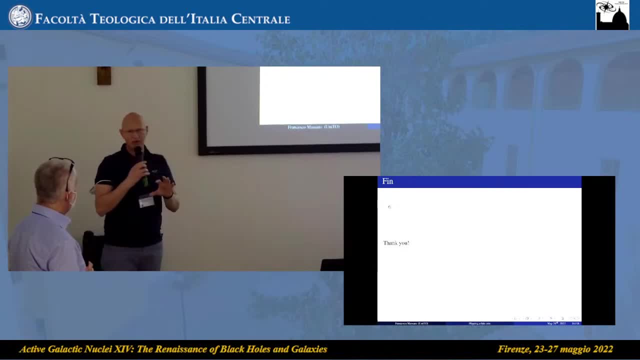 So I mean they- First of all, BLX- are different from FR1s, so you don't expect to diffuse emission in the radio. okay, That's the major point. And different physics. I mean you're looking at different objects than the one you were expecting before. 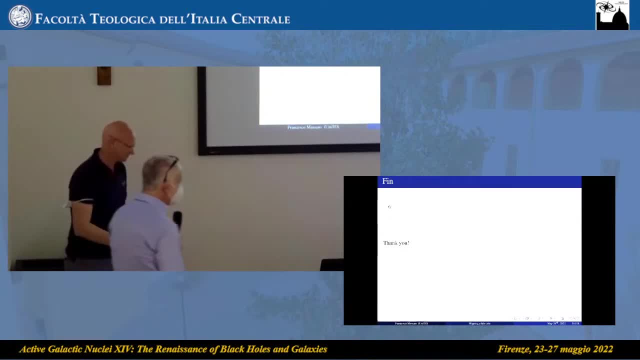 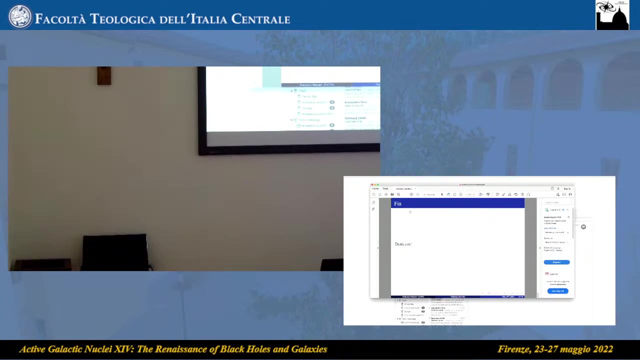 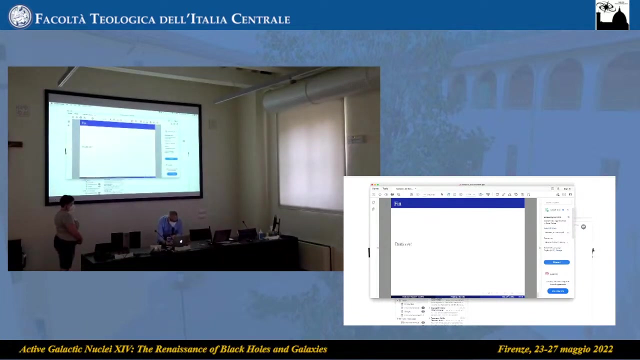 Okay, Okay, thanks again. Let's thank Francesco again. Thank you, And now, Okay, now we have He. It's a garland. Where is your Okay? I'm searching for your Okay, so I found it. 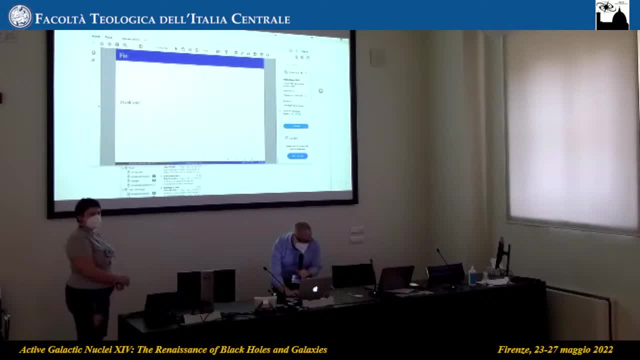 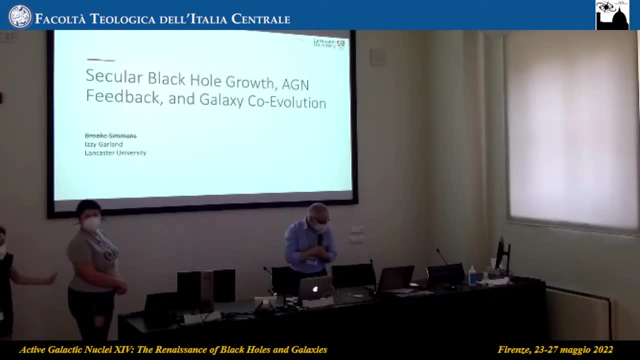 Okay, Okay, Okay, Okay. I think the title Okay, Okay, Okay, Okay. So we have, Okay, so we have, Okay, so we have. So we have a change from the, From what is written in the. 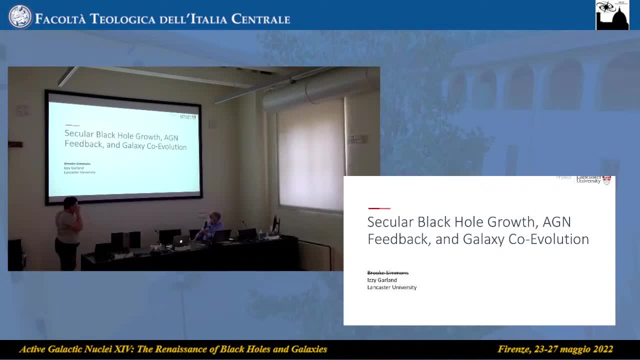 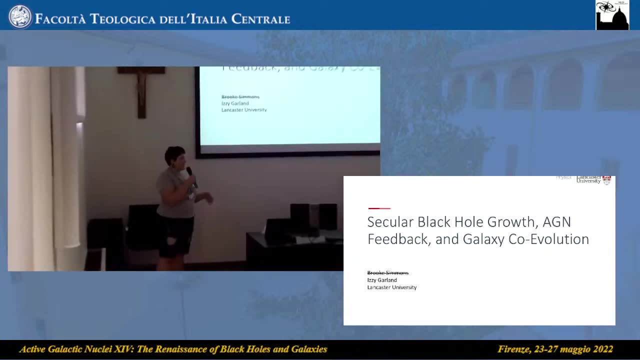 In the program. So we have It's a garland with secular black hole, growth agent feedback and galaxy revolution. Please, Thank you very, Yeah, cool. So thank you very much for having me. As you've probably gathered from the programs, 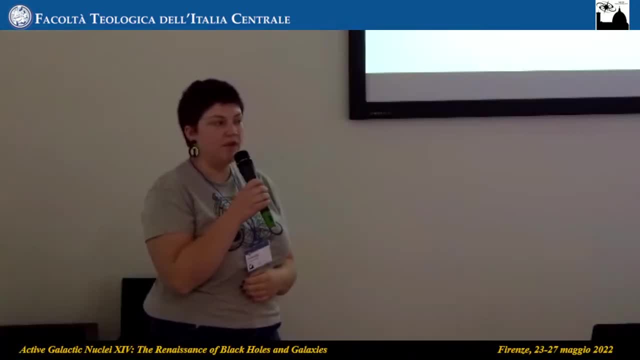 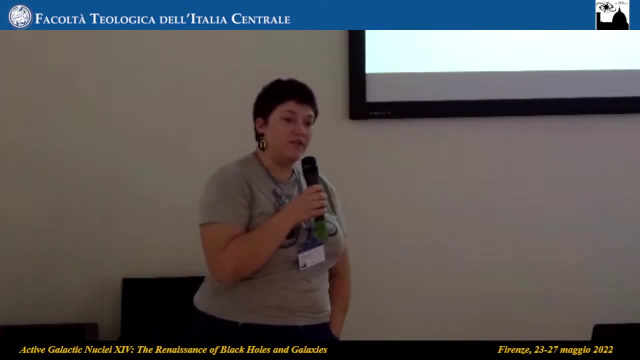 I am not Brooke Simmons. She unfortunately couldn't make it. Unfortunately, last minute changes happened, so you're stuck with me instead. I'm one of her PhD students at Lancaster University in the UK and I'll be using my time today to tell you about results. 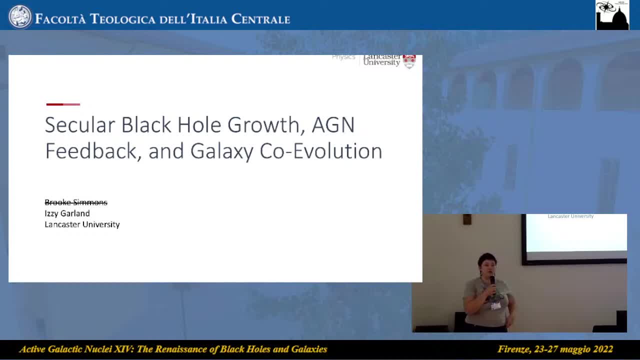 from our group and collaborators on supermassive black hole growth and galaxy co-evolution, specifically through the lens of secular processes, That is, processes that don't involve mergers. They occur in the absence of mergers. Is there a thing for me to flip? 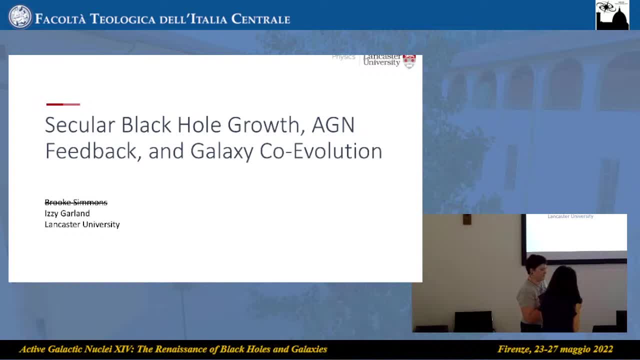 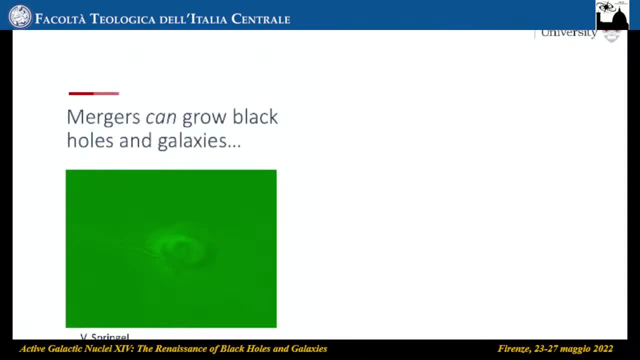 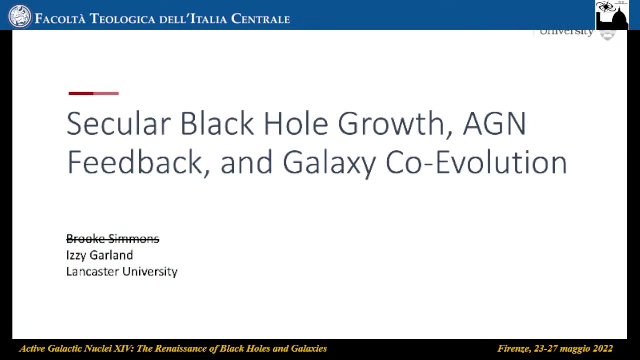 Cool, Thanks, Excellent, Sorry, Cool. So for a long time, discussion of merger growth dominated the field, and this was for several reasons, including selection effects and the fact that mergers can drive all these processes Like. it's very clear that mergers can and do. 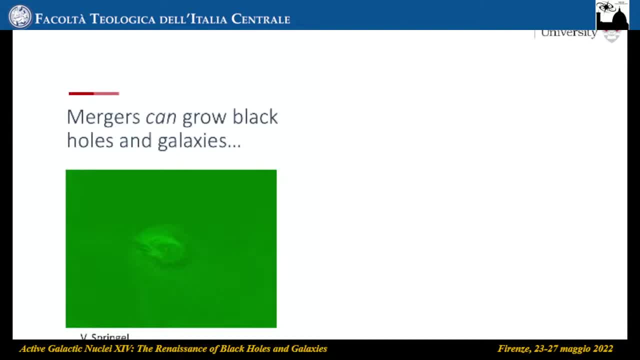 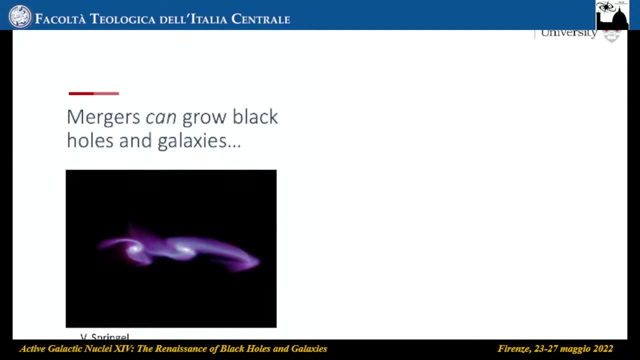 grow supermassive black holes and galaxies, and this is for several reasons. oh cool, the GIF sorted itself out. This is for several reasons, including the rearranging of angular momentum, you know, messing everything up, causing stars to grow, causing black holes to form. 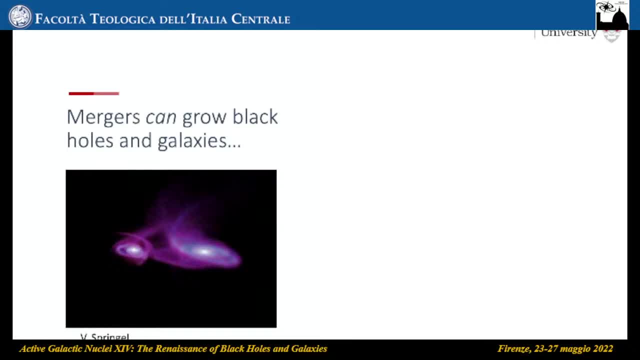 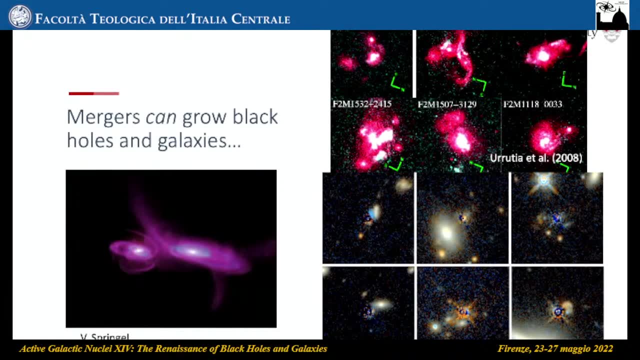 But it turns out that mergers might not be the dominant mechanism. But here we've got a couple of samples. There have been so many studies dedicated to merger-driven growth I can't possibly do them all justice with the time that I have. 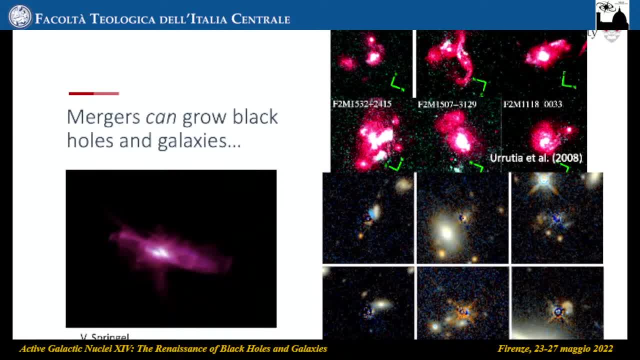 So here's just a couple of examples that use HST data and find that red, superluminous, red, radio-loud- sorry- quasars- a subset of AGN- lie overwhelmingly in merger-dominated environments. So, like I say, it's clear that mergers can and do. 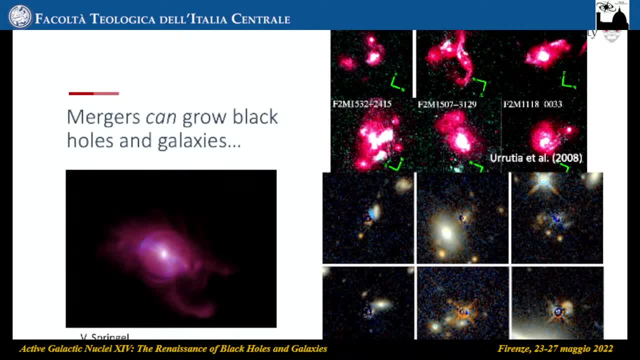 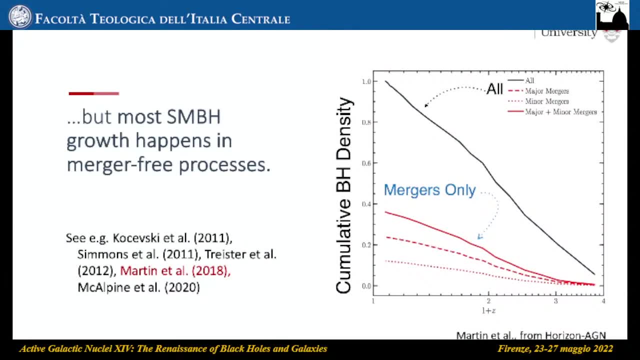 grow these galaxies and these black holes, but it turns out they might not be the dominant process. Actually, we're pretty sure at this point they're not the dominant pathway. So I'm showing a study here from a recent simulation by Martin et al. 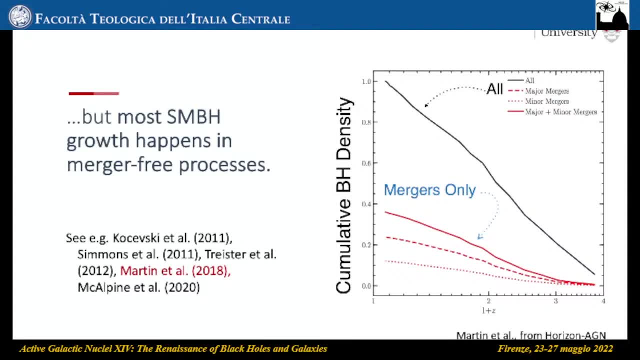 from the Horizon AGN team And it's showing that the cumulative black hole growth since redshift- about three up to the present day. only about 35% of this is due to merger-driven growth And studies such as McColpine et al more recently. 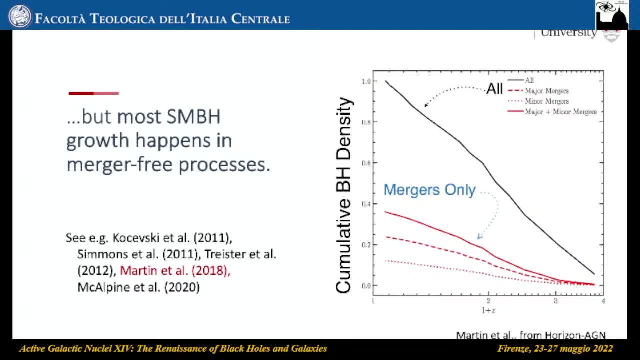 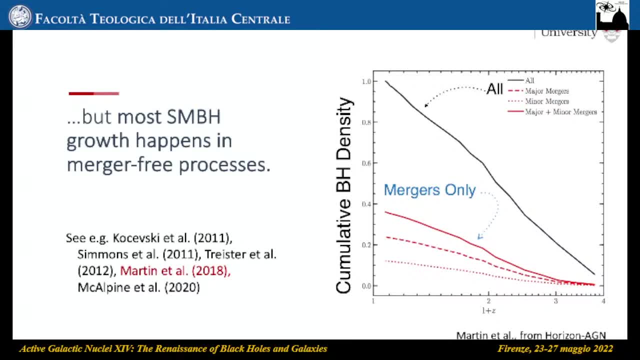 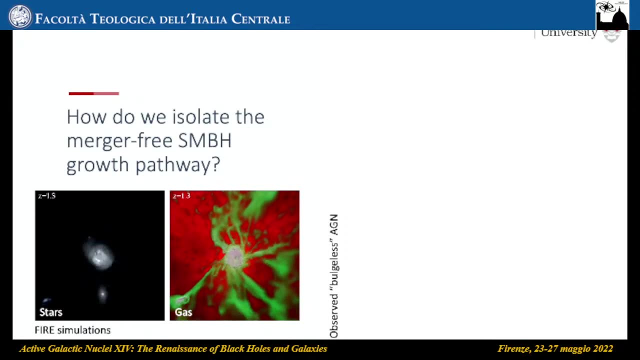 So it's crucial that we understand black hole growth in the absence of major mergers, because it clearly dominates the population. So the problem is isolating this merger-free pathway, And another thing that simulations have shown over the last few years is that a classical bulge, as we know, in a galaxy. 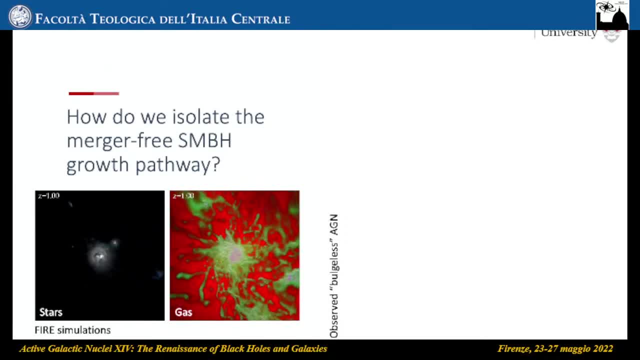 is an inevitable consequence of a large merger, a significant merger, And in the absence of such a merger, galaxies tend to evolve into bulge-less disk galaxies, such as here in the fire simulations. so if we see a galaxy, if we just observe a galaxy, and it's 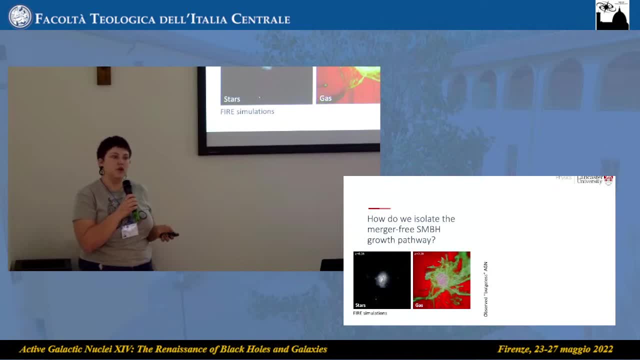 very strongly disk dominated. there's not much or there's no presence of a bulge there. we can assume that it hasn't experienced a significant merger since Redshift 2.. It's just grown via gas accretion and through micro-mergers. 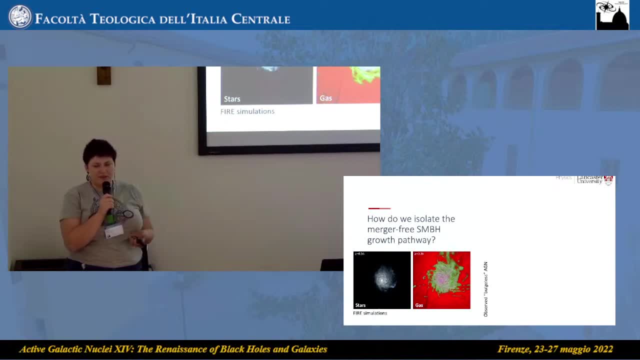 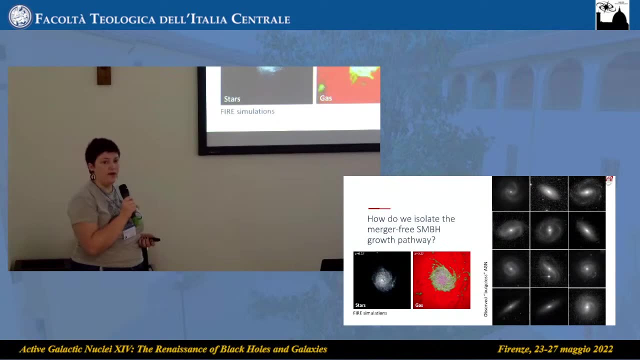 what we might call- which aren't really significant enough to disturb the disk shape. so we can isolate this merger-free black hole growth pathway by selecting exclusively disk dominated, bulge-less galaxies, and then, to get the black hole growth, we select a subsample of those that have AGN. 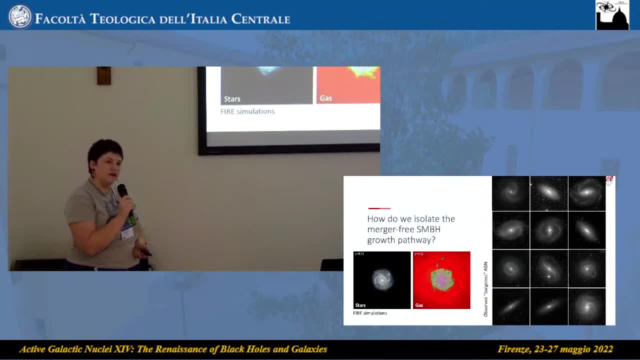 so the sample I'm showing here is a selection of our sample which is observed with Hubble. These are all disk dominated AGN. our whole sample is about 100, but if I put them all on there you wouldn't be able to see any of them. 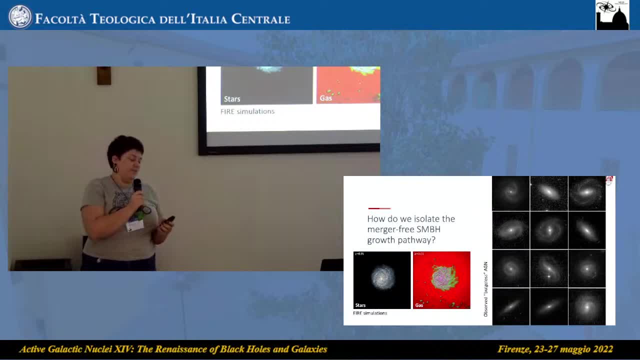 um, and these are all luminous AGN. in fact they're so luminous that they're quasar-like luminosities at the Redshifts they have observed, which is relatively local. we also have SDSS fiber spectra or Lick-Longslett spectra. 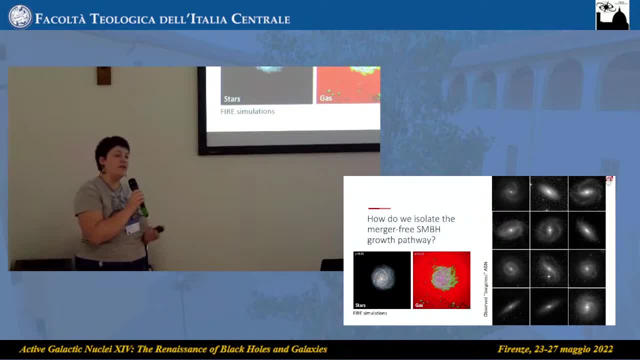 of each of these galaxies. for a couple we even have IFU data and for a small handful we have archival data at wavelengths from sort of x-ray to infrared. so, like I said, they're all luminous and they're all unobscured. AGN. 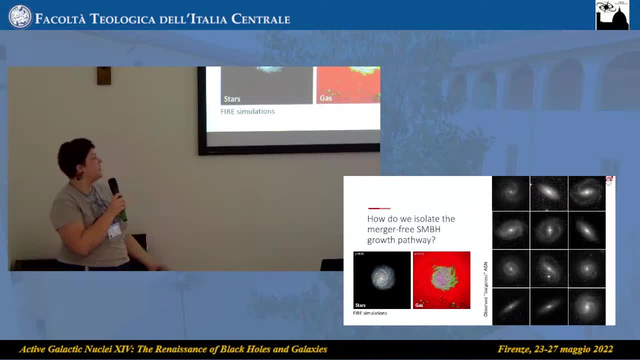 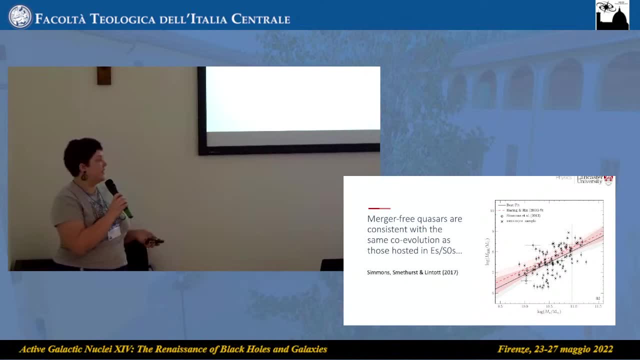 which means that we can estimate their black hole masses. so the first thing we looked at was: are these galaxies co-evolving? and we took their black hole masses that we estimated from single epic broad lines and we plotted this against their total stellar mass and you can see in the black 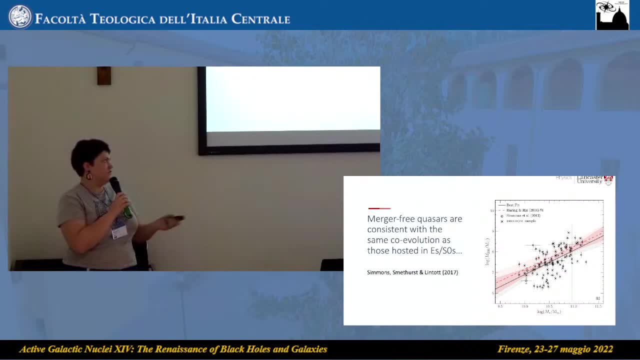 solid line and the shaded region, the black shaded regions, gray shaded regions, which are the best fit line, and the three sigma uncertainties that there is evidence for coevolution. and not only is there evidence for coevolution, there is also, if you look at the red dash line, which is the same plot but for um agn, hosted in merger driven galaxies such 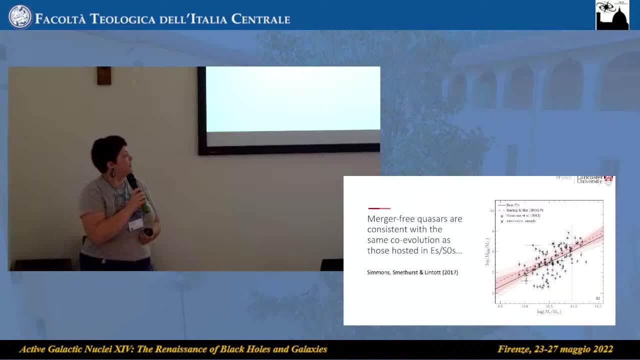 as ellipticals and s noughts, and statistically, these two lines are indistinguishable, um, and their slight difference in their normalization can be accounted for by the different methods that we use to obtain the black hole masses. so, um yeah, they co-evolve and they co-evolve in such a 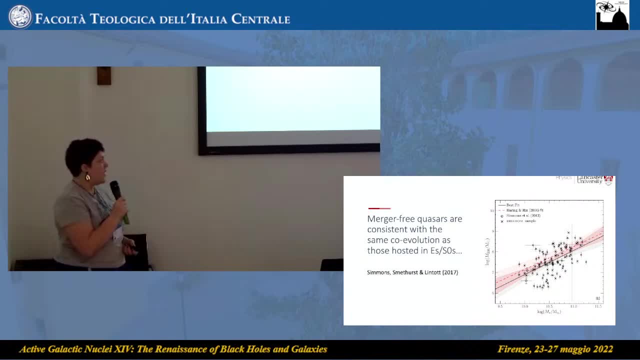 similar way to merger driven processes. but i should note, this is just one study, and not only is it just one study, it's a study that was selected specifically for very luminous agn, which means you're going to then involve things like selection bias and other studies doing this. 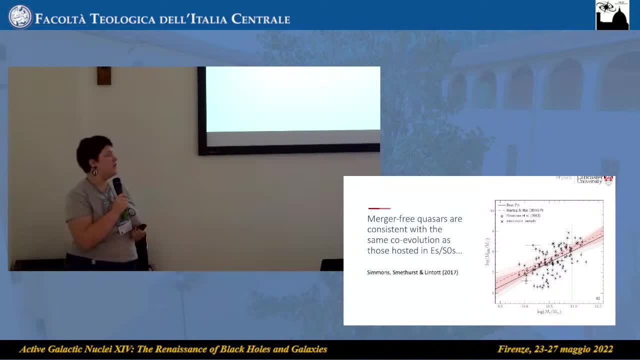 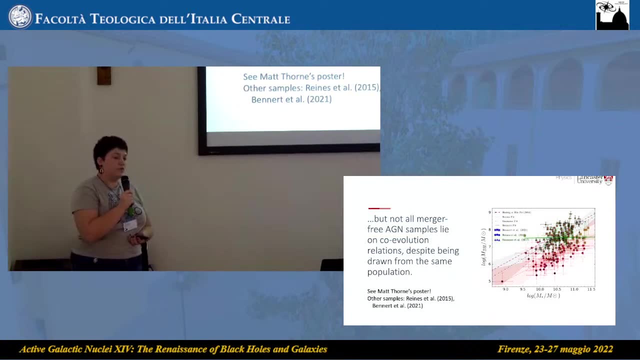 sort of work, selecting for different priorities, find different results. so here's the same plot, but an extra two studies overlaid on top and you can suddenly see that the overall picture is not that clear. and my colleague, Matt Thorne, who is also a PhD student at Lancaster and is here today, 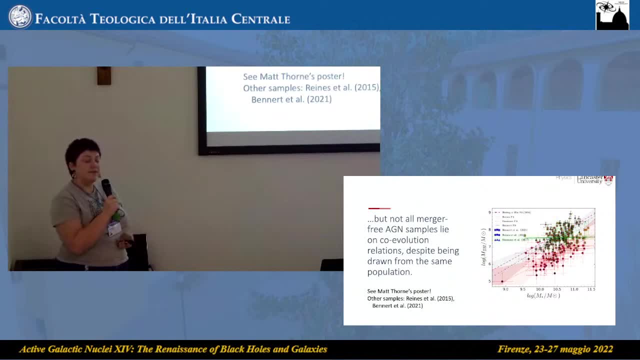 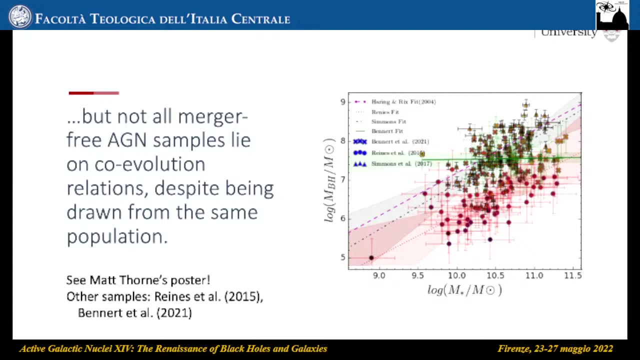 is working to reconcile these apparent differences in the results obtained by different studies and he's shown, through careful comparison of simulations and observations, and particularly folding in selection functions, that actually all of these samples are consistent with being drawn from the same underlying sample of supermassive black holes. Now Matt's writing up his results at: 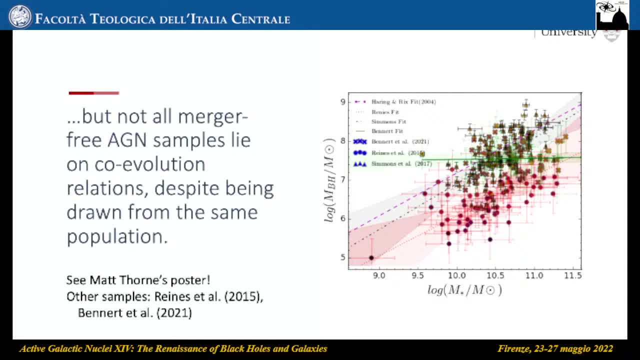 the moment, but you can get a sneak peek by checking out his poster, which is available upstairs. but this is just a really good reminder that selection effects are so important and we really need to consider them in the work that we do, and it's also a nice confirmation that our sample of merger-free 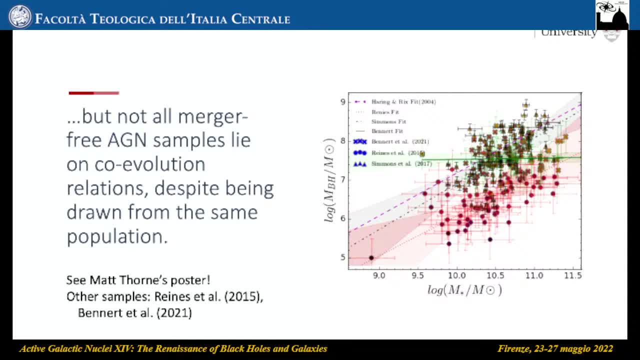 AGN are, in fact, consistent with being drawn from the overall underlying population. So we've got these galaxies. we now know what. well, we now know what their black holes are doing and forming rapidly. but if the black holes are forming rapidly, what are the host galaxies doing? 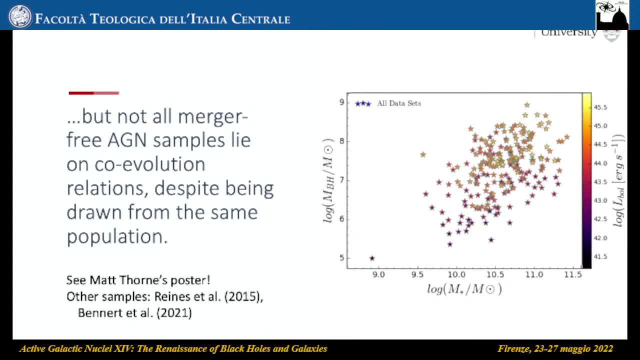 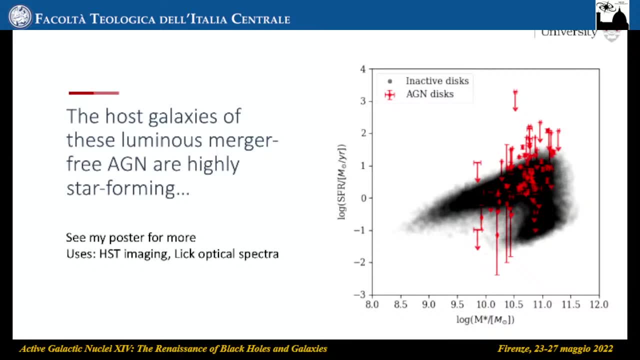 and this is what excuse me and this is what I'm working on. So, as part of my PhD, I'm looking at how the star formation rate changes in these AGN galaxies, which has proven a challenge, given that the AGN are making every attempt to contaminate our measurements of star formation. 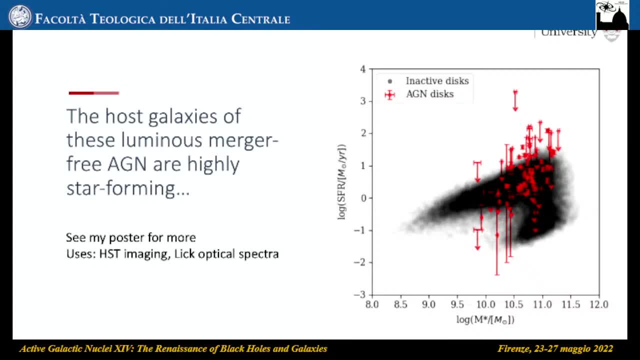 but after removing these so-called contaminants- obviously they're not contaminants, but they feel like it some days- we can see that the star formation rate of galaxies hosting AGN takes up the same sort of range as galaxy disk galaxies that don't host an AGN, as you can see from this, 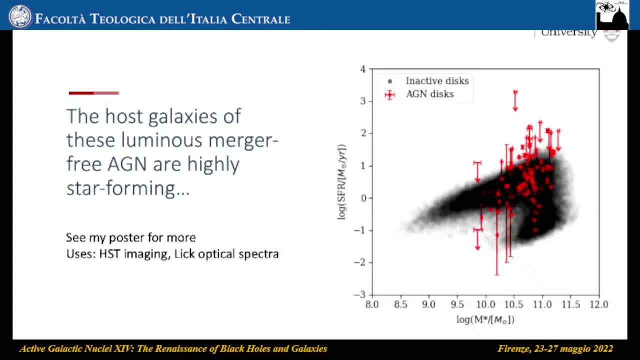 plot I've got up here. However, the average star formation rate for the disk galaxies hosting AGN is slightly higher than the average star formation rate for the disk galaxies hosting AGN, Then for that of the inactive disk galaxies. So this is really, really interesting. they're kind of 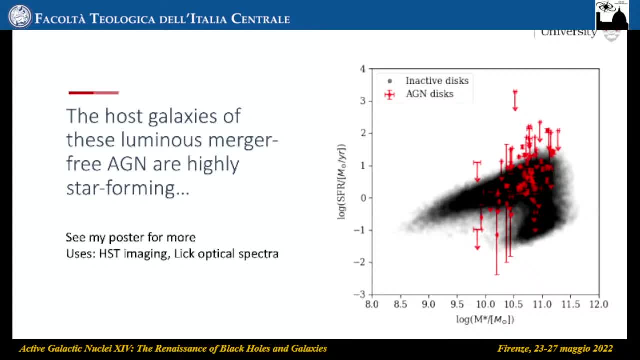 growing their black holes and their galaxies at the same time and it kind of sort of helps us sort out one side of the co-evolution relationship. Yeah, these black holes, these galaxies are growing together. So I also have a poster here so you can come and talk to me about that at some of the 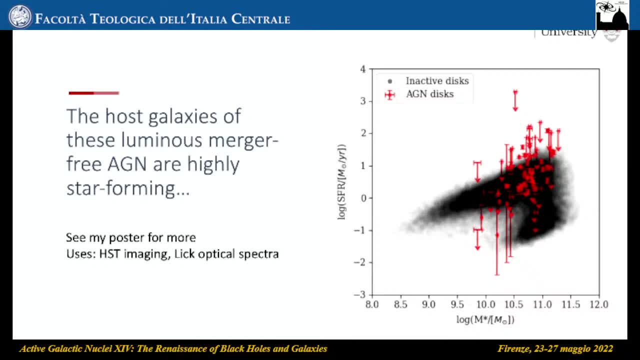 coffee or lunch breaks if you'd like to. This is just one of the interesting results I've found so far on the work I'm doing with these AGN disk galaxies. Now, another really interesting thing to note about our sample is similarly to a sample of AGN in. 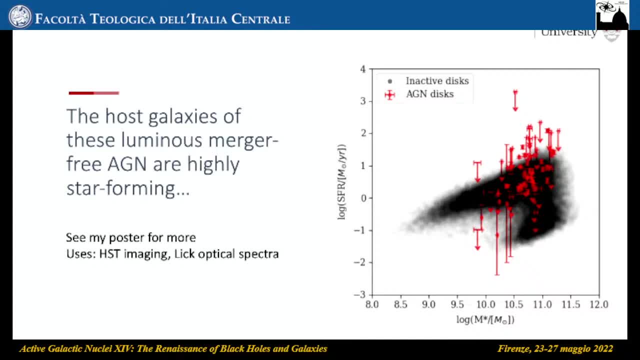 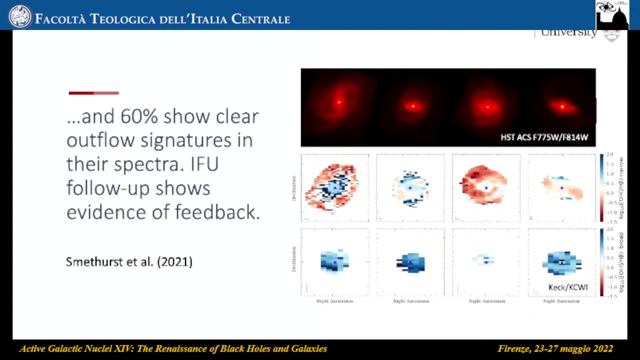 merger driven systems. about 60 percent of our AGN show significant evidence of outflows in their O3 components And we got Keck time to look at this. We used KCWI in a project led by Becky Smethurst, who is an RAS fellow at Oxford, And what you're seeing here is INI's. 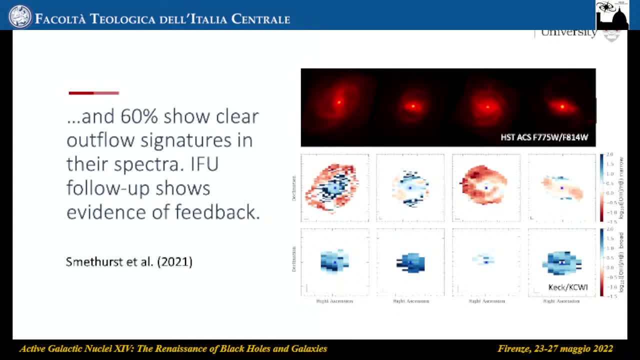 ionisation graphs or ionisation plots, specifically O3 over H beta. The red colouring is indicative of regions with high star formation and the blue colouring is indicative of regions of such high line ratios that it's so likely that they're triggered by an AGN. And the thing to notice is: 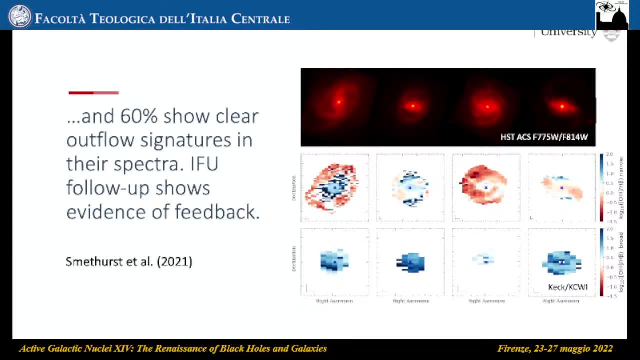 the extent of these, like the spatial extent of these outflows. Sorry, it's the top button, the little laser button. Sorry, how much? Yep. Thank you, Yes, Cool. So yeah, you can see the significant extent of these outflows here. 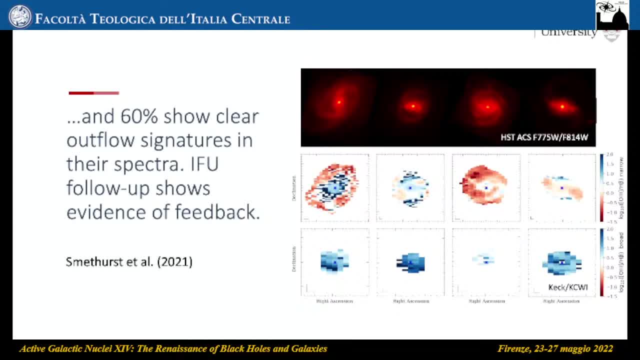 What you can also notice- or you can't notice- from these graphs, but I can tell you- is that the power in these outflows is very typical to the same sort of power you would get in AGN hosted in merger driven samples. So this indicates that they should. they're typically the same And this is not what. 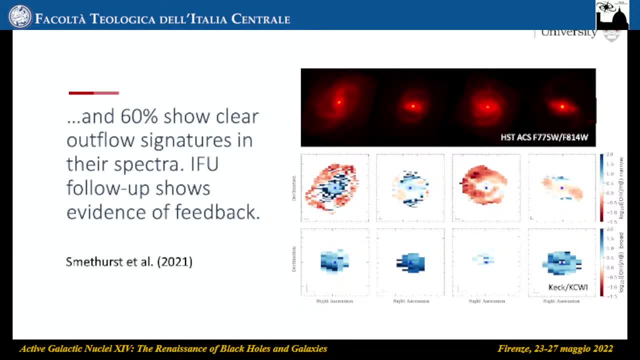 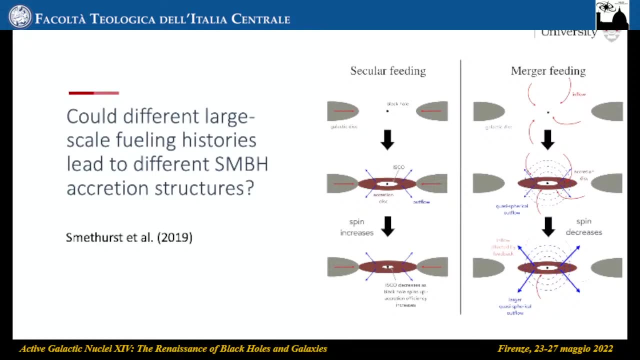 we were expecting at all. There's actually several reasons to think that accretion through merger driven systems would be very different to that in secular systems. So we know this from a 2019 study also run by Becky, where we used narrow band images of those same little sources you saw before and we analyse their outflows And it turns. 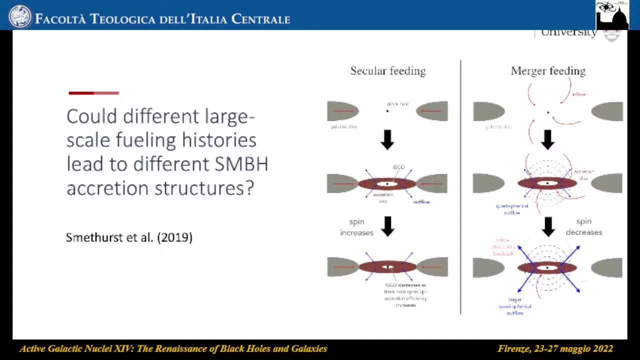 out that they were different to a carefully selected control sample of AGN in merger driven systems, And this is complicated by this toy model here. So on the left hand side we have secular feeding, so merger free processes, And the black hole is consistently fed from the disk. 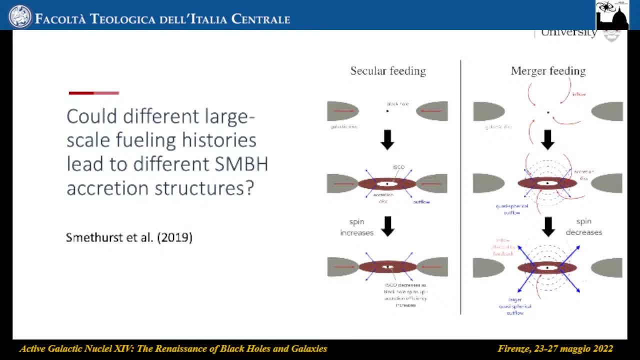 galaxy in very consistent matter, All in the same direction And over time, this leads to eventual spin up of the black hole. I have timed this really badly. This leads to eventual spin up of the black hole, increasing the overall accretion efficiency And, in the merger driven system, because it's being 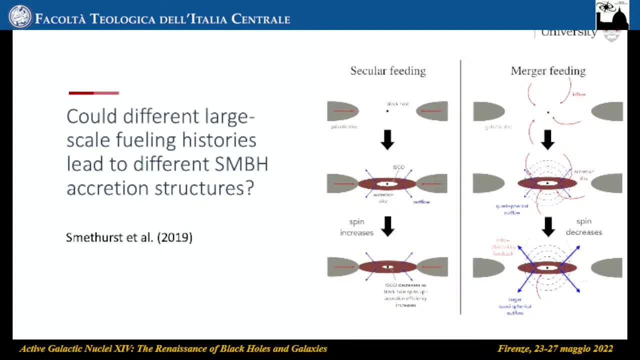 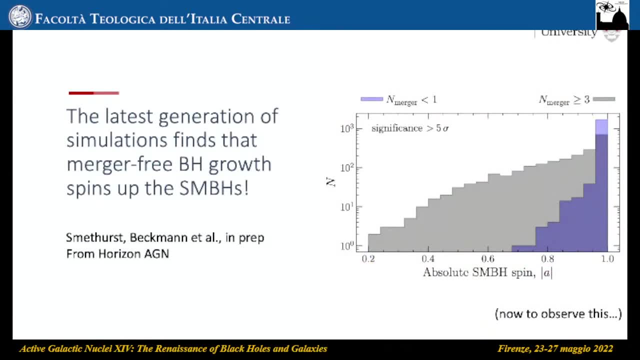 fed from all directions. this leads to the eventual spin down of the black hole, and we don't have data to observe this yet, but what we do have is cosmological simulations. so Becky is currently working with Ricardo Beckman, a JRF fellow at Cambridge, and they're looking at cosmological 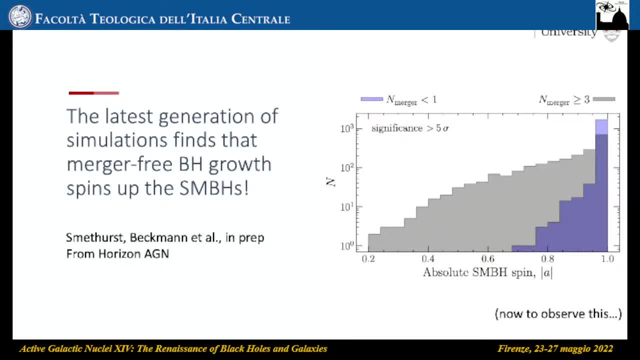 simulations and separating the samples by the number of mergers they've had in their system. so in the purple we've got merger free systems and in the gray we've got systems with several mergers. as you can see, their spins really are different. the toy model was pointing us in the 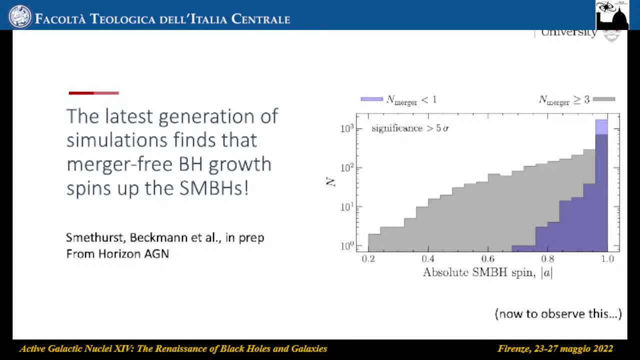 right direction. merger free systems have much greater spin up and the dream is to observe this directly, but given current facilities and the fact that we need a large sample, that's just not currently possible. but what we can do is look at other parameters in the supermassive black hole. 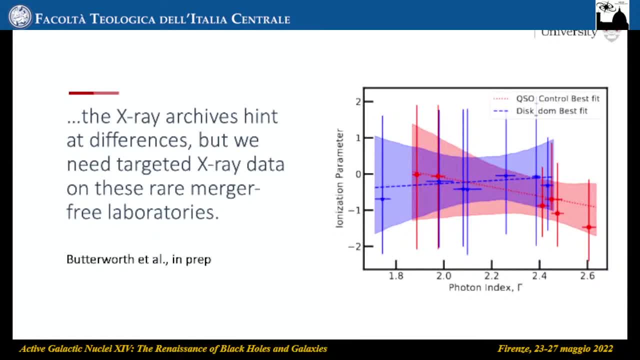 region that could be affected by this. so a master's student previously in our group, Josh Butterworth, who's now a PhD student at Leiden, looked into this. um um, you looked through the archive data and it turns out we had xmm data for a very small handful of. 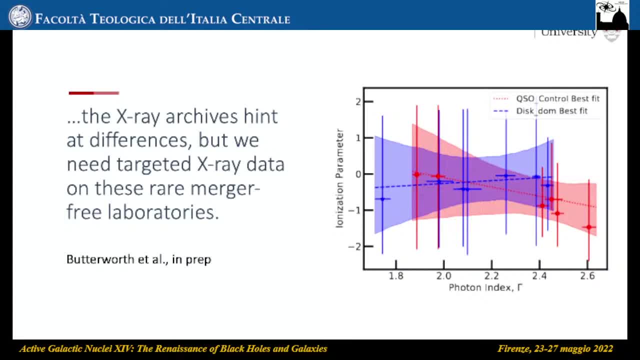 our sample, as well as for agn in a couple of our merger driven samples. so the photon index you can see is higher in the control sample and there's even they could have slightly different slopes when relation to the ionization parameter, but the sample is too small to say with any sort of 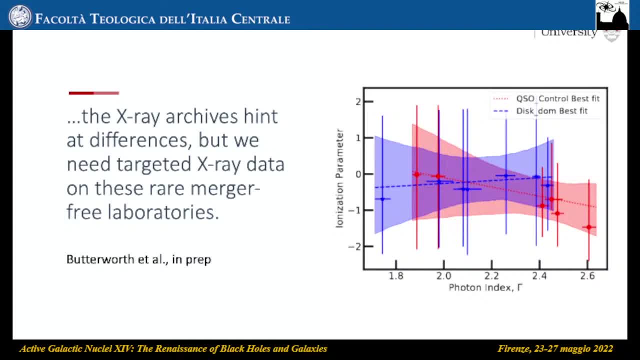 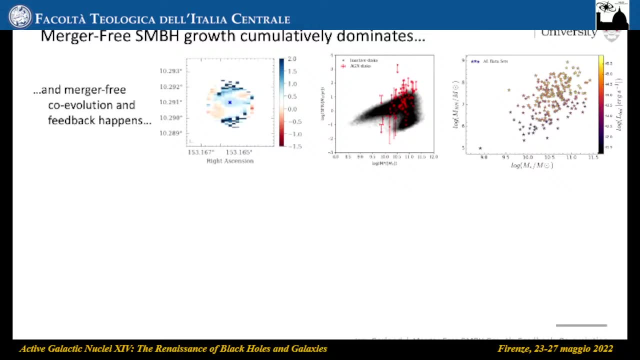 significance that they are actually different. so we've sent- well, we're applying for xmm time this autumn to try and hurry this um to get better and more data. so just to sum up, if there is one thing that you take away from this talk today, it's that merger free, supermassive black hole growth is the primary mechanism through. 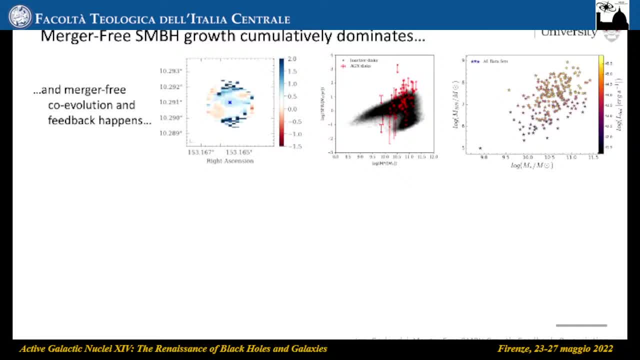 which black holes are grown in our universe, and this mostly happens in a way that's very typical to that in merger driven systems. however, there are some slight differences that persist right down to the tiny scales of the supermassive black hole. um so, watch this space. hopefully we will have 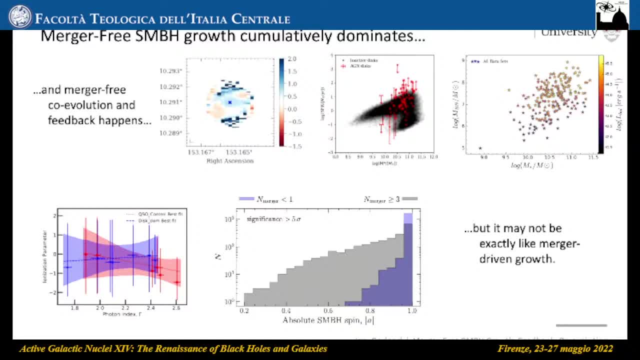 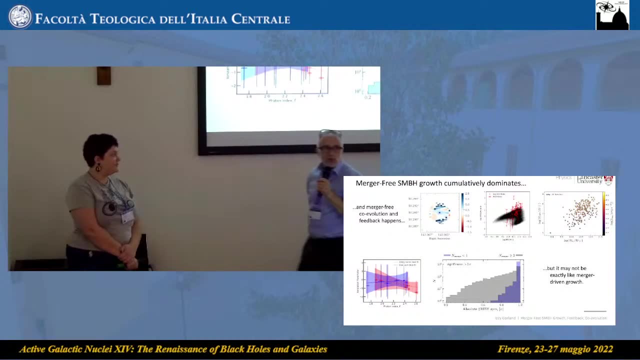 some more data soon and we can really complete this picture of merger free growth. um. the future holds so much. i'm so, so excited to see where this takes us um. thank you very much for listening to me. thanks, some questions for itzim hi. thank you, very nice talk. i was wondering um is it possible that some of your bulgeless agn are? 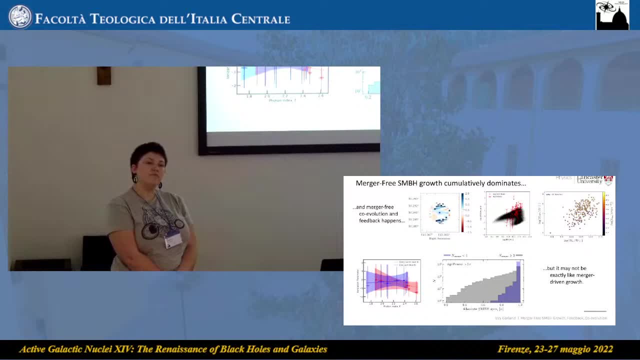 actually misclassified because the agn is dominating the central emission outshining the bulge. yes, so we use not only galaxy zoo to kind of get an initial idea of where the bulgeless sample came from, but they were then looked over by a single classifier because there's only a hundred in there. 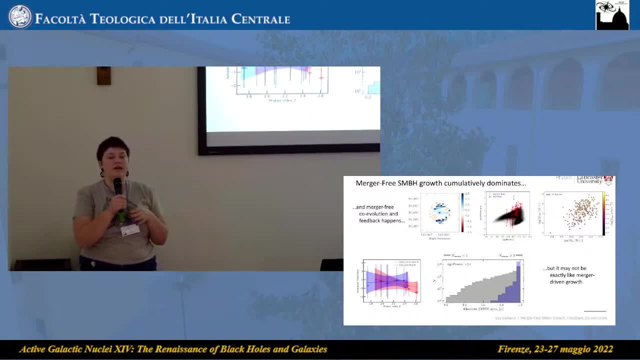 so they've all been individually looked at by um sort of one single expert classifier. um and any that we were like, we're not really sure if they're bulgeless or the agn that's a bulge or the agn is there. um, we kicked out so that our sample is very, very pure but might not contain. 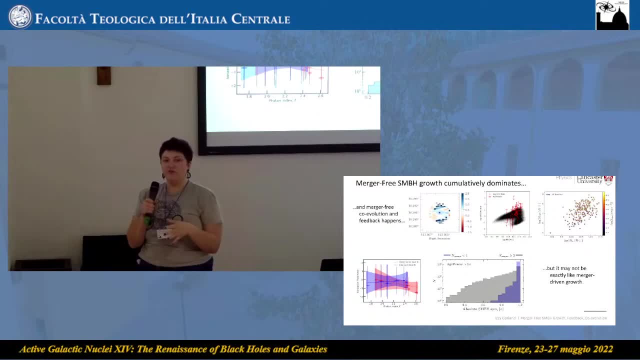 all of the bulgeless agn that we could have potentially done. we went for purity rather than completion. thank you. last questions for itzim hi. do you think um the the importance of merger driven uh triggering would increase the tire ratio, say ratio two, three, four. sorry, can you repeat the question i couldn't quite. you said: 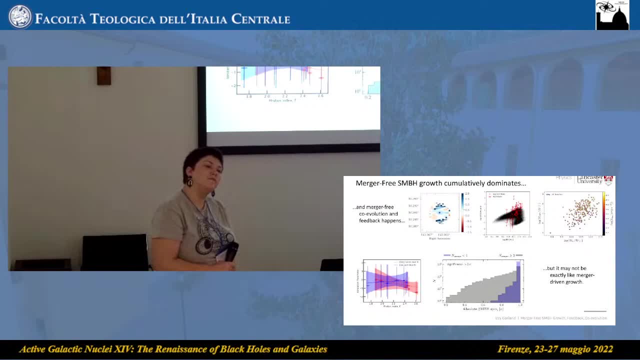 the merger free. supermassive, supermassive growth actually dominates the growth of the cause. you think this holds for all redshift? so obviously at the moment, because we need to understand the morphology so well, we need to understand the morphology so well. we need to understand the. 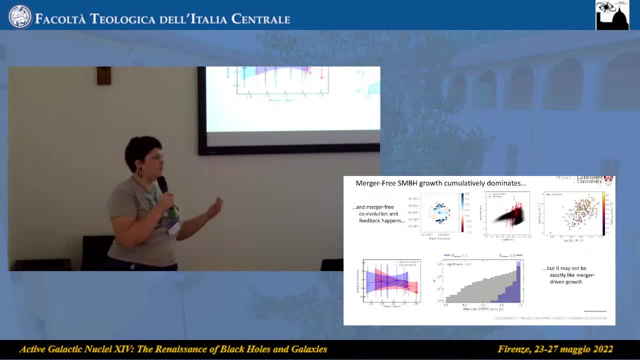 morphology. we're using high resolution stuff which is generally lower redshift um the beautiful hubble images we can get um. at the moment we can't really take it back observationally further because we currently don't have data that's clear enough on the morphology to truly understand it. 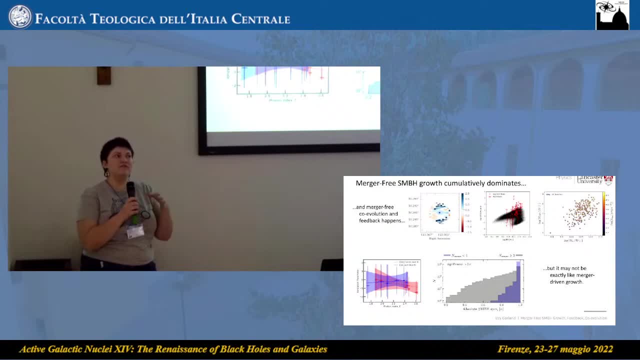 but i think simulations will help us sort of tease out the answer there. but i think we will heavily rely on simulations or jwst. i can say that now it's up, um, so hopefully i'm thinking about in a couple years time applying for jwst time to get a deeper look at some of these galaxies. 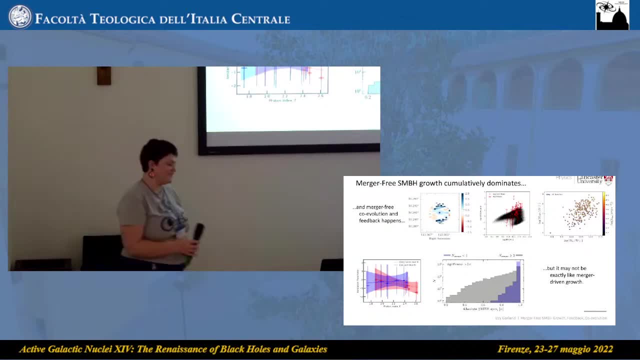 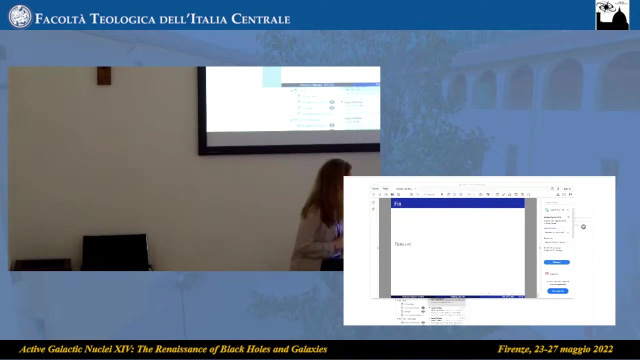 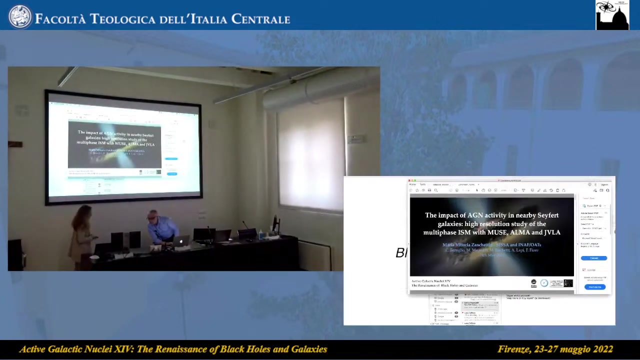 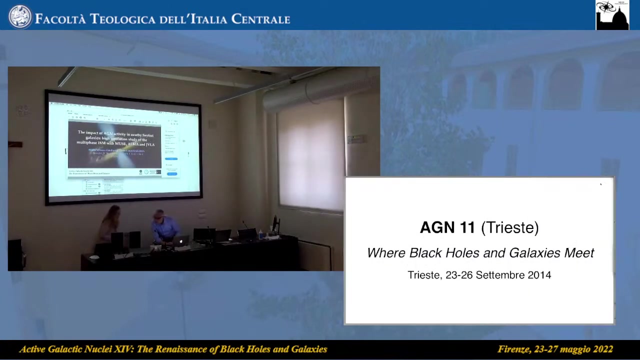 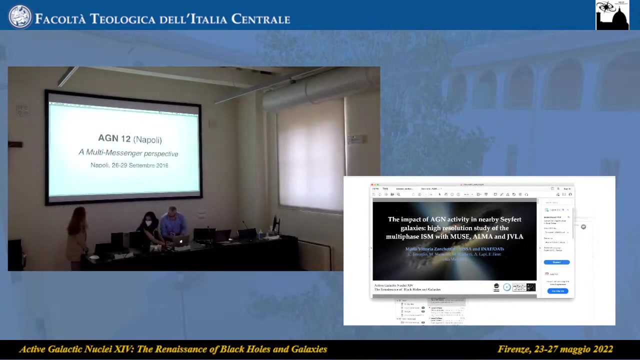 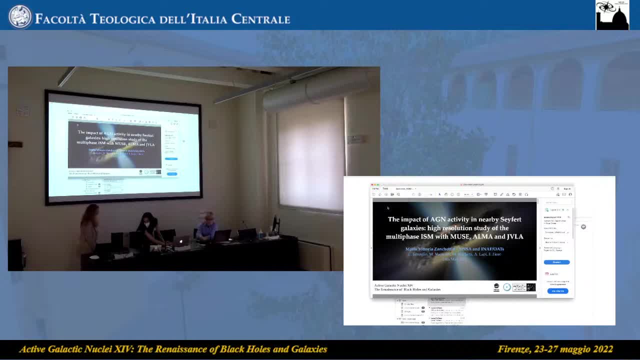 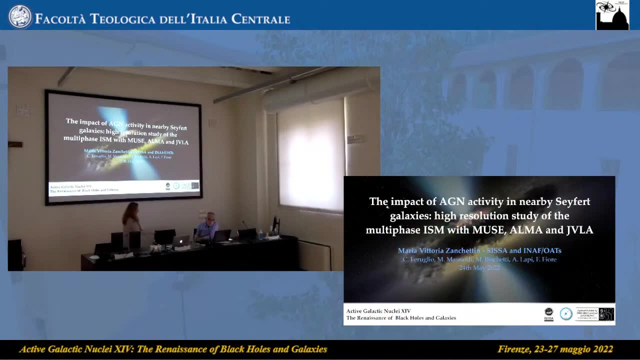 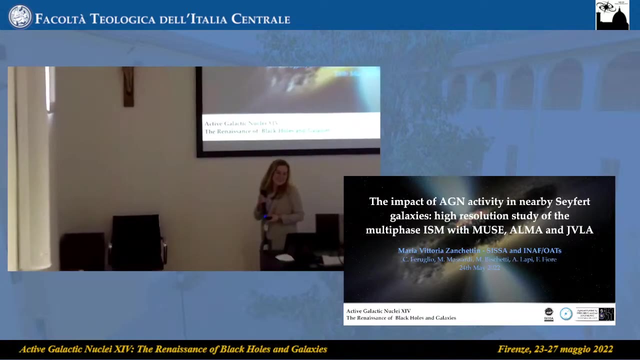 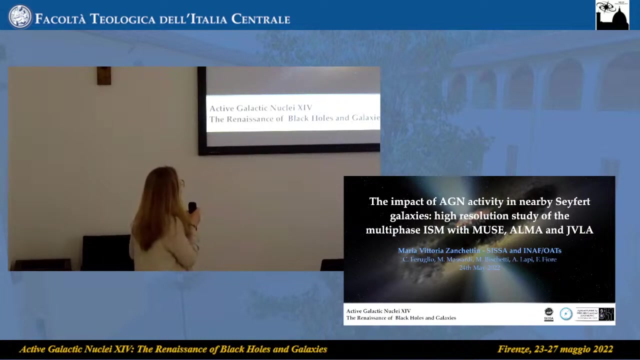 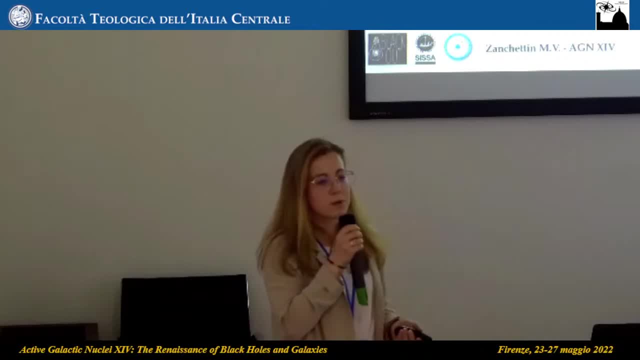 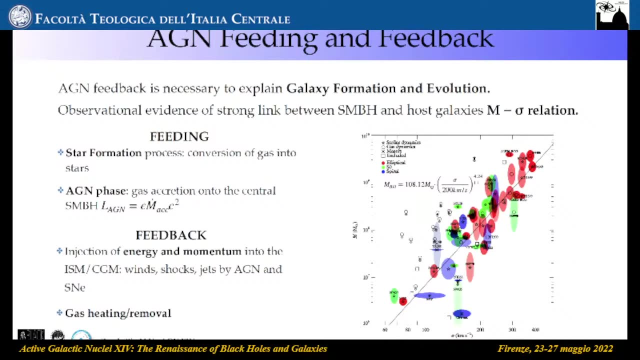 strong observational evidence of a strong link between a supermassive black hole and host galaxy and their host galaxy. just to show, there is the well-known the m sigma relation. we have the. it points to our feedback. we have the feeding- feeding phase that involve the agn phase and 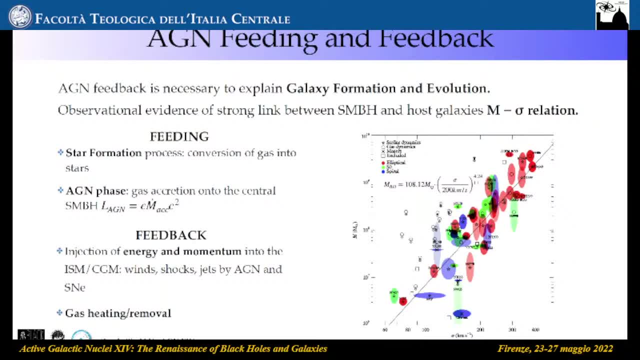 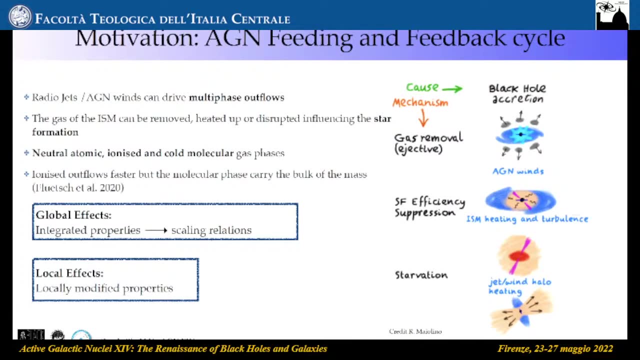 then star formation. that the feedback and it implies the injection of energy and momentum into the interstellar medium circle, galactic medium or the gas heating or removal, in this context, the edge. there are different way of feedback. we can have radio jets or agent driven winds that can drive a multi-phase outflows that involve a different gas phase, like the neutral. 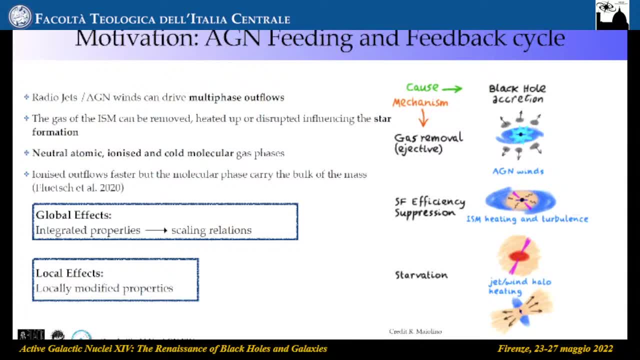 ionizer and called molecular one. then the gas in the interstellar medium can be removed, heated up over, distributing um, influencing the star formation profit process itself. and there is some hint about that, the fact that the united outflow are the faster and but the molecular phase is the one that carry the bulk of the mass. to study the feedback we can 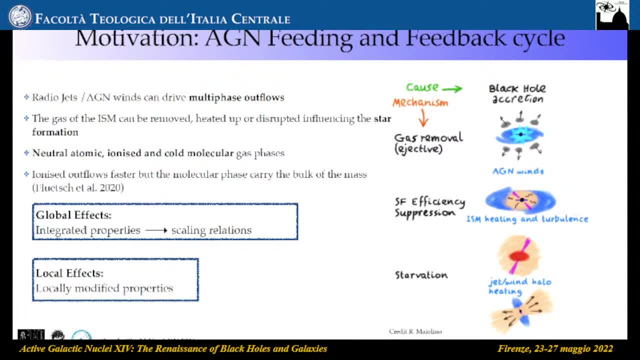 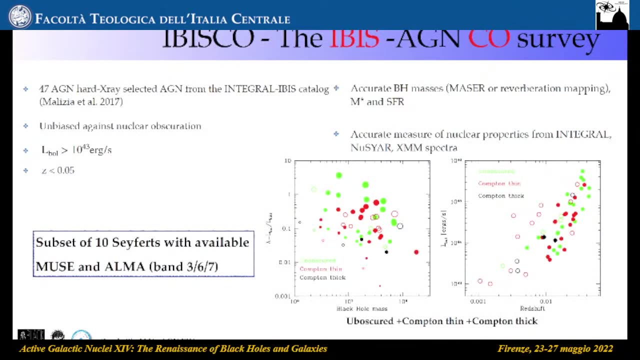 have a different approach we can to. we can look to global effects- so integrated properties- and study the scaling relation, or study local effects, so locally modified properties. to do so, we selected the ibis agn we perform. we took the ibis agentio survey that involved 47 agenda arctic sprayer, selected from the integral ibis agn catalog. 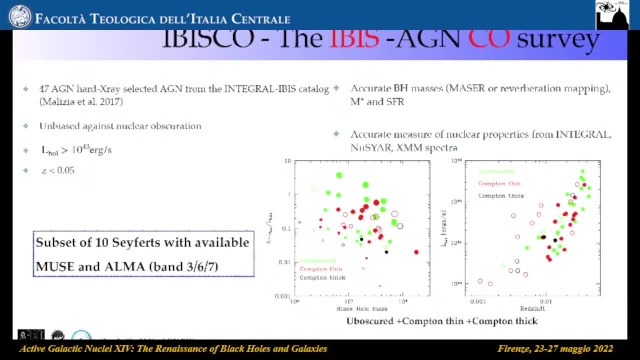 in order to not to be biased against nuclear obscuration. this sample, as a volumetric luminosity above 10 to the 43 arc per second, are local agn and the accurate measure of the black hole masses is some master star formation rate. of this sample, we selected the um for my phd thesis: a subset of the sea of 10 seaford. 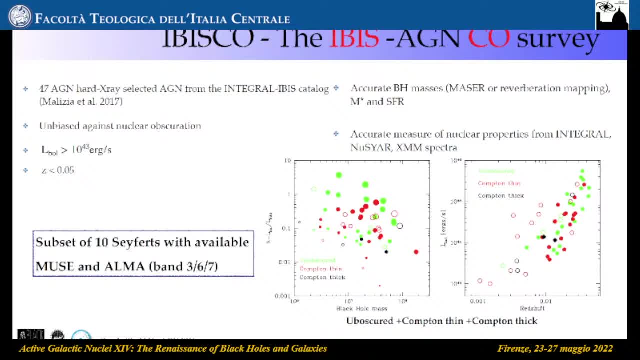 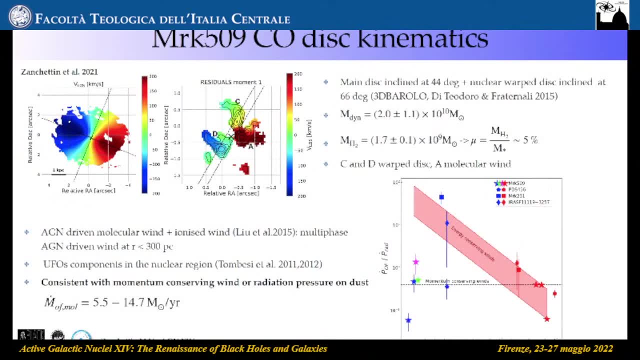 with a variable muse and alma data in order to perform a multi-phase approach. first of all, in this presentation we show you the results on two main two seaford. the first one is the marcarium 509 and this in the in the our work. in my work i studied the mainly the 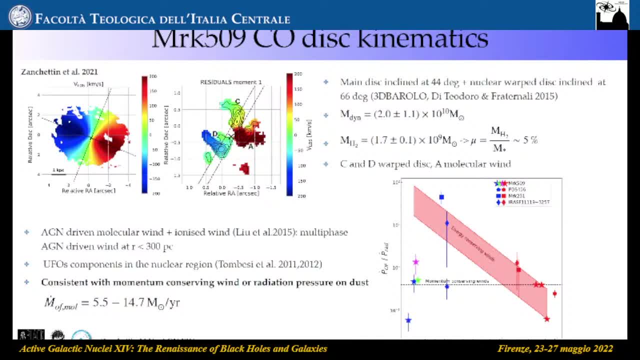 co221 data from alma. as you can see, the the alma velocity map, the the alma data, can be modeled with a main disk inclined at 44 degrees. we use the 3d barolo software by the tutorial fraternali. subtracting this, the main disk, to the alma data we we found that the inner region can be modeled with: 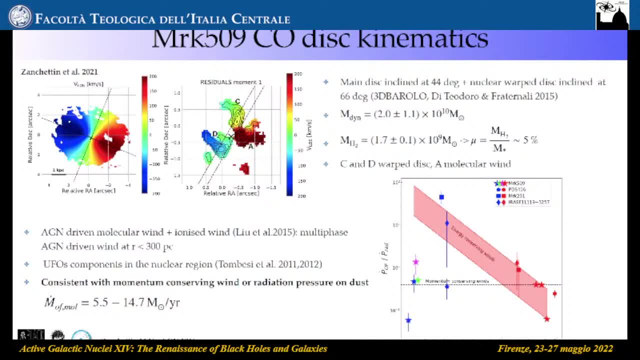 a nuclear warped disc inclined with respect to the main one and moreover, we find that perturbation to the disc, like kinematics here report- is with a a level that is consistent with age and driven winds in the molecular phase. from literature we know that this. it is been reported that 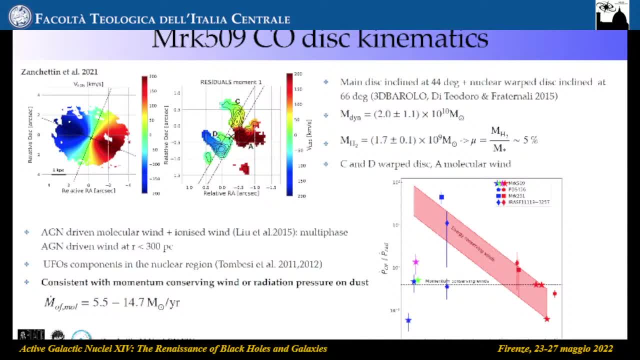 these galaxies show also ionized wind, wind and the several ufos component. putting all together, we can. we can assess the fact that this multi-phase outflow is consistent with momentum conserved, with the momentum conserving wind or radiation, pressure or dust, as you can see here from from: 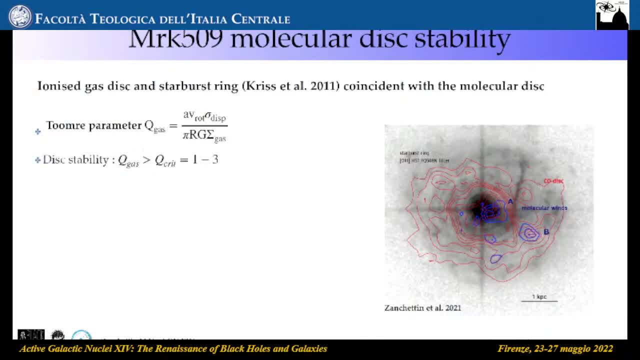 the plot. and we also found that the molecular disc is coincident here in red contours with a nice gas disc and with the star bustering that you can see in the in the map from hsc. and we will, uh, we want to assess the stability of this disk. to do so, we computed the tumor parameter. 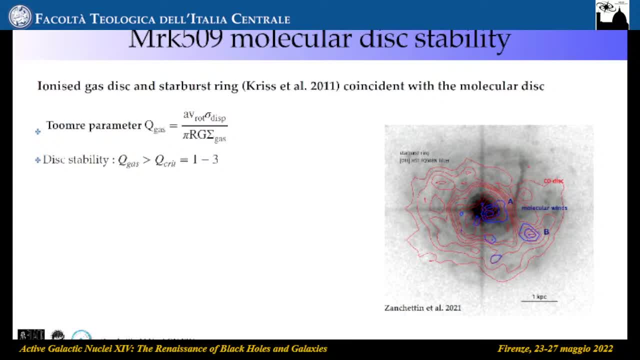 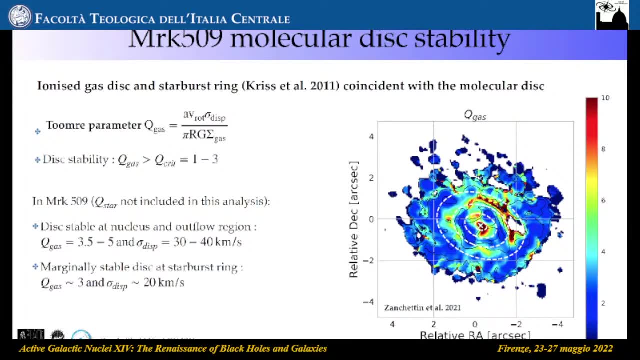 this parameter. if it is above a critical value. that for the gas phase is between 1 and 3, the disc is stable for this galaxy. we found that the disc is stable at the nucleus and in the outflow region. we found values between 345 and 5 and the velocity dispersion between 30 and 40 kilometers per second. 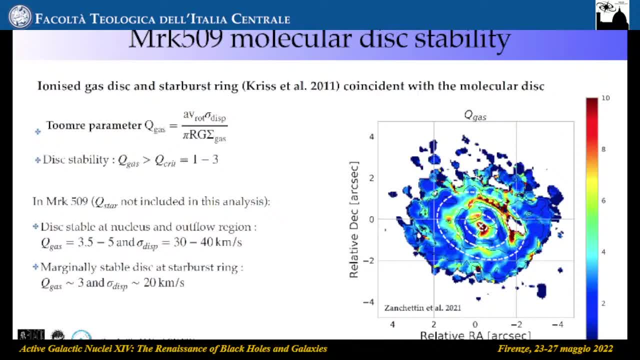 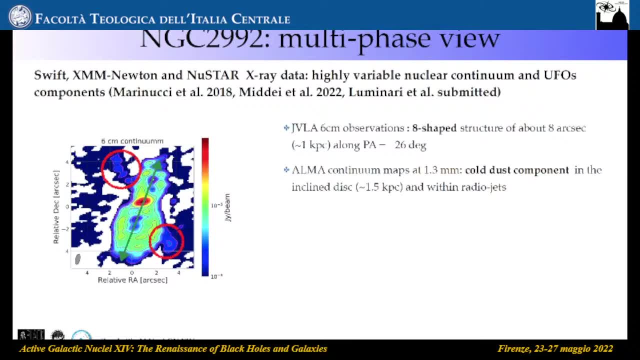 marginally stable at the start bus ring with values report in this slide. Then we analyzed also the local CFR Guaranty, NGC 2992.. In this case it is an object well studied in X-ray And from X-ray analysis it is reported a variable nuclear continuum in the UFO's component. 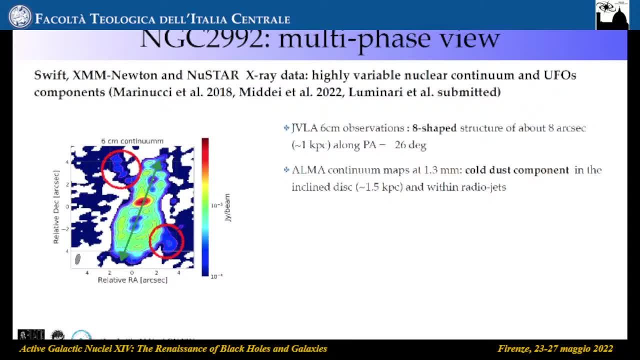 In my work. I instead analyzed a different set of data. First of all, the GVLA emission at the six centimeters that you can see here. This is the. the map show the radio shape structure of about one kiloparsec a nuclear radio jet. Then the point is that the emission 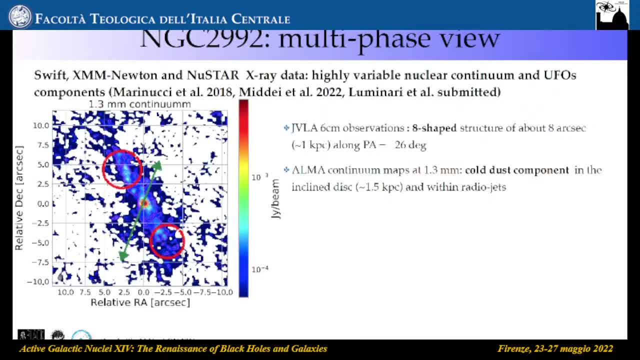 in the red circle is well aligned with the ALMA continuum, ALMA continuum and the radio jet, In this case the ALMA continuum map. at 1.3 millimeter the trace they call dust component in the, in the, in the inclined disk, And also there are hint of emission. 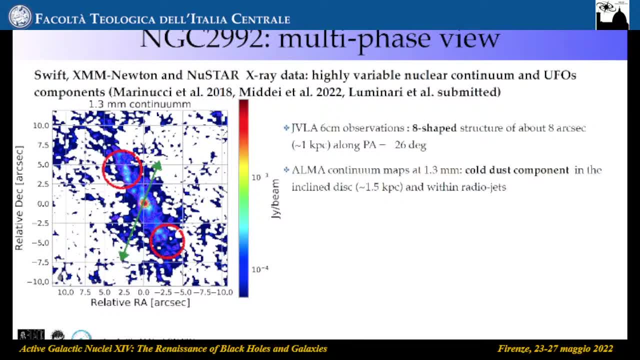 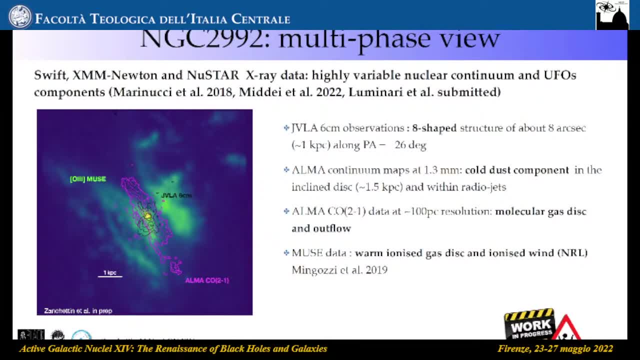 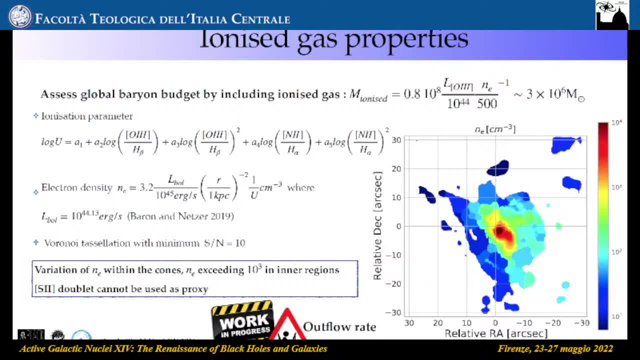 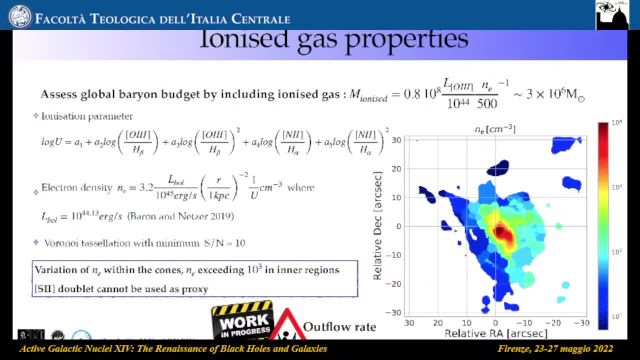 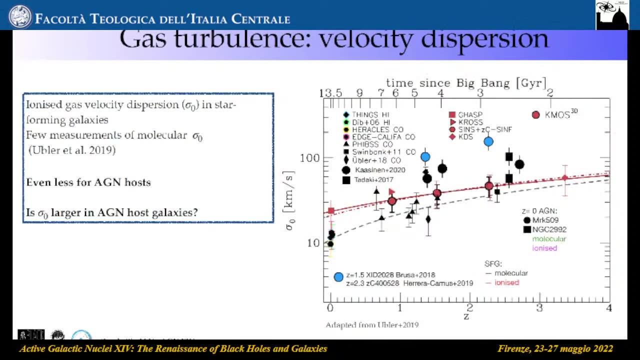 And this is why we cannot use the SU-W2 as a proxy of the electron density, And this work is still ongoing. We have to derive the outflow rate both for the molecular and for the ionized gas phase. Okay, And to put this in a weather contest, 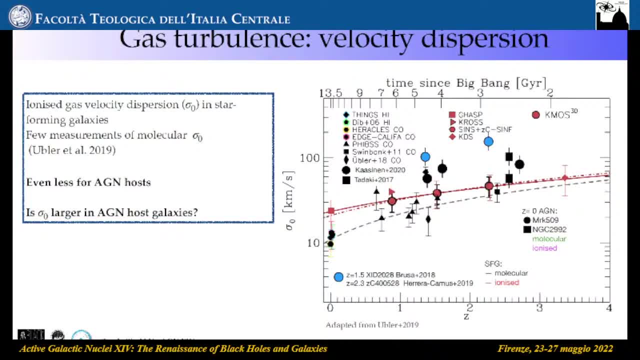 I reported here the plot from Hubler et al 2019.. When you can see the velocity dispersion as a function of the redshift for a sun-forming galaxy: In red the value for the ionized gas And in black the value for the molecular gas phase. 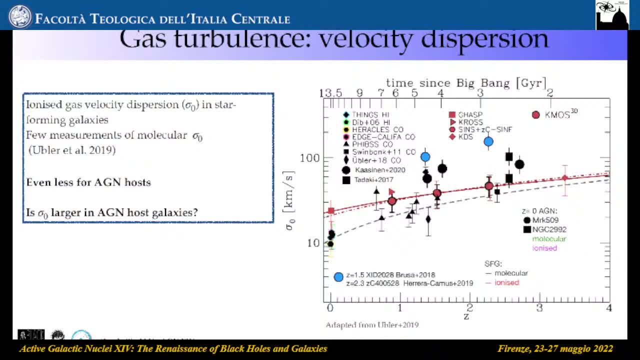 As you can see, there are a few measurements for the molecular gas phases, And even less if you take into account the Aegean host. So we want to understand if this value is higher in Aegean host galaxies. Okay, So using our results that are only for two galaxies, of course. 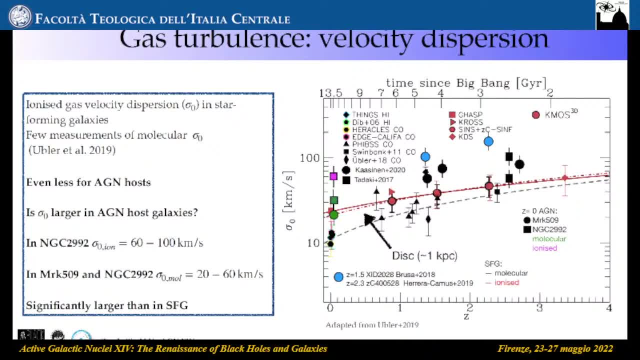 we found that both the molecular velocity dispersion the ionized gas dispersion are higher with respect to one in a sun-forming galaxy. Both in the disk- here the velocity dispersion is computed at 1 kiloparsec- And both at the nuclear region, when at an early 200 parsec is even worse. 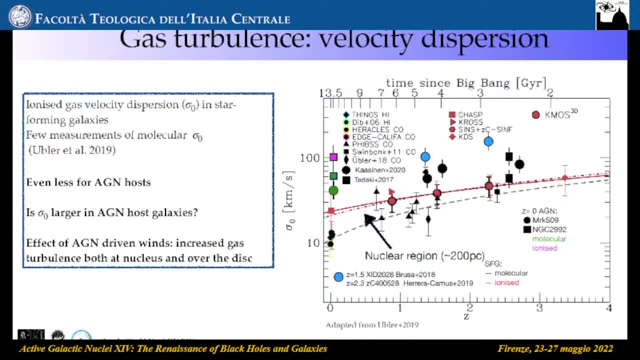 Okay, So this is a hint- that one of the facts of the Aegean-driven winds is to increase the gas turbulence both at the nucleus and over the disk. Of course, this is the results only for two objects. What you want to do is to assess this value for all our sample. 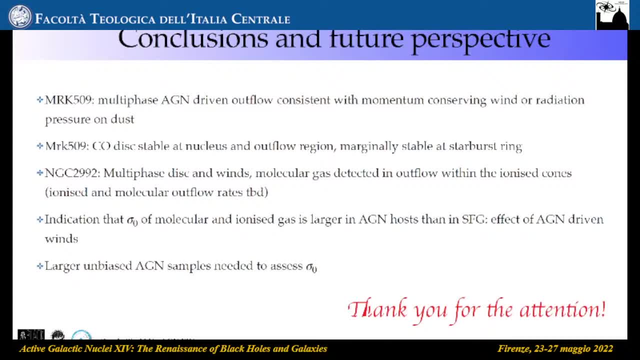 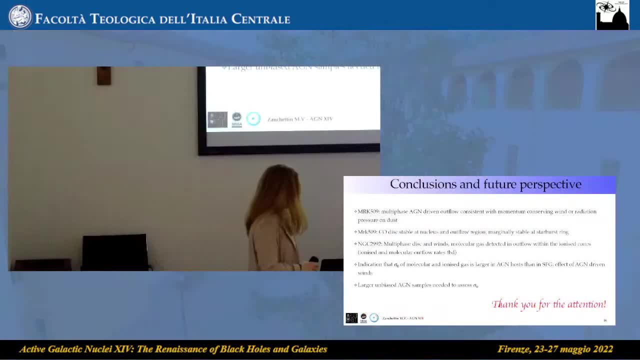 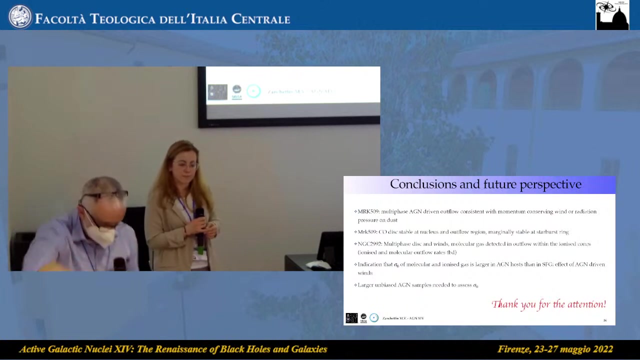 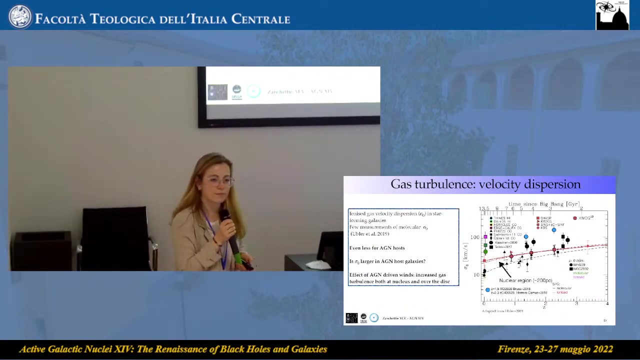 And so, to conclude, this is my conclusion And I thank you for the attention. Thank you, Okay. questions for Vittoria. Okay, This one, Yes, Okay, I really don't have a particular question, but it looked like a complicated plot to me. 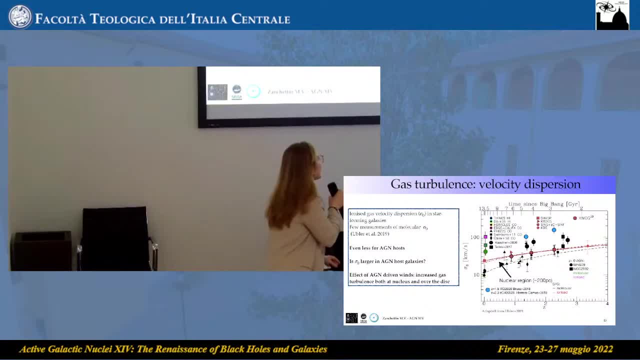 And I didn't really. Yeah, yeah, Okay, I mean, you said that there is a clear evidence that in Aegean- Okay, I don't see the evidence- The red and black points are for star-forming galaxies from Hubler et al 2019.. 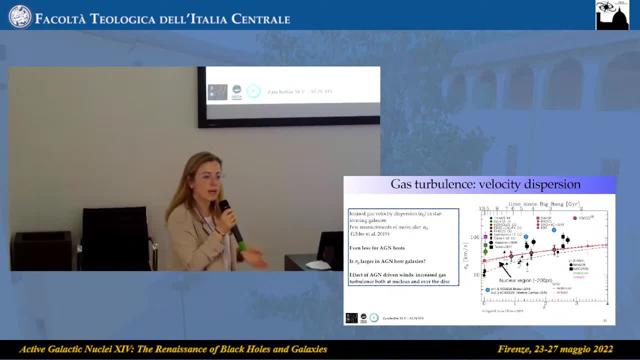 The red one are for ionized gas and the black one for the molecular gas. Then the blue points are for Aegean host at higher air shift at 1.5 and 2.3. And then the green points and the magenta points are from my work on CIFAR galaxy in the local universe. 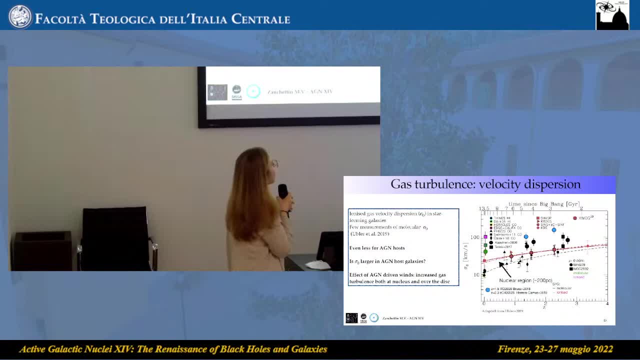 So, as you can see, the green points and the magenta points are above the relation found for star-forming galaxies. But how many sources do you plan to investigate in this way to have a statistical? Okay, Just to start, the whole subset we found. 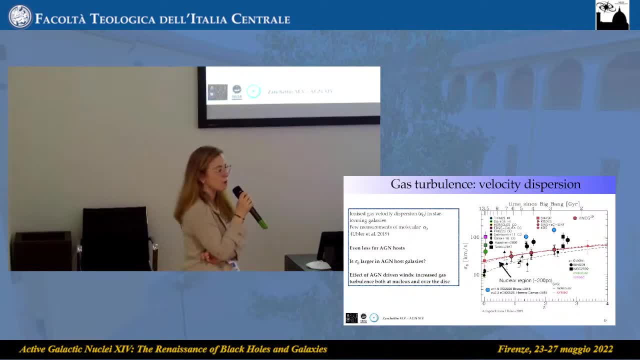 Because the problem, The problem, The problem. We want a multiphase approach, So we want to have objects with both ALMA at high-resolution observation and NEWS, And that's the point. So we will start with these 10 galaxies and then we will see what we found. 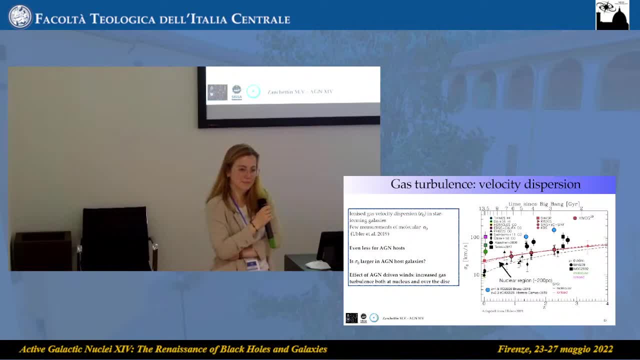 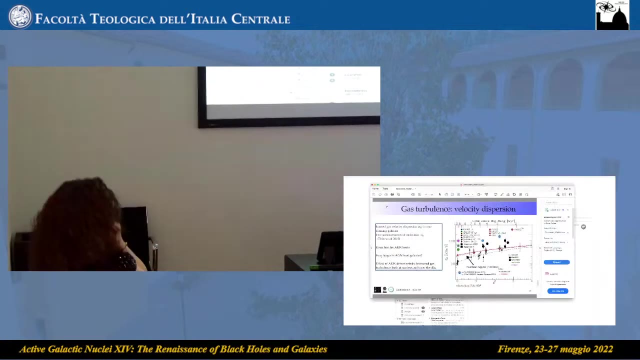 Very last question for Vittoria, Otherwise we move on. Thanks again. So the next talk is by Milena Valentini. host galaxies of higher air shift quasars. So we must be black-host growth and field, Okay. 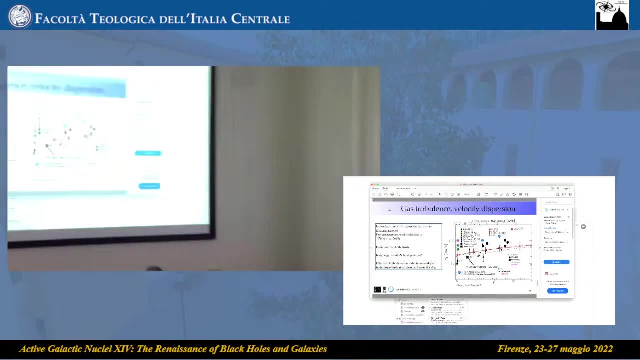 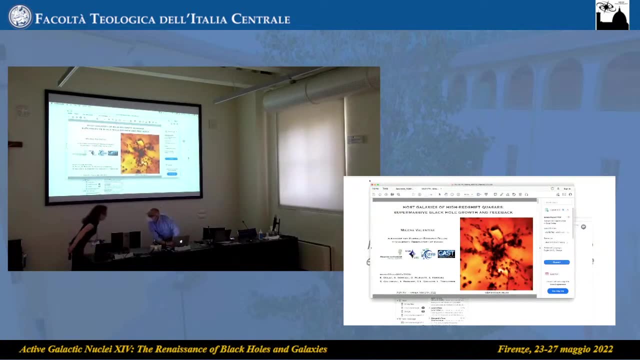 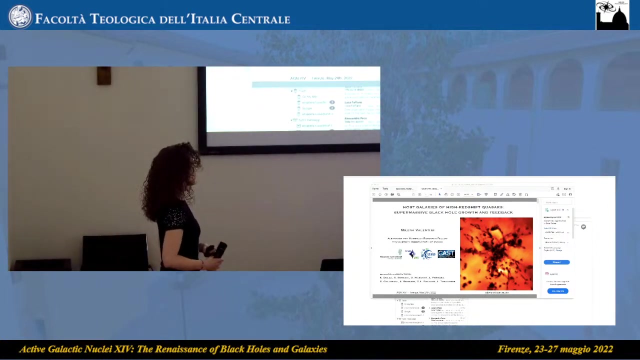 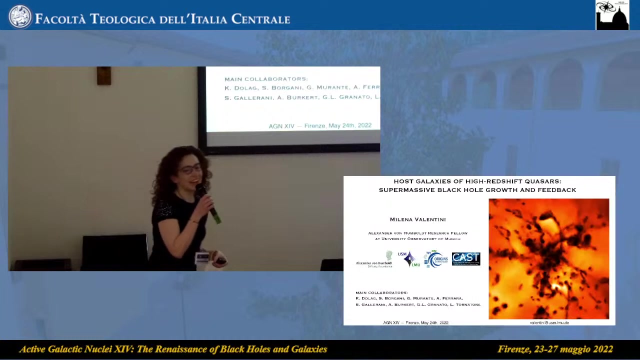 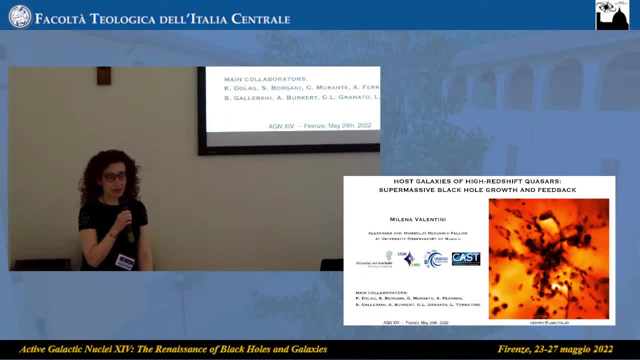 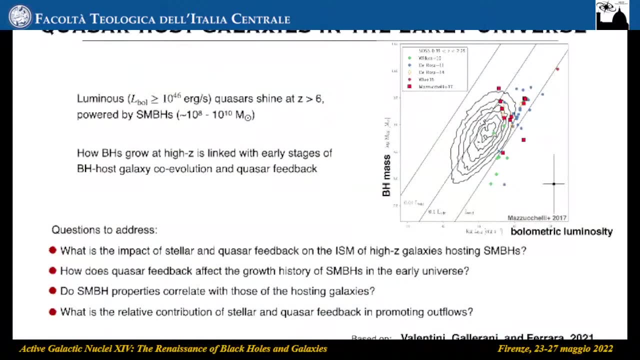 And today I'll discuss the impact of quasar feedback in the citizenship universe from cosmological simulation. A few hundred quasars have been observed in the last decades at high radshift and they have been studied by means of multi-wavelength observations. 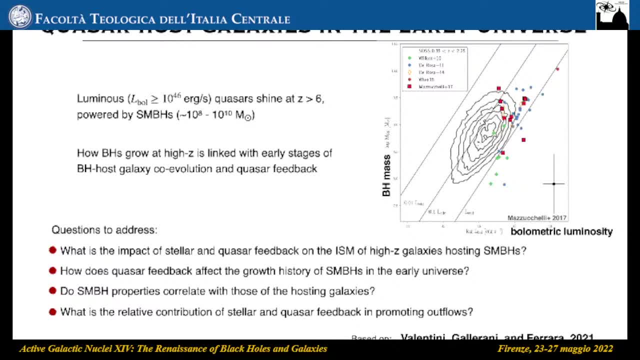 With high radshift. I refer to RadShift 6 and above. These observations suggest that this active galactic nuclei have high volumetric luminosities, as high as 10 to the 46th per second, and are powered by supermassive black holes with 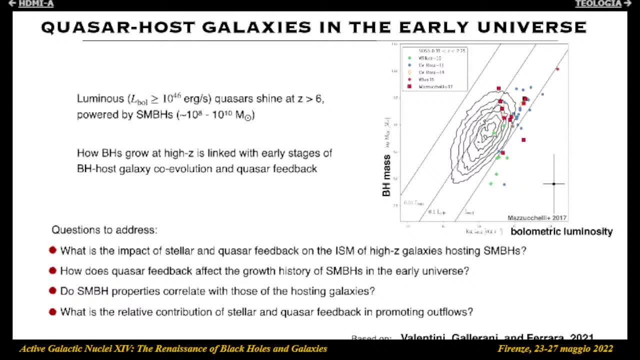 mass in the range of 10 to the 8th to 10 to the 10 solar masses. Of course, the presence of these black holes, which grow supermassive in less than one giga year, puts constraints on the theoretical models of the formation of supermassive 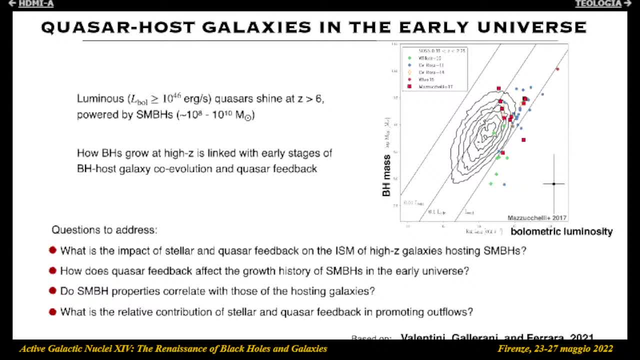 black holes and challenges the theory of black hole evolution, especially as for the mass of the initial seeds of these supermassive black holes and as for the maximum accretion rates that these black holes have to have in order to reach the final observed masses. The presence of these supermassive 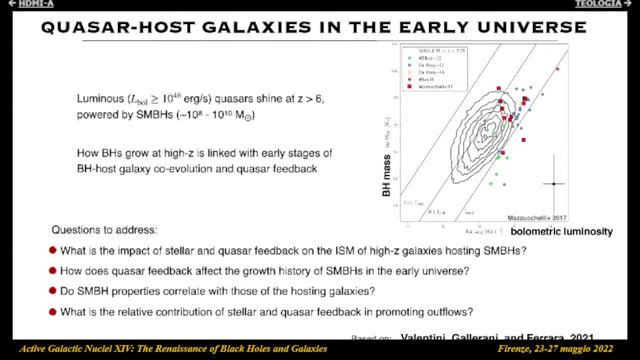 black holes in the high radshift universe is tightly connected to the early stages of the black hole galaxy co-evolution, and recent observations have shown that these supermassive black hole galaxies are characterized by dynamical masses of up to 10 to the 11 solar masses. they have a multi-phase 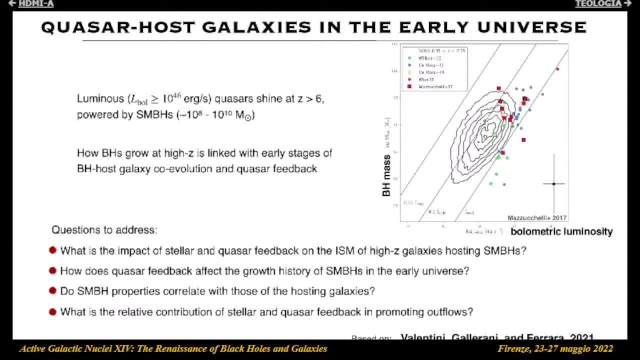 interstellar medium dust, and they host galactic scale outflows which represent one of the main signatures of the ongoing activity of agent feedback. The observational scenario that I've just outlined motivated our numerical study. We simulated the formation and evolution of a high radshift host quasar and focused our analysis at 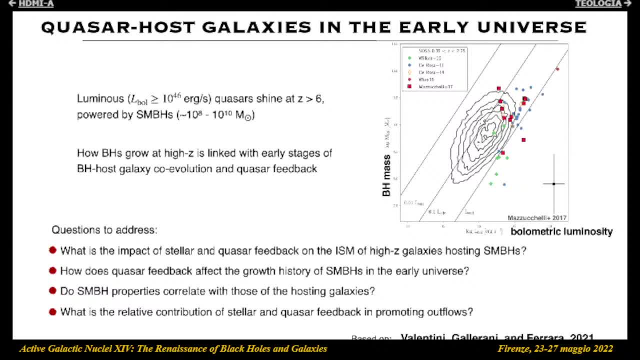 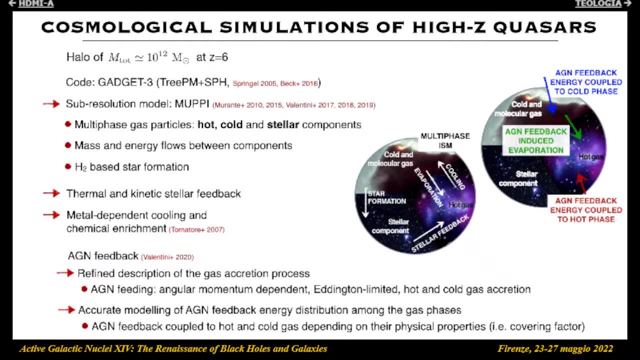 radshift 6.. These are some of the questions that we addressed with our work. So, as for the initial conditions of our simulations, they describe a dark matter halo which is as massive as 10 to the 12 solar masses at radshift 6.. We 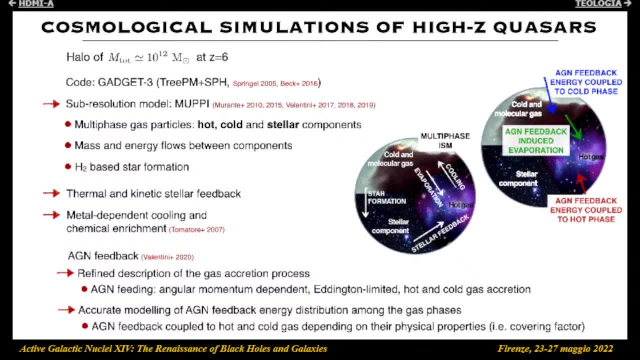 carried out our cosmological hydrodynamical simulations with the gadgetry code and we adopted a sub-resolution model to account for all those physical processes which occur below the resolution limit of our simulation. Our sub-resolution model describes a multi-phase interstellar medium, as you can see from this slide. 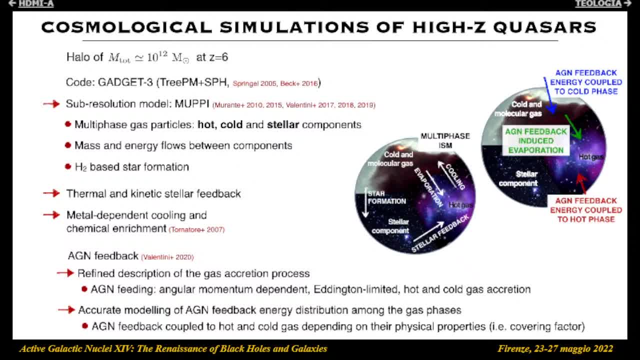 And it accounts for several physical processes such as an H2 base, star formation, thermal and kinetic stellar feedback, chemical enrichment and, of course, gas accretion onto black holes and agent feedback. As for gas accretion onto the black hole, we assume that gas is accreted via a modified bondi formula and 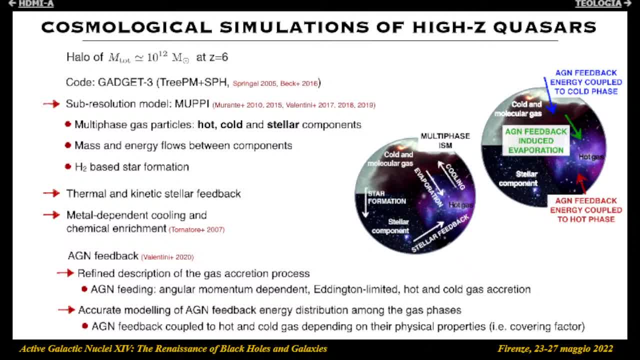 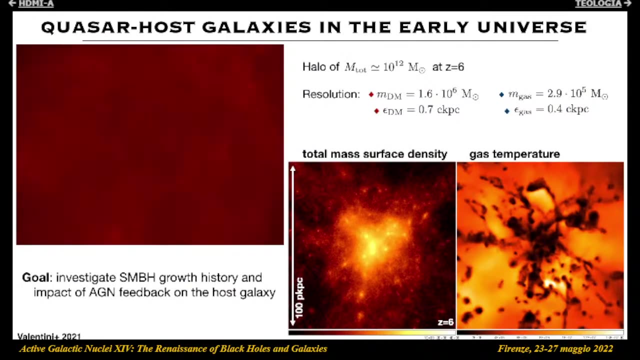 we also take into account the angular momentum of the gas which is accreted. As for agent feedback, we model the distribution of agent feedback energy to the different components of the multi-phase interstellar medium according to the physical properties of the hot and the cold phases. Here we can see the evolution of the central black. 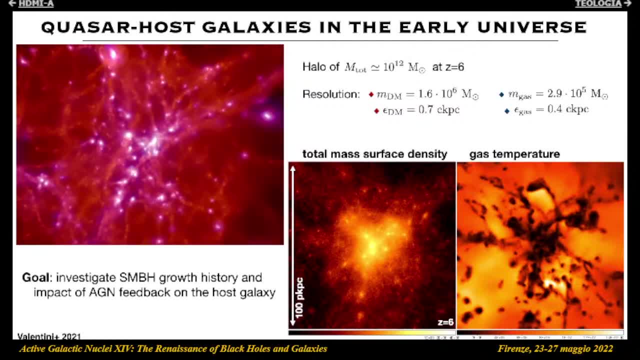 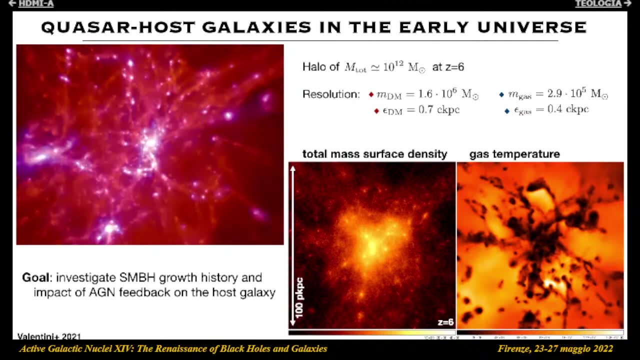 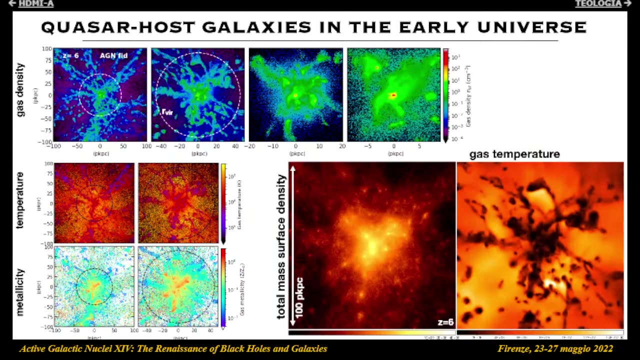 hole within the quasaros galaxy, at the center of the most massive halo of our simulation. and these projected density and temperature maps introduce our cosmological simulation, the innermost regions of our fiducial cosmological simulation, As you can see from these maps, the central 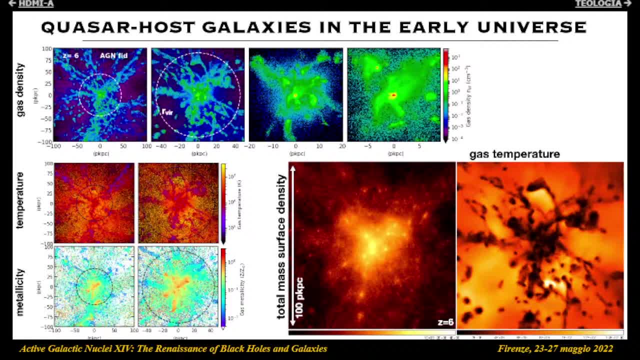 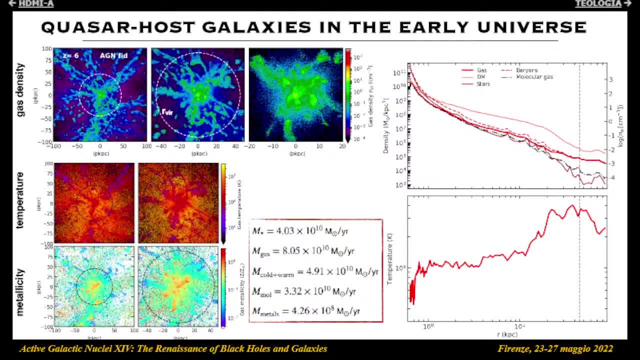 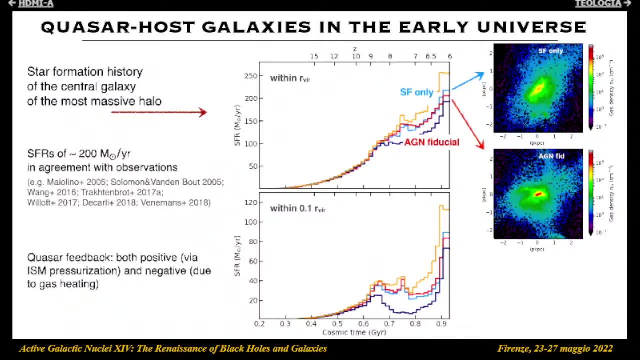 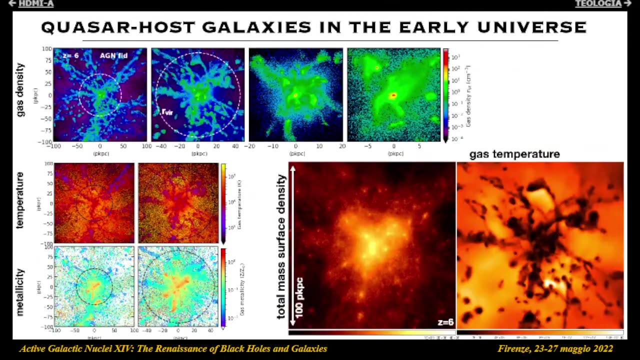 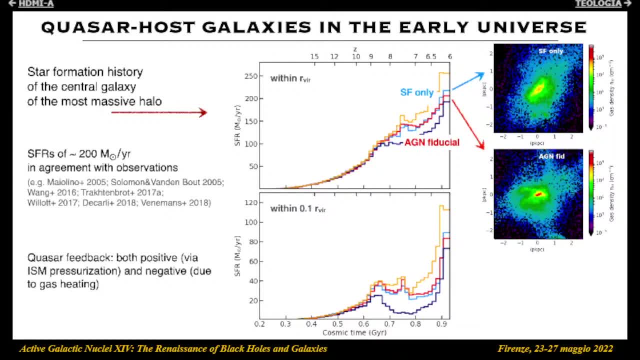 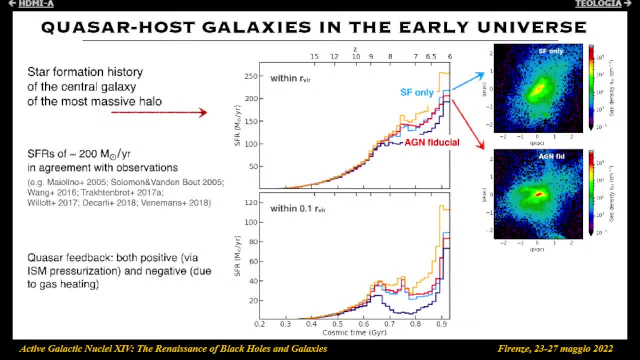 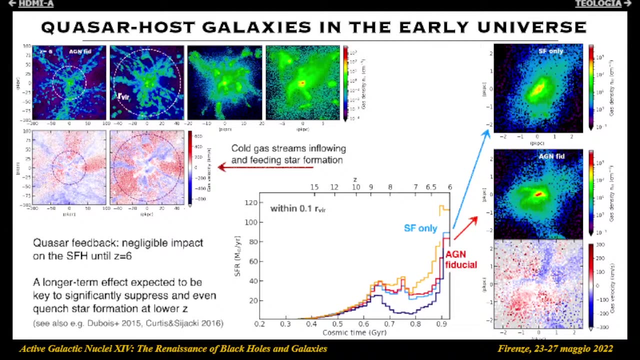 indeed, quasar feedback can over pressurize the ism and dance and thus locally enhance the star formation, but of course it can also heat up the ism and suppress locally the star formation rate. however, we find that the star formation history of these galaxies um is not sensitive um to the effect of quasar feedback, since it is almost completely shaped. 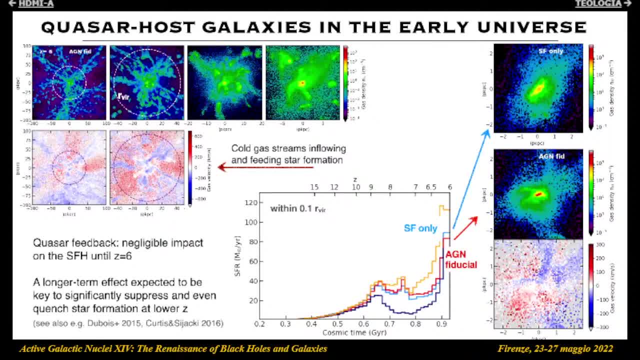 by the cosmological info of gas which is accreted from the large scale structure at redshift six. so we expect that a longer term and more cumulative effect of the quasar feedback is needed to suppress significantly or even quench the star formation later on. 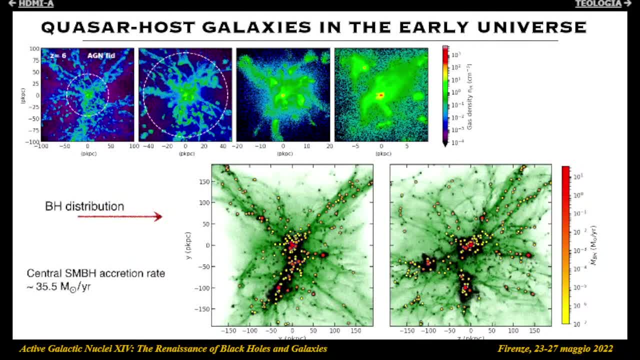 besides the distribution of gas and stars, we can of course analyze the distribution of black holes within the simulated volume, and they are here color coded according to their black hole accretion rate. and the black hole accretion rate of the central, most massive black hole, is of around of about 35 masses per year. we can investigate the location of: 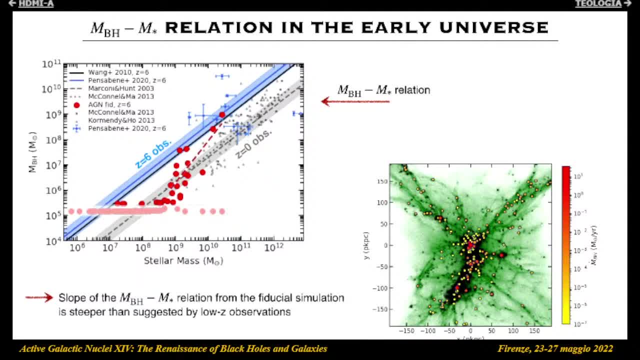 black holes in the simulated volume in the black hole mass stellar mass relation. so we calibrated the agent feedback efficiency of our model so that the mass of the most massive black hole in the simulation is in agreement with high redshift observations. by doing that we see that the distribution of black holes in the simulation is characterized by a slope which is 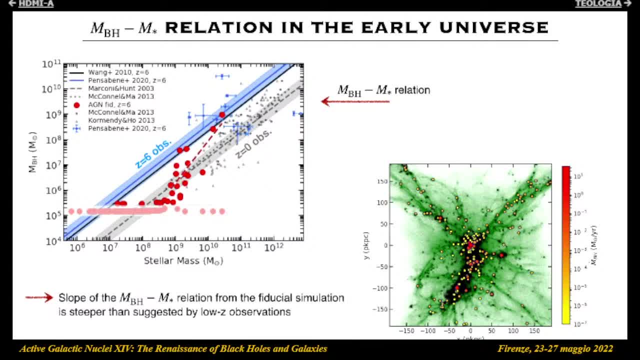 greater than the slope of black holes in the local universe. this is something particularly um relevant, since it is often assumed that the magorian relation only evolves in normalization across redshift, while on the other hand, our study suggests that there is also an evolution as for its slope. of course, we can investigate what happens if we adopt a higher. 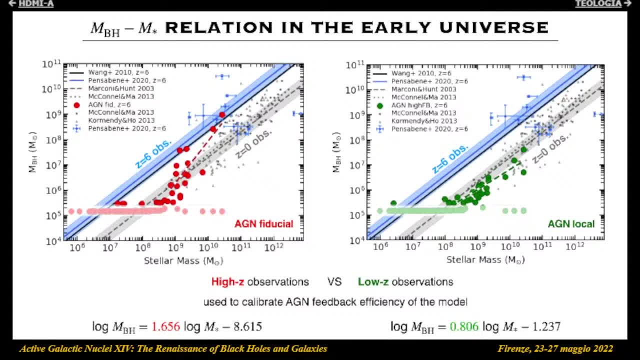 agent feedback efficiency, so that the mass of the most massive black holes is in agreement with observations in the local universe. in this case, the distribution of black holes in the simulation is characterized by a slope which is closer to that of observations in the local universe and way shallower than the slope of the distribution of the fiducial simulation. 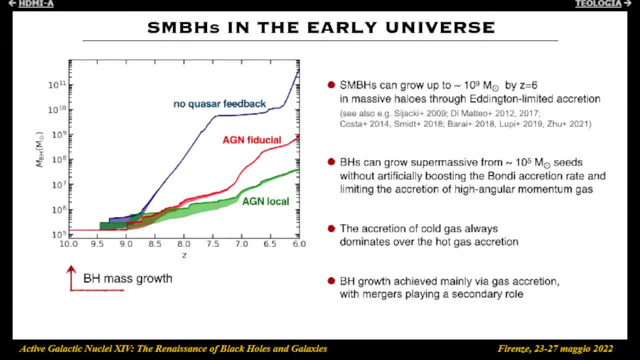 we also analyze the uh evolution of the black hole mass growth for the two simulations that have just introduced and of a reference simulation where the black hole is present and can accrete gas, but no quasar feedback is included. we find that it is possible to produce a super, supermassive black hole, as massive as 10 to the 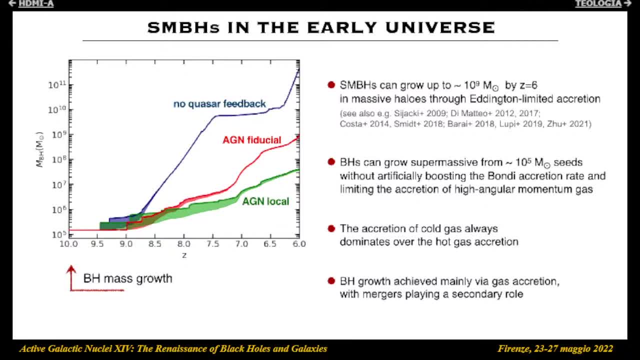 9 solar masses by redshift six, starting from um initial seats, which are as massive as 10, to the 5 solar masses. we found that the accretion of cold gas always dominates over the hot phase and, of course, we also find that gas accretion is the most significant process, meaning that 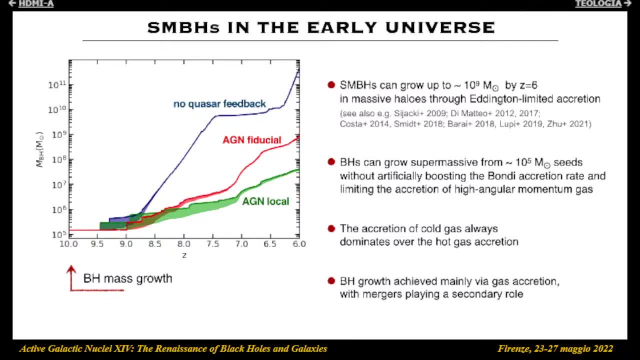 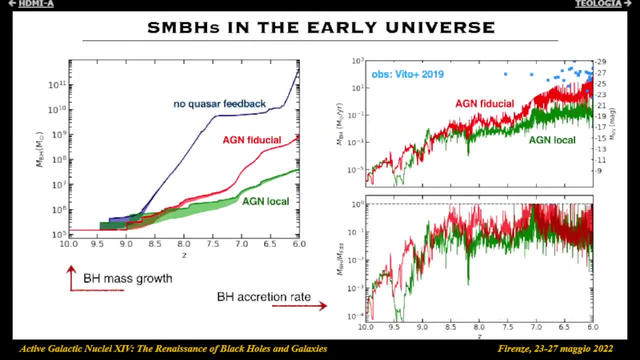 black hole. black hole mergers contributes little to nothing to the mass growth of the supermassive black hole. we can also analyze the evolution of the black hole accretion rate, both in terms of solar gas per year and in eddington accretion rate, and we find that a low agent feedback efficiency. 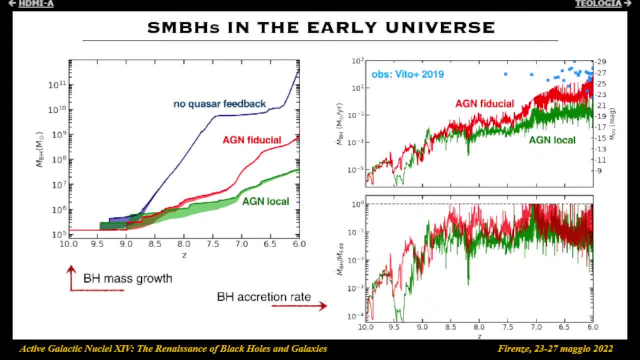 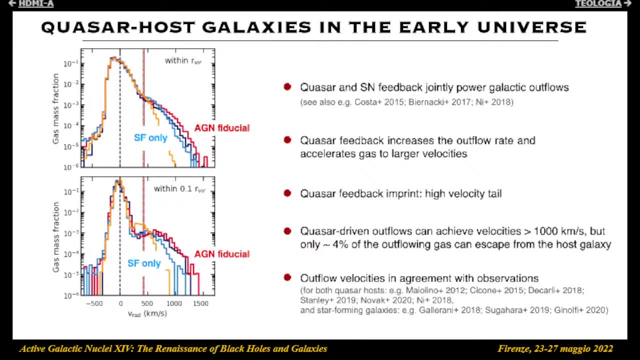 is needed so that the central black hole can be in agreement with observations of supermassive black holes in the high redshift universe. we also analyze the distribution of outflowing gas. in our simulations, outflowing gas is promoted by the joint activity of stellar and agent feedback, and we quantified 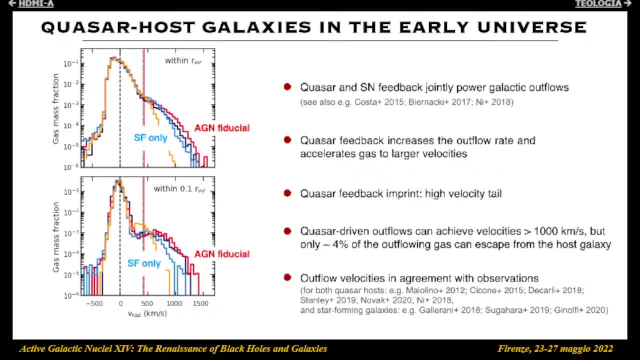 the relevant importance of these two processes. we found that quasar feedback is able to accelerate outflowing gas to highest velocities and leaves a significant imprint on the high velocity tail of the distribution of the outflowing gas. velocity of the gas in outflows is in agreement are 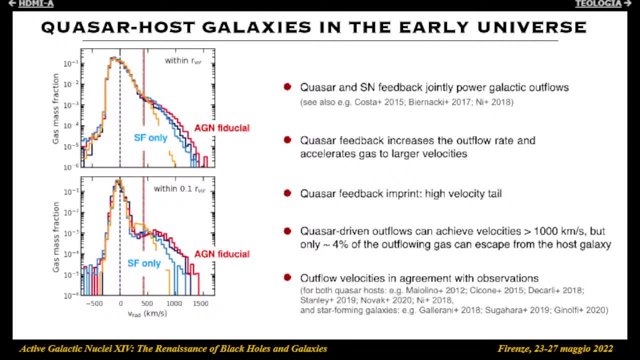 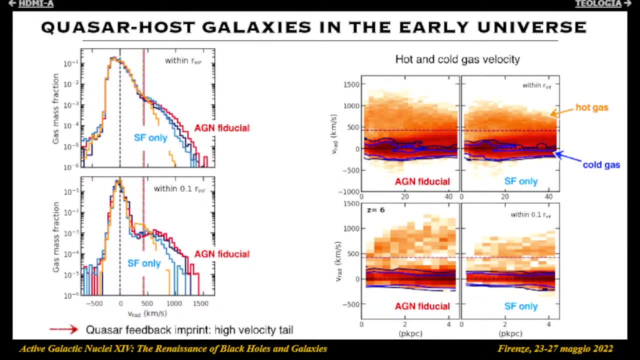 in agreement with observations. and of course we can also investigate the radial velocity of different phases involved in outflows. we analyze the evolution, so we analyze the radial velocity as a function of the distance from the galaxy center, and here we focus on on coal gas and the hot and diffuse phase. 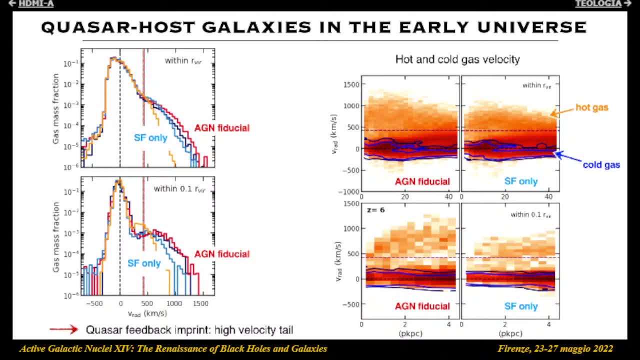 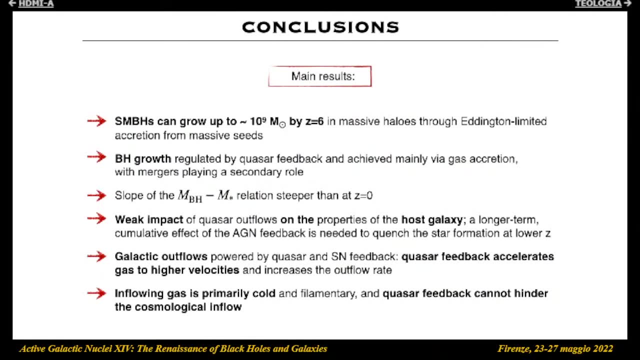 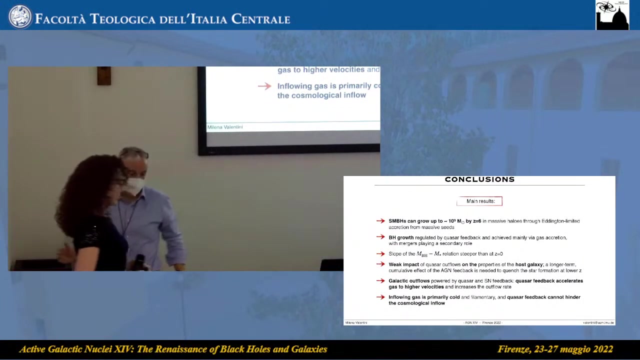 We see that coal gas can be accelerated up to roughly 300 kilometers per second, while the more diffuse phase can be accelerated to larger velocities. I leave here with my conclusions and take questions. Thank you very much. Questions for Milena Hi. did you test your model on different seeding mechanism? 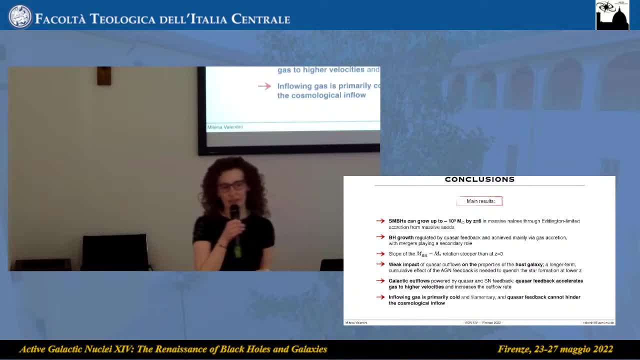 of the supermassive black holes. No, we assume massive seeds which are the likely outcome of direct black coal collapse scenarios. Okay, okay, So. and the mass threshold is So: their seed mass is 10 to the five solar masses. 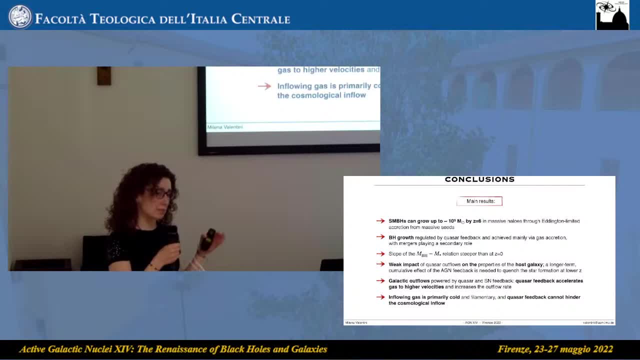 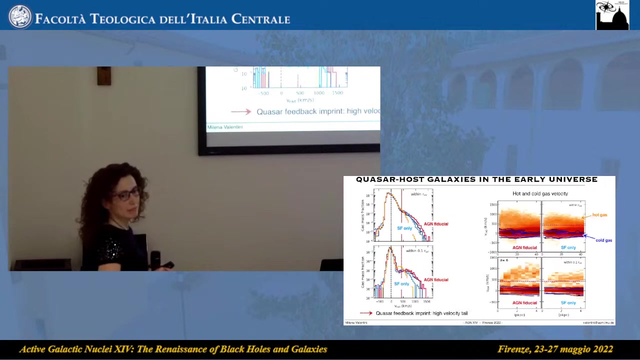 and they are seeded in halos which are as massive as 10 to the nine solar masses. Okay, thank you. And they're either Parce нашor of the. Can you go back to the last slide? Not this one? Okay, the one with the different phases. So you're saying that the coal gas can be accelerated at most of the odd a few hundred kilometers per second. but then the observation. the evidence that we have in the early universe from observations point out to even larger velocities for molecular outflows, at least looking at the references that were put before. So when we say cold gas, actually we refer to both the cold and warm That the molecular gas makes up the bulk of the outflowing gas, but of course here we also include the warmer phase, which has a temperature of up to a few hundred Kelvin. Very last question. No, I was just thinking that the hot phase, when by hot I mean 10 to the 6 Kelvin- I don't know if this is the temperature you have in mind. Okay, These velocities actually should have been seen already, at least in our galaxy, in oxygen. 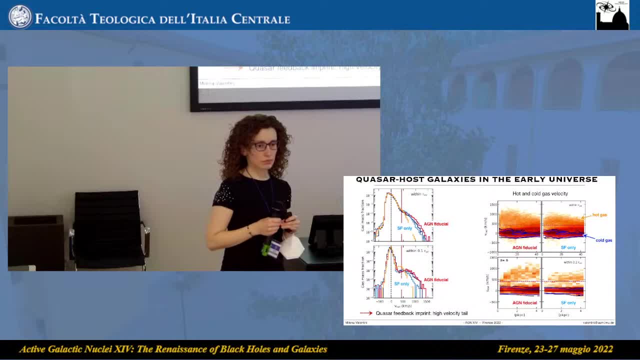 7 absorption and we actually don't see such high velocities In our galaxy. Yes, they should have been resolved in absorption by the RGS, for example. The centroid is known to a few hundred kilometers per second. I don't know whether it was a comment, meaning that we are focusing the analysis at redshift. 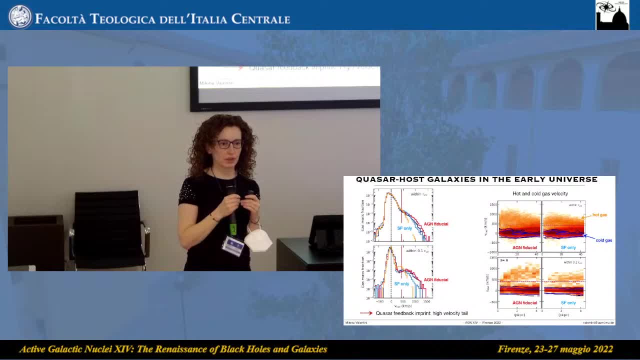 6 and I don't see the connection with: I'm sorry, We are focusing the analysis at redshift 6 and I don't see the connection with observations. No, no, no, I know, but if these objects have these velocities at redshift 6, probably also. 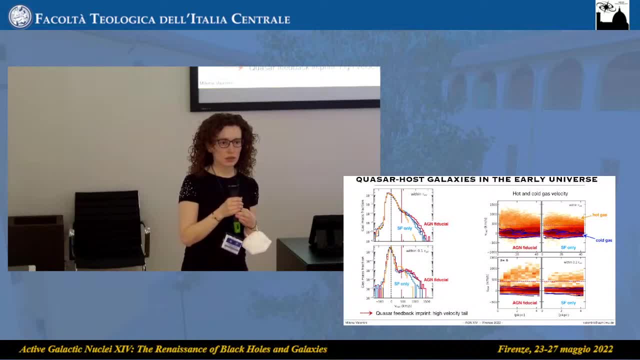 at lower redshift, the CGM should have this imprint. no, It might be. maybe we can discuss at the coffee break. we have to move on. Thanks again, Elena, And the next talk by Andrea Travascio. let me read the title. 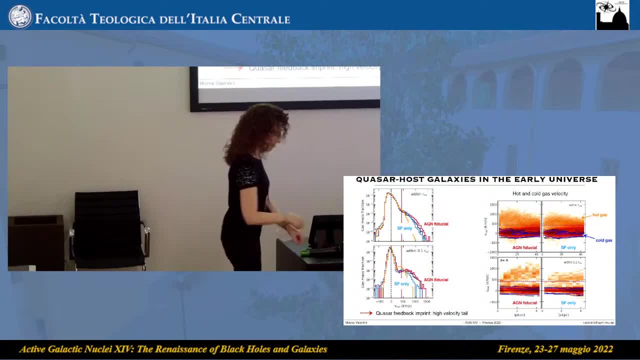 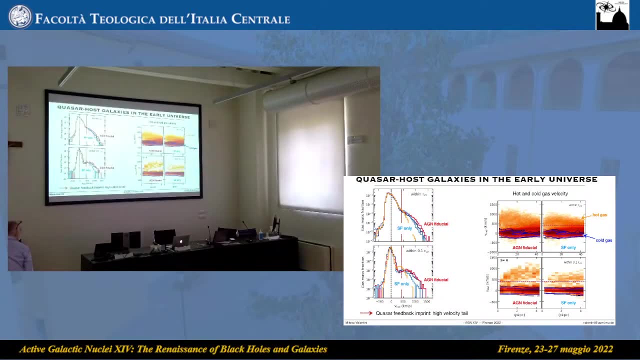 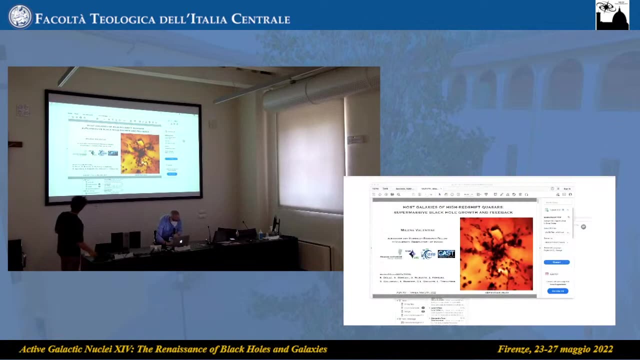 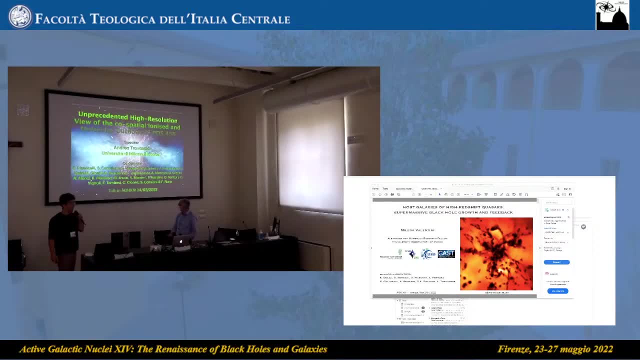 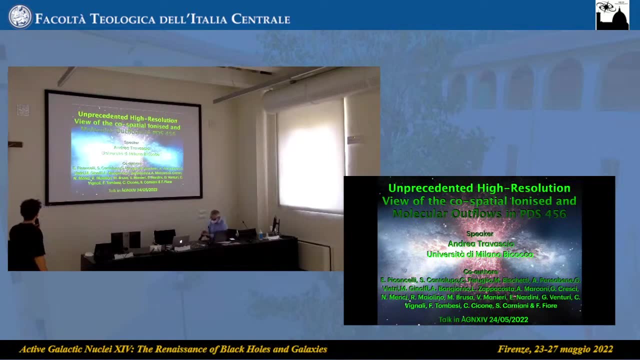 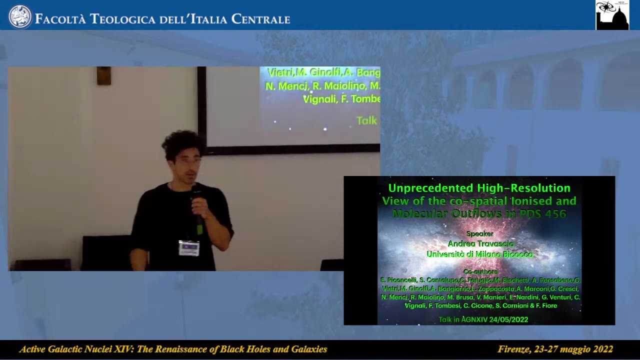 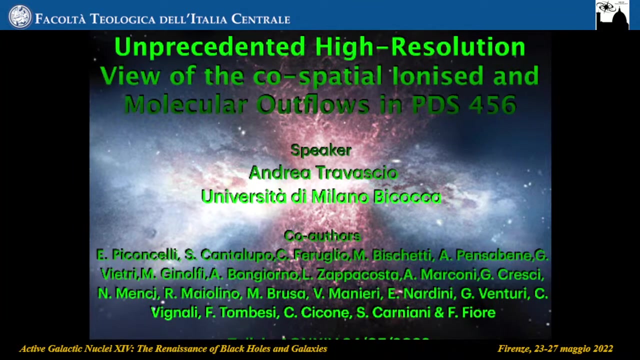 I want to present to you some first restores. all work in progress, please. comments are welcome. Good work-in-progress in which me and co-authors investigate multi-phase outflows in a hyperliminal quasar with unprecedented spatial resolution, with narrow field model muse data. So studying multi-phase outflows is. 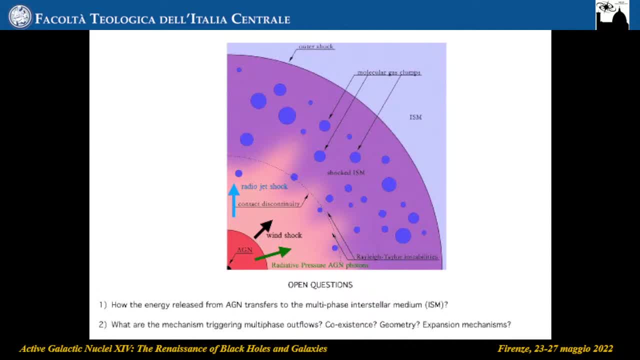 interesting because it helps to get more information about the agent, feedback for how the agent can impact the host galaxy evolution. and here just briefly let me say that, as also Maria-Vittoria mentioned before, the energy risk by the agent as jets or relativistic nuclear winds, but also radiation, can have an. 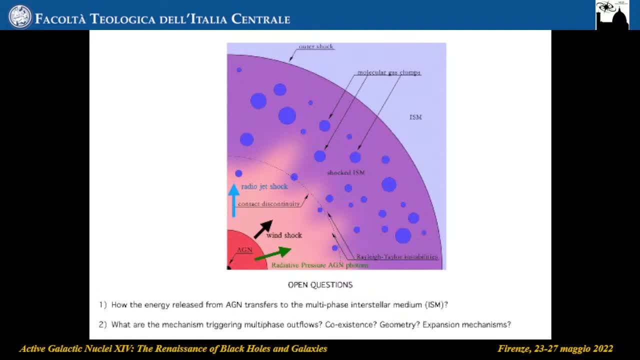 impact on the multi-phase interstellar medium, triggering galactic scale multi-phase outflows, and the situation is a bit more complex. indeed. there are lots of questions regarding, for example, the impact of multi-phase interstellar medium and the impact of multi-phase example, the way in which the energy is transferred to the multi-phase interstellar medium, but 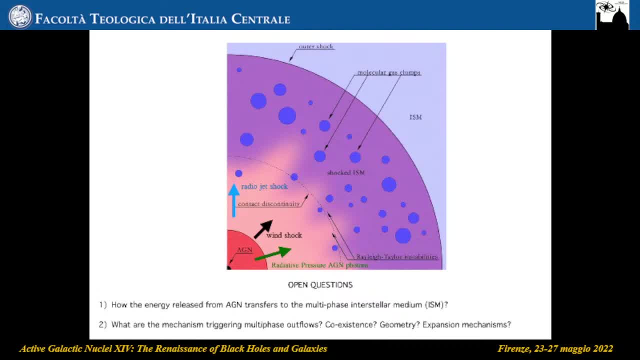 also about the expansion of these galactic-scale outflows. We don't know if multi-phase galactic-scale outflows are triggered by the same mechanism. We don't know what is the geometry of these multi-phase outflows and we don't know what. 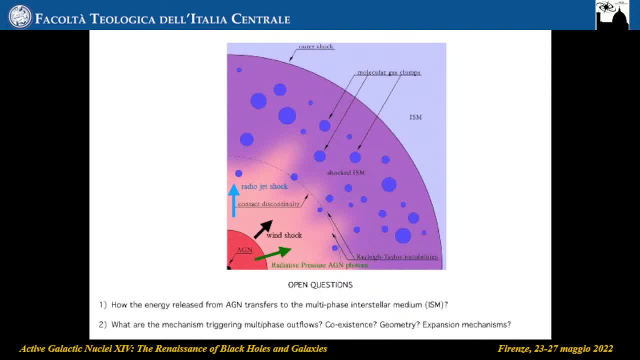 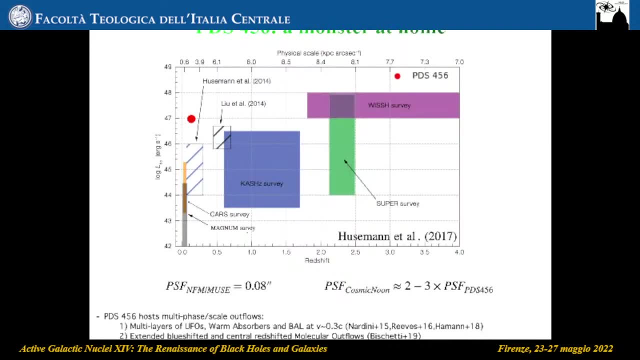 is their impact on the, if they have a different impact on the galaxy evolution. Therefore, why PDS-456, that well, PDS-456 is stunning. PDS-456 is a great opportunity to investigate multi-phase outflows in a very important detail, in particular, if it is observed. 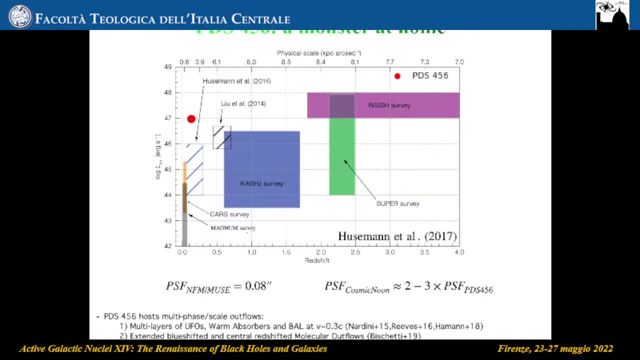 with studied with the Narrow Feed Modules data, for two reasons actually, because here you can see a plot, redshift versus barometric. You can see the barometric luminosity by use metal, in which they show also different characteristic features of characteristic of HGN in sample studies so far, and you can 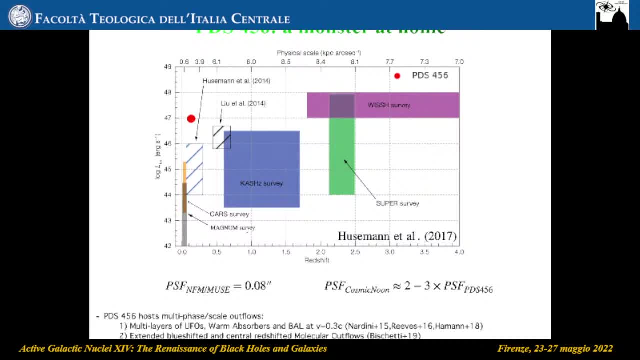 see that PDS-456 represents the most luminous quasar in the local universe and it can be seen as a local counterpart of hyperluminous quasar shining at the cosmic noon, like, for example, wish quasars. What this means? it means that we have a laboratory of hyperluminous quasar where we expect to 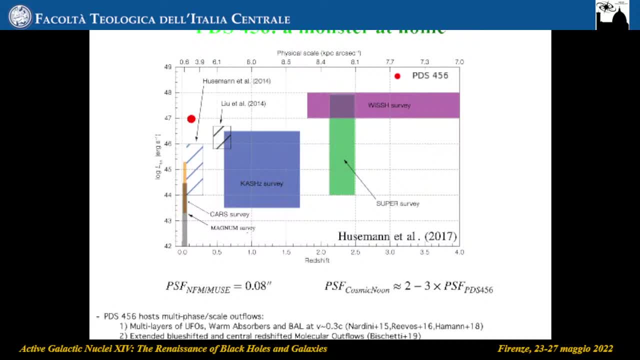 have a high efficiency of HGN feedback, radiative HGN feedback In the local universe. therefore, thanks also with narrow, a powerful integral for spectrograph Narrow Feed Modules data with adaptive optics, we can achieve a value of the PSF 0.08 arcseconds. 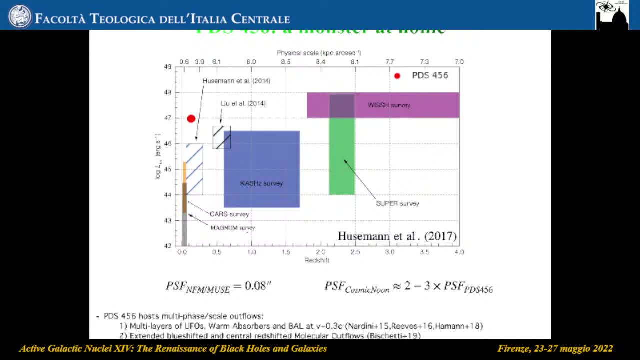 and therefore it could be two, three times higher, lower than typical PSF that we would have with, by looking at wish quasars, for example. Second reason is that it hosts very important, very powerful winds, The most powerful ultrafast outflow never observed, but also warm-absorbent and broad-absorption. 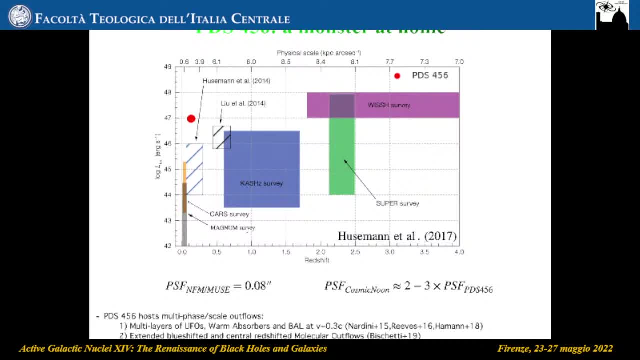 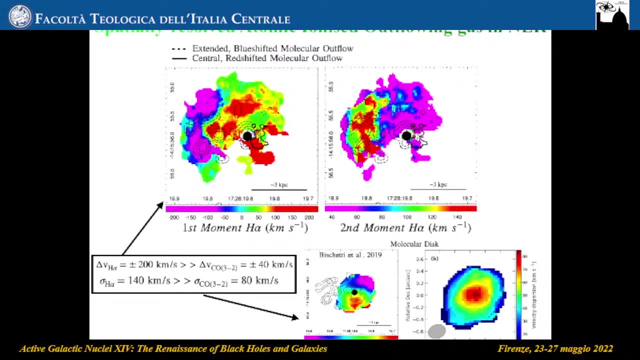 line of outflow in carbon-4,, each of them with velocity 0.3 speed light, and also by Bisqueti et al. with ANMA has been detected an extendably shifted and uncentral redshifted molecular outflow. So going going to see the results. the first results. 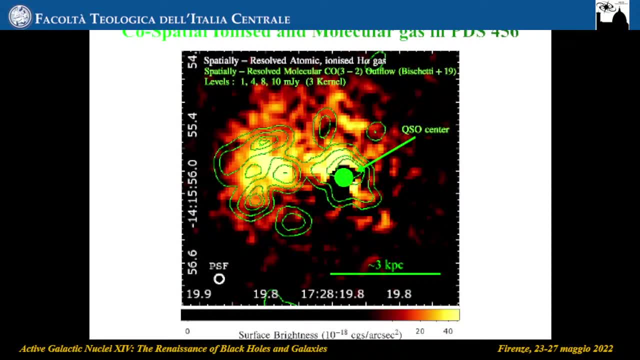 By subtracting PSF and continuum of the quasar, We can start it in this data: the HF emission line, nitrogen emission, nitrogen-2 line and sulfur-2.. Here I show you a sulfur brightness map of the spatially resolved HF emission. 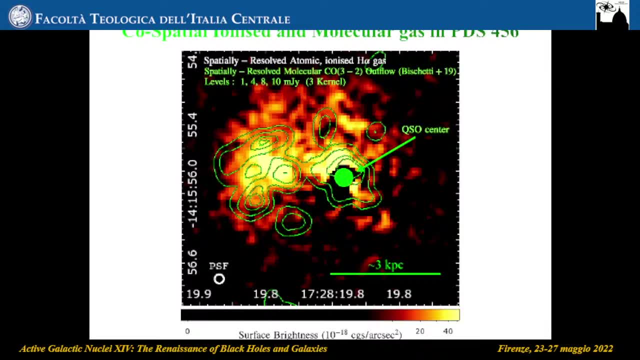 And the green contours here represent the morphology of blue-shifted molecular extended outflow detected with ANMA. You can see just here a correlation, a spatial correlation between the multi-phase gas, therefore ionized atomic and ionized atomic gas, and molecular gas. 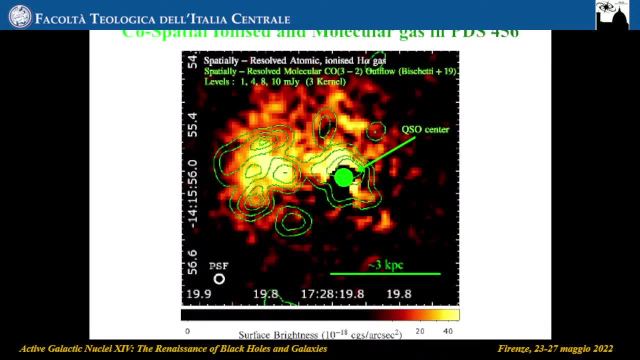 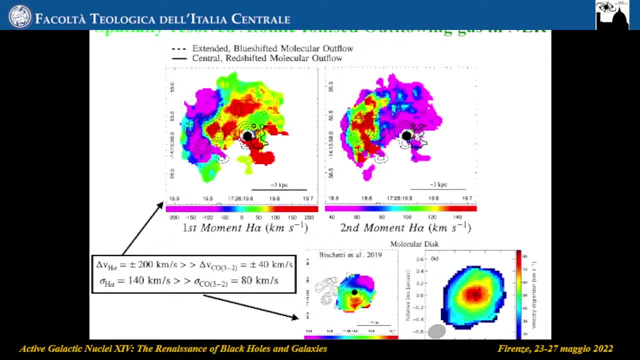 And those are clumpy HF region at the position of the bulk of the molecular outflow, suggesting probably a connection between them. And looking at the kinematics, morph kinematics maps of the HF spatially resolved HF emission, you can see, and here you can see here this velocity shift map. 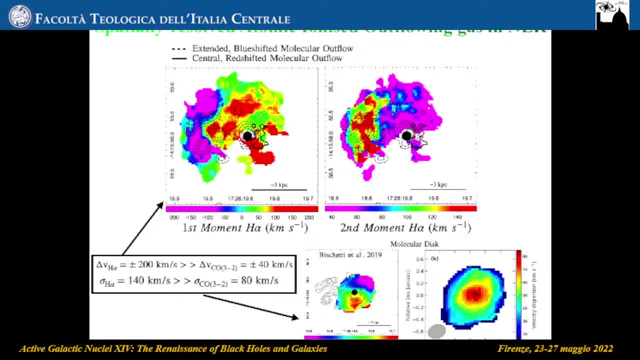 Here the velocity dispersion map. The dashed by contours again are blue-shifted extended molecular outflow, while here you see the central red shift and molecular outflow in a black solid line. while here you see the same velocity kinematics map for the molecular disk detected with ANMA. 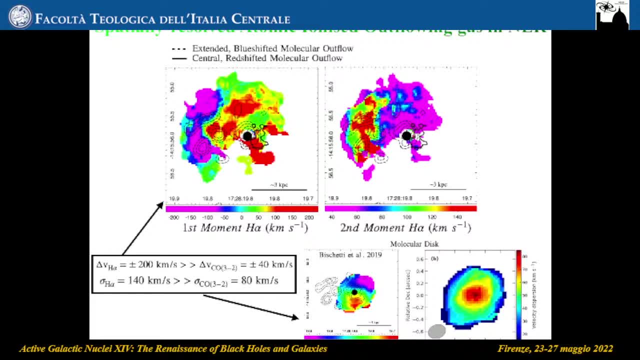 And you can see that here we have extremely larger velocities than what you observe in the molecular disk. But also the morphology, the kinematical pattern suggests that this HF emission is probably tracing outflow. Therefore what we assume here- and it's plausible- is that this represents ionized outflow observed. 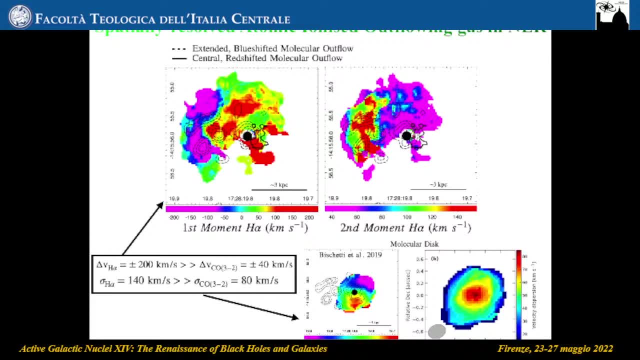 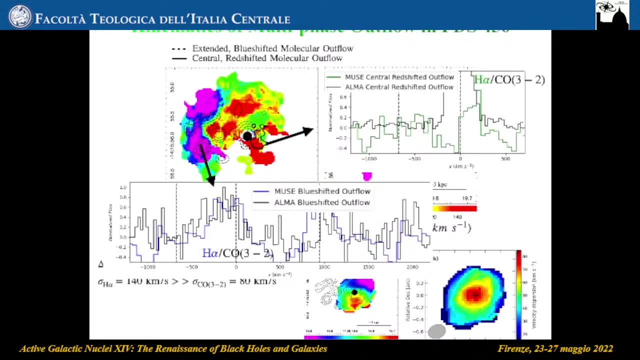 in the narrow-line region. You can see that we have- it is spatial correlated also- the high dispersion region with the molecular outflow. So looking at the kinematics in these two regions, in particular the blue-shifted components, both in molecular and ionized outflow, and the red-shifted central components, here you 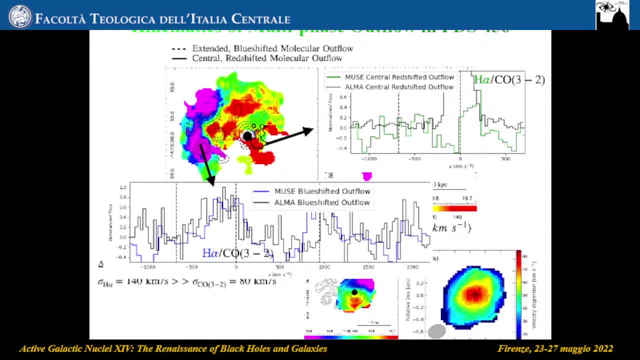 can notice a strong correlation between the kinematics of the CO2 emission, the molecular outflow and the ionized outflow. You can see here black spectra extracted from ANMA in the same region of blue-shifted outflow and the ionized outflow. 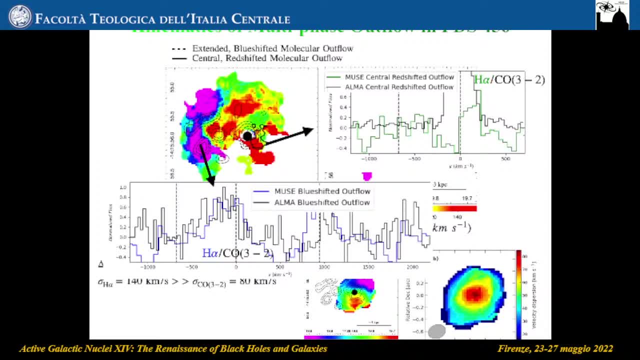 of colored spectra extracted from MUSE and you can see that for the blue shifted component we have same kinematics of H-alpha-HCO3-2 emission shifted at the systemic ratio of the quasar estimated with CO3-2, and here we have also we have to compare the wing. 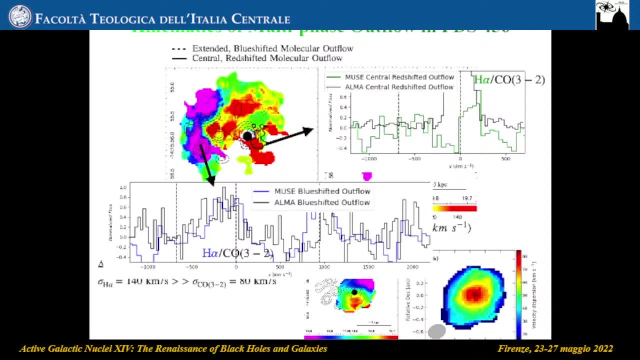 of these emission lines that it is due to the fact that in ALMA we have not subtracted the PSF, so we are observing the molecular disk, and this line is the H-alpha line, and also here in this case they have quite similar kinematics. 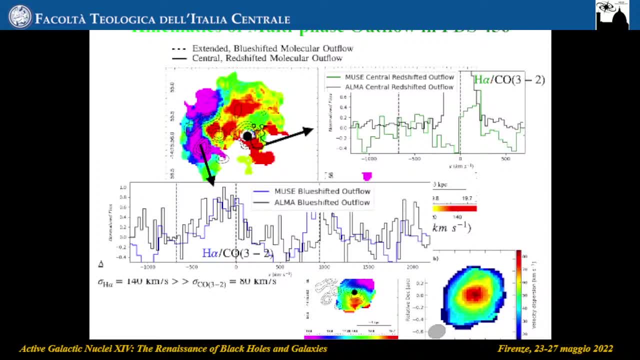 So what we found from here is that we have special correlation. we have similar kinematics, except for the fact that for the ionized outflow we have a shifted component that we don't see in the molecular phase. Now, driving from the question, 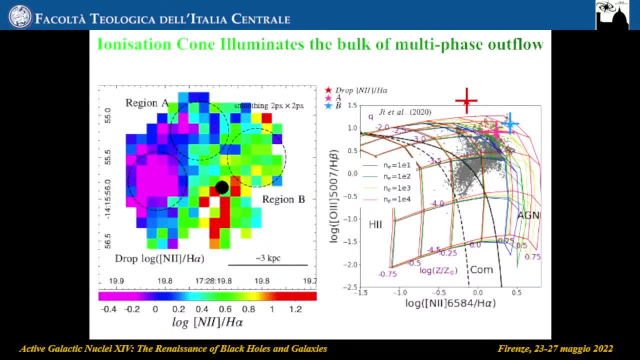 so what properties this gas are. we are going to see the nitrogen to H-alpha emission map and what you can see here is that there's a drop- interesting drop- in nitrogen to H-alpha emission that is specially correlated both with H-alpha clamp region but also with the 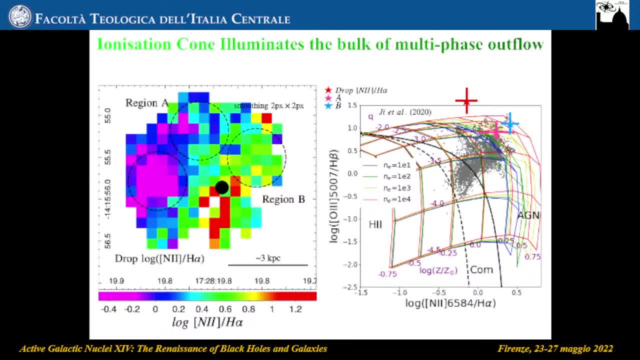 bulk of the multi-phase outflow. Now what we can do is just looking at extract the nitrogen to H-alpha emission in these regions and, as we have also Weifel-Mod's MUSE data for this object, but I don't have time to discuss about that. 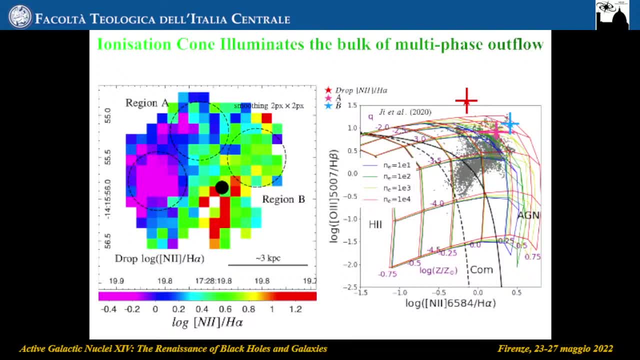 but we have in that data information about oxygen to H-beta. we can also extract from here this information about oxygen to H-beta ratio line in these regions because they have the similar size of the PSF of Weifel-Mod MUSE data. and by extracting this and putting 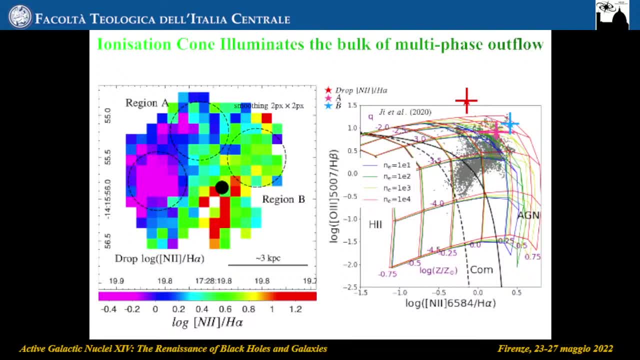 in this BPD diagram. we obtain these three points here. The red one is the drop of nitrogen to H-alpha ratio and we compare it with cloudy photoionization model from G et al, in which they assume a typical agent set, and you can see that. 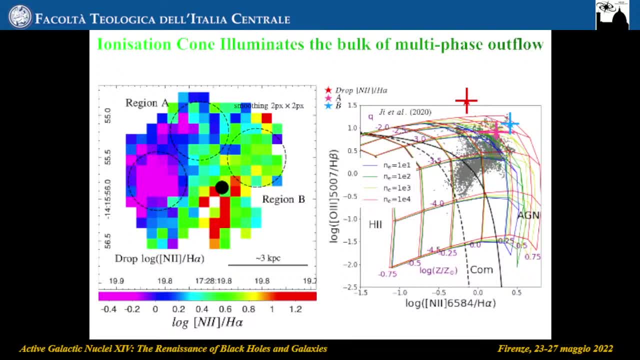 surprisingly, the points follow the trend of these grids, In particular suggesting that this, This is the, This is the, This is the gas emitting gas in these different regions can be considered at the same metallicity. Indeed, you can see here fixed metallicity for these lines and fixed ionization parameter. 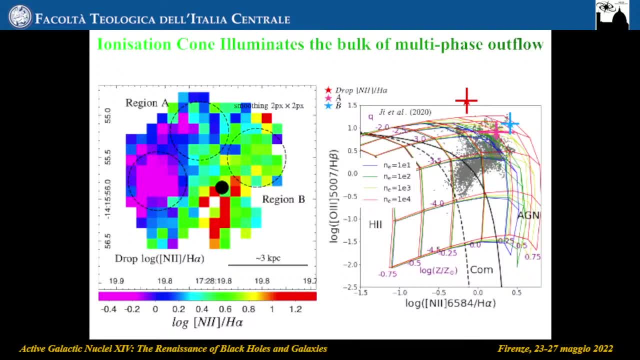 for these lines on similar electron density that we could fix up 10 to four centimeters minus 3, and what exchange is the ionization parameter? and this is not strange because there are a lot of other observations showing that a drop in the nitrogen to H-omission. 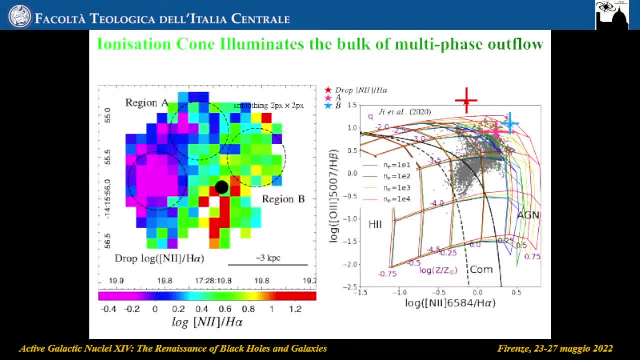 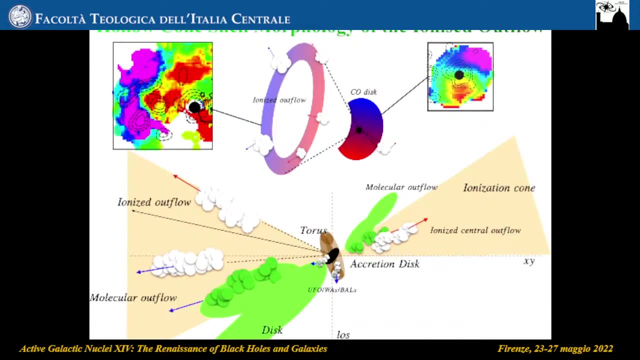 to the presence of ionization cone. Therefore, what you're observing is that the bulk of this multiphase alphalus corresponds to a region in which there's ionization cone. here, Very well, so. okay. so, taking all the kinematics, map, morphologies and what we obtained from the first results, we can develop a. 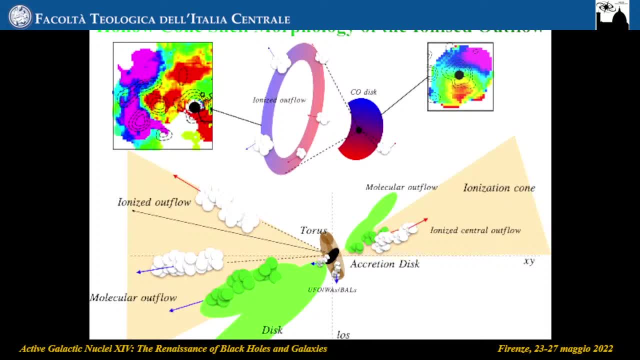 scenario for the geometry and the expansion and the mechanism involved. the geometry, and then, well, the spatial correlation between multiphase ionized outflow. What we can see here is that, okay, what? based on the Martin kinematics, we assume that this has a holoconcial geometry. the ionized outflow. 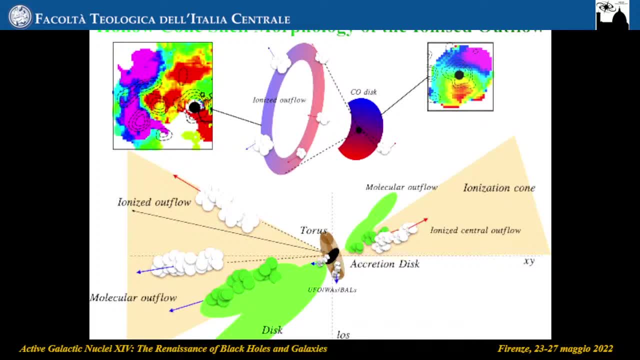 that I show here, while the molecular disk is observed, Observed in face on, according with the estimations in Biscayte-Yedal, with a slight angle of 25 degree with respect to the line of sight, While looking at a different perspective in which here that's the line of sight and here the XY plane. 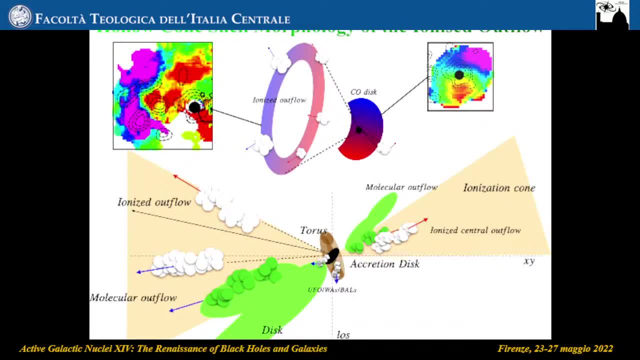 which the maps lie, You can see that the angle of the ionization cone has to be that is not perpendicular to the line of sight, but has we need? we have to consider an angle in order to explain the fact that we are observing a blue-shifted component, a larger distance. 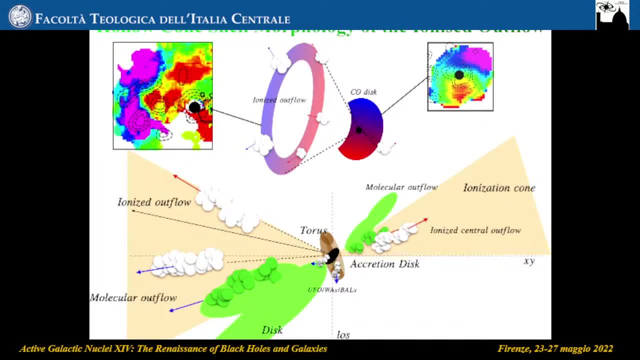 from the center with respect to the similar components. Moreover, the presence of only blue-shifted molecular outflow suggests that the molecular outflow has to be in front of the ionization cone and therefore we are assuming that this configuration in particular. we assume also that the molecular disk has to be 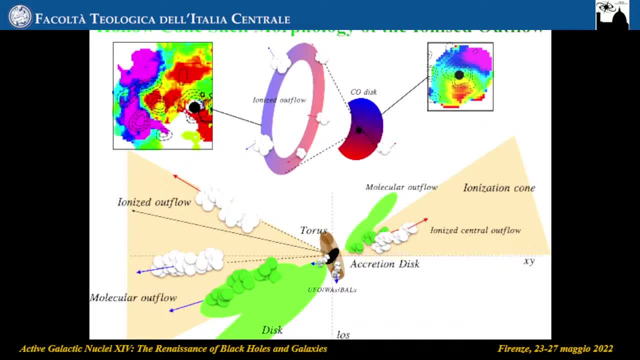 oriented in this way in order to explain molecular outflows as sweep molecular disk gas after the impact of radiation or winds. the nuclear region is difficult to constraint, while the redshifted central multiphase outflows can be explained in the same way. therefore is a mirror case of this site. this is how it's possible. 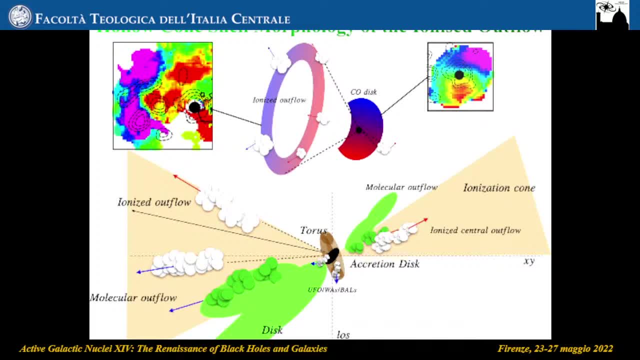 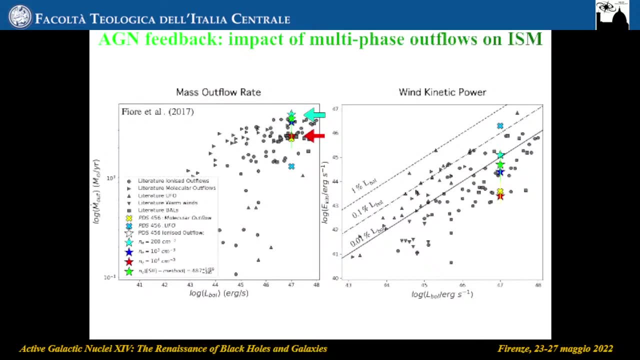 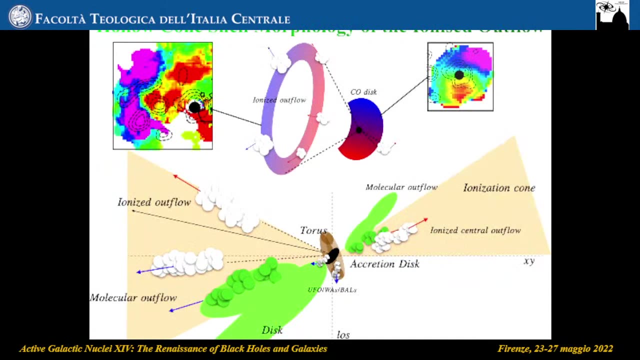 thanks the high resolution that we achieved in this data, while if we want to be sure about the same, I mean we are suggesting that probably the molecular ionized outflow are triggered by the same mechanism. to be sure about that we need to see the energetic properties of these outflows. here I show you. 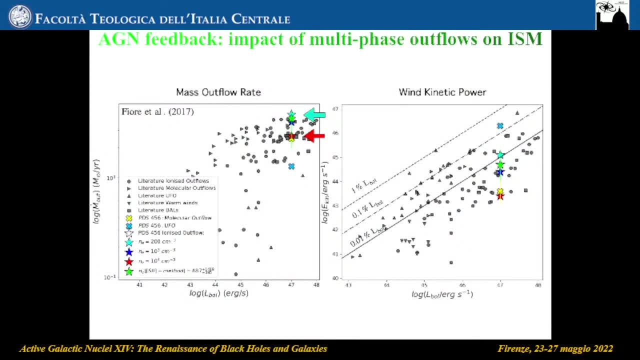 volumetric luminosity versus mass outflow rate and wind kinetic power, and you can see that these are values obtained by Fiori et al, assuming a fixed electron density, 200 cm3. this in blue and yellow crosses are molecular and ultrafast outflow in PDS456. 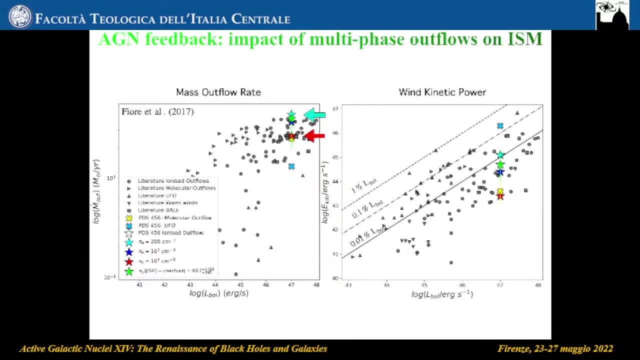 while stars represent ionized molecular outflows, considering different electron density, that are very hard to constrain. in this case, let me just focus on the China one. therefore, the 200 cm3 that is, that one that allows us to compare this PDS, this ionized outflow, with the rest of the of the 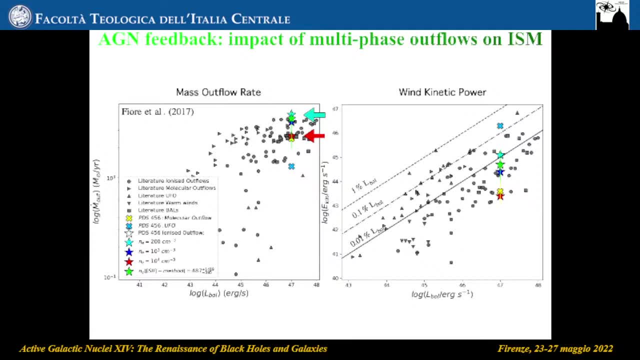 population observed in gray color here and the 10 to 4 cm3. that because it is the most plausible electron density considering the formalization cloudy models and you can see that we are not conclusive. we're not conclusive. entire workshops since 2010 hint about that because just say that if we 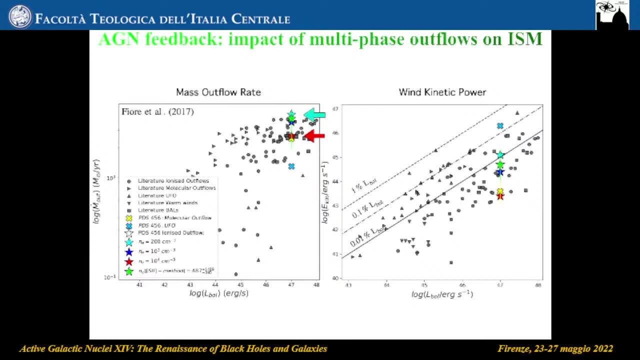 assume low electron density, we can say, okay, this is a very powerful ionized outflow, it has very large impact on the host galaxy and gone, okay, did what we expect. because I'm considering that I was on the show leading the whole winner here and that I would have gone as a short break today, so I will stay in our chat. 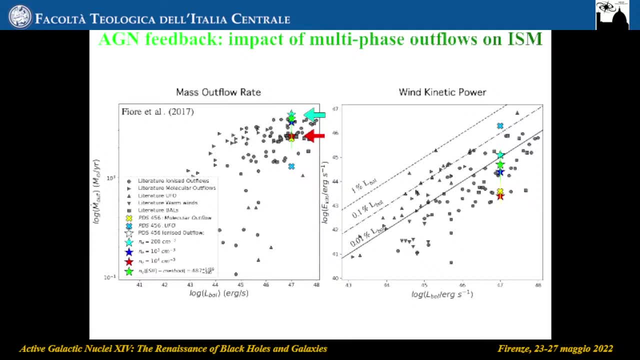 this is a very high luminous quasar. if we are considering the high electron density, we say okay, we have similar energetic properties of the molecular hot flow and therefore it's the fact that the molecular units are triggered by the same mechanism is strength, is more strength also. this plot is very 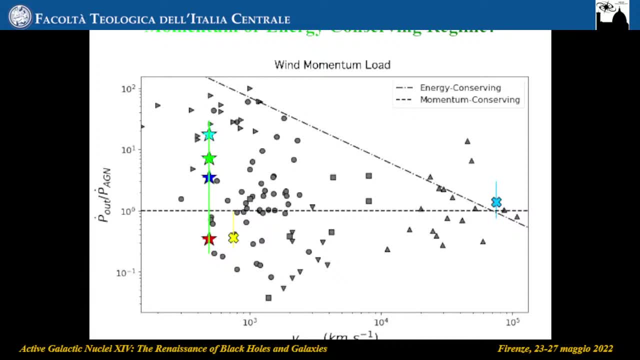 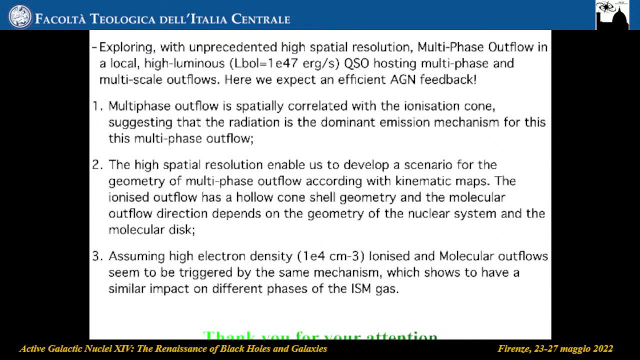 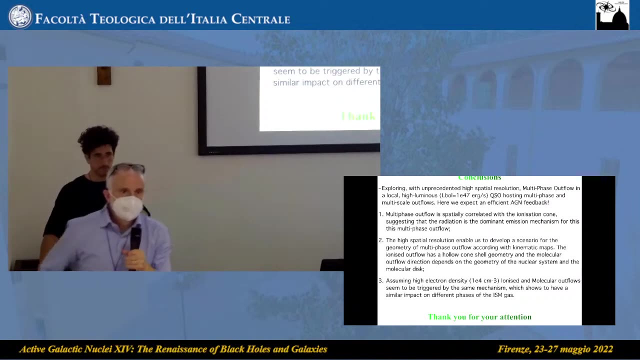 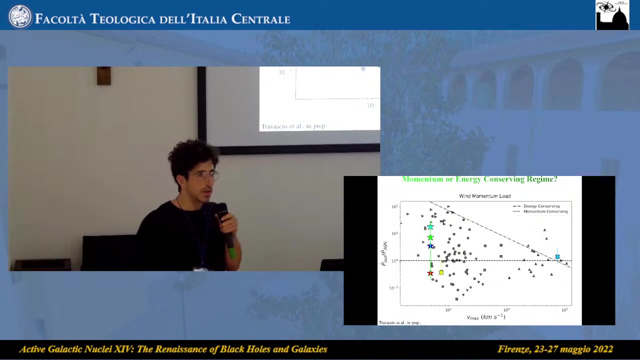 complicated, but anyway, let me skip about this, and so these are conclusions. thanks, thanks, andrea. we have just one question for andrea. we are running late. yes, no, just if you can go back to the previous slide about the conclusion on momentum or energy conserving. yes, sorry, no, if you just comment on this. 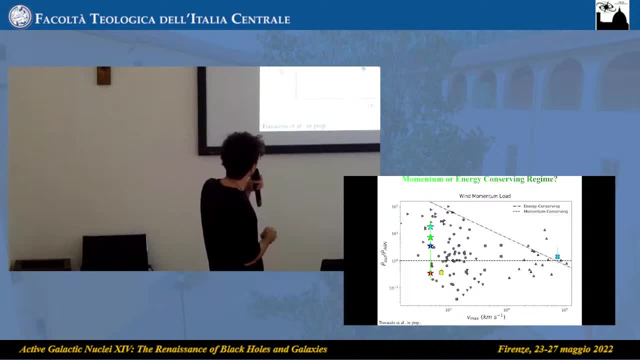 slide. yeah, well, the fact is that here we found a very low value that was expected, against the theoretical expectations, because it suggests that we are observing a molecular hot flow in a momentum conserving regime, and what we expect is that. okay, we assume that, due to the high volumetric luminosity, we 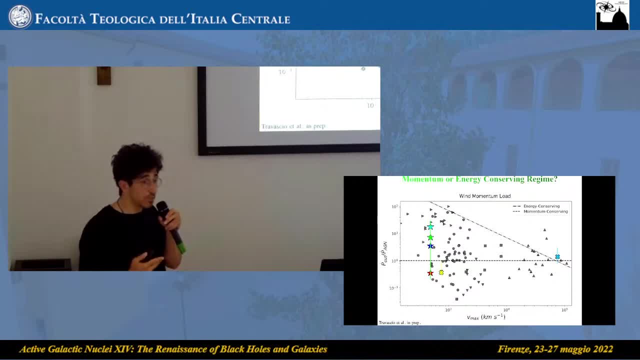 assume that the ionization, the ionized hot flow dominates the system, and so we expect to have something like that and therefore, in this case, we could suggest that we have a energy conserving scenario. looking at high electron density, we see that it's not. it's. 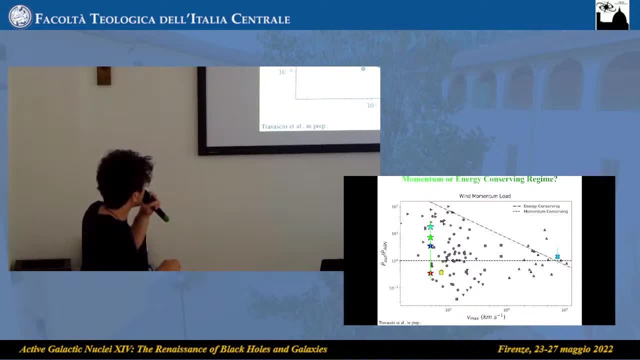 similar to the. we are not able to achieve the energy conserving regime. so I mean, I'm not- it's not concluded by here, but the fundamental things should be constrained electron density for this system, and this would be the next step. I think it's a good idea and we move to the next, to the last talk of this morning we have 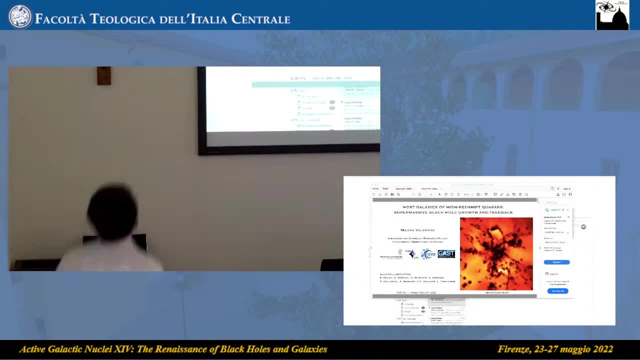 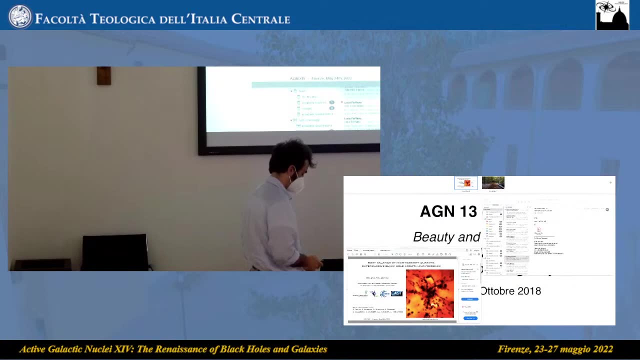 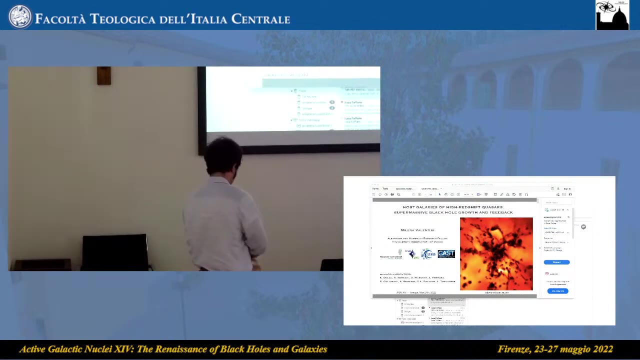 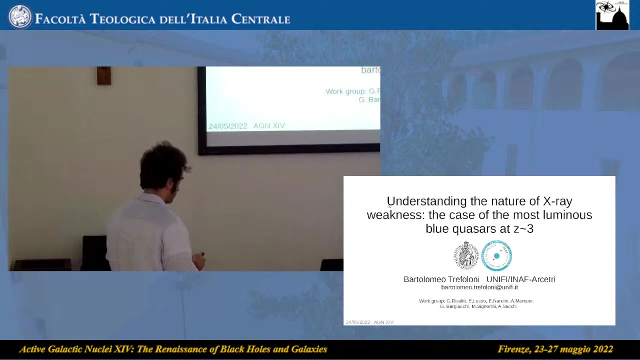 but don't matter, for only talking about understanding the nature of x-ray weakness, the case of the most luminous blue quasars. address shift 3. and let me okay, you, you, you, you, you, can you hear me? yes, no, yes, ok, thank you, thank you and thanks to the computer. 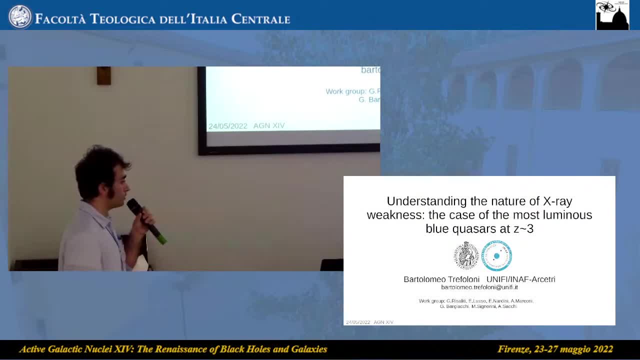 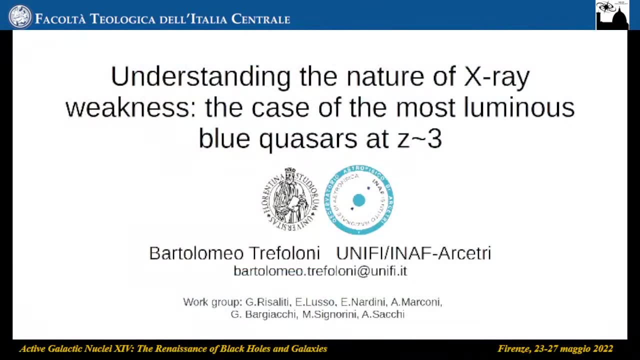 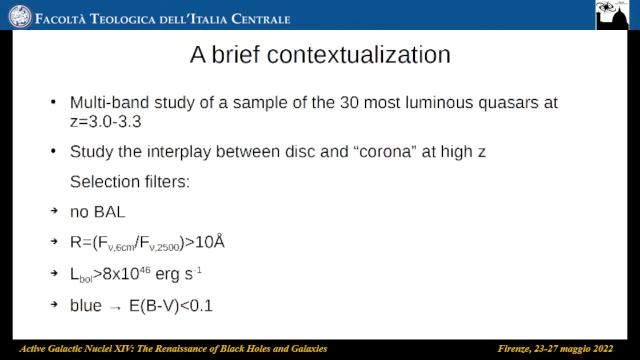 for giving me the opportunity to share my work with you. so my work has been devoted mostly to understanding the major and characterizing the properties of a sample of very luminous quasars at high rate shift. okay, just to give you some brief information about this. 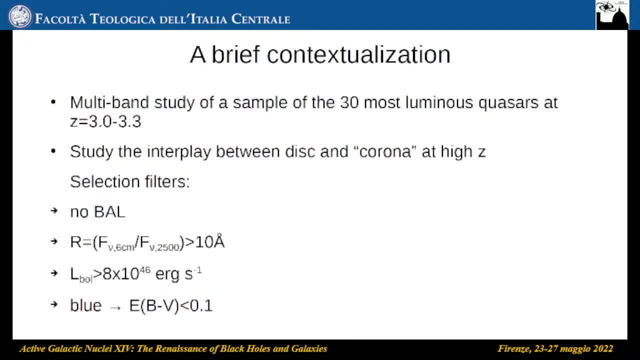 sample. this sample was built in order to investigate properties and the interplay between the x-ray coronal emission and emission from the disk at very high rate shift. so, in order to have a clean view on this topic, we selected those objects in order to fulfill some basic 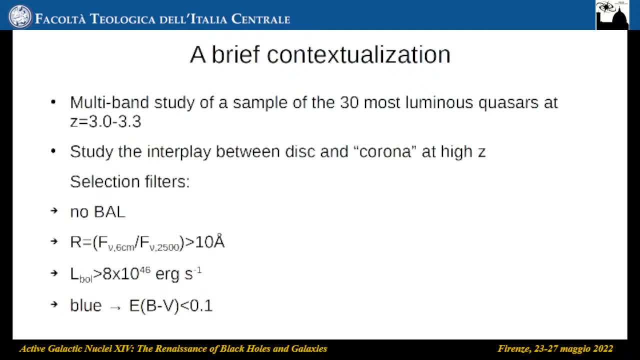 requirements. so, for example, no, the pointer doesn't work okay. so, for example, we wanted to exclude the objects with blood absorption lines, or objects which are radio loud, or even we wanted them to be very luminous. so something like almost 10 to the 47 egg per second. 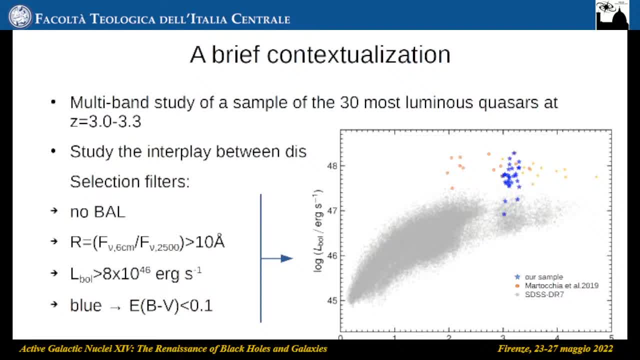 and we also wanted them to be- okay, it works. we also wanted them to be with the leastly affected from emission from yes extinction. so just to give you an idea of where this sample locates with in comparison with other samples, we see that this is located here a thread. 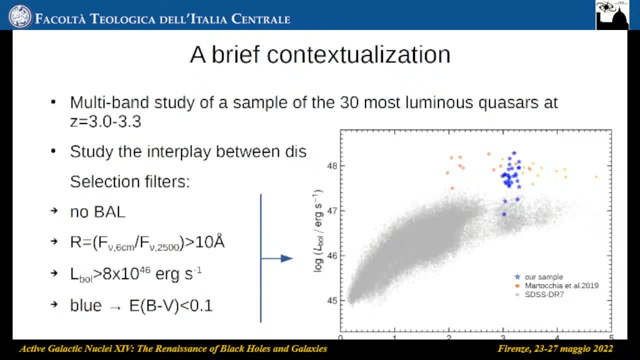 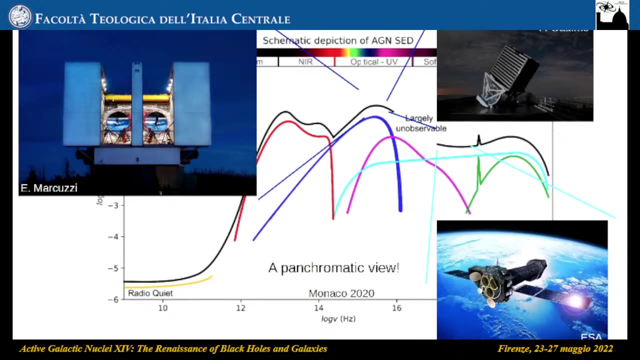 shift between three and three. point three, and it, yes, it- detaches from the main body of the sdc7 release of quizzes in the very high luminous steel of it. okay, uh, no, okay, no, it's very sensible. okay, uh, yes, uh, we embarked on a multi-weaving mission in order to uh sample each possible uh band relevant band of. 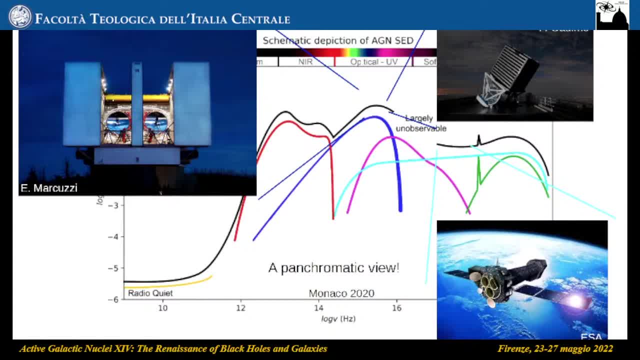 the spectra of these objects. so we have, for example, xmm newton observation, dedicated observations for ipod, we had some archival data from the sdss for the lyman alpha region and we also had the possibility to use the lbt observatory to get some some spectroscopic data of the mg second region and 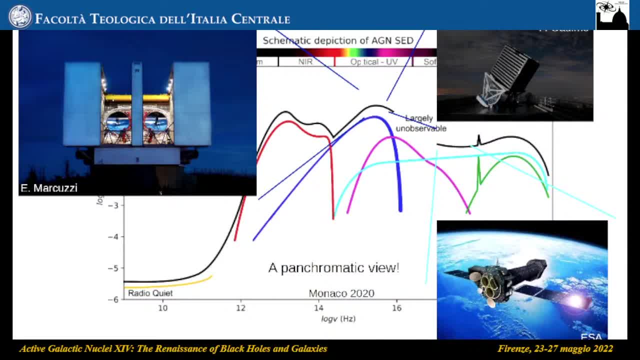 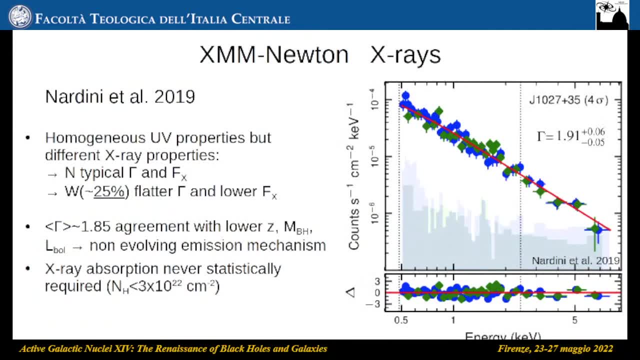 on the optical side. so, uh, just some quick results from previous works. uh, the beginning of it was in 2019, with analysis of xmm data, where the the first surprise happened. so, despite the or very homogeneous degree of properties in the uv side of the spectra, we found two distinct samples. so the main body of 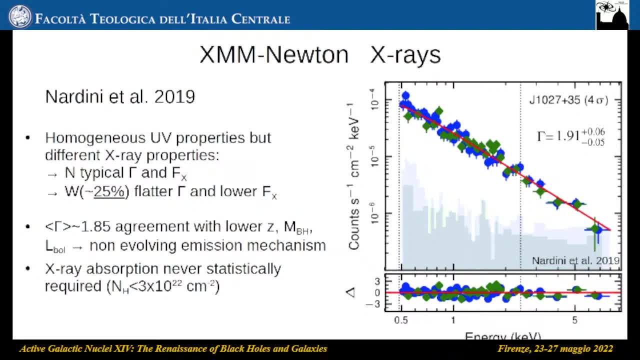 these 30 objects displayed very typical x-ray properties. so, for example, i have a photon index uh, which is 1.9, which is great and in line with what we observe from lower black hole mass quasars and lower red shift and volumetric luminosities. and also we uh, we see that the 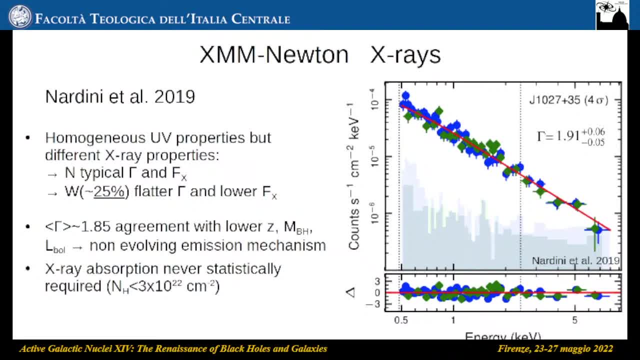 fluxes. the x-ray fluxes are the ones with we would expect for such luminous objects. uh, this is an example of one of those, and we call them the x-ray normal sample. on the other hand, we see that almost percent of the the other objects display flatter photon integers and lower fluxes, and we refer to. 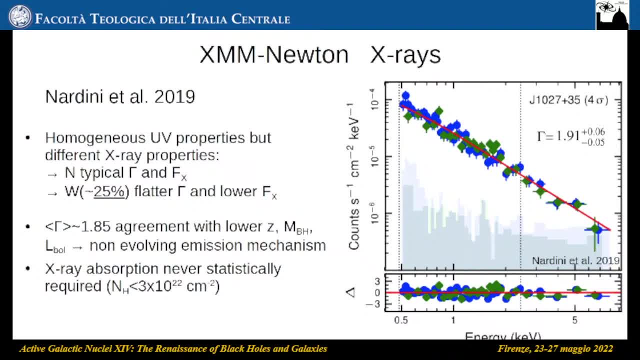 them as the x-ray weak sample. overall, we also see that, as i said, the photon index is in line with what the spectra at lower redshift and this is great because this is telling us that probably the emission mechanism for quasars is kind of ubiquitous through cosmic ages. 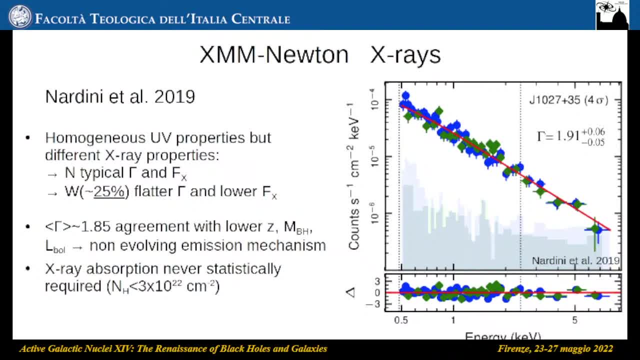 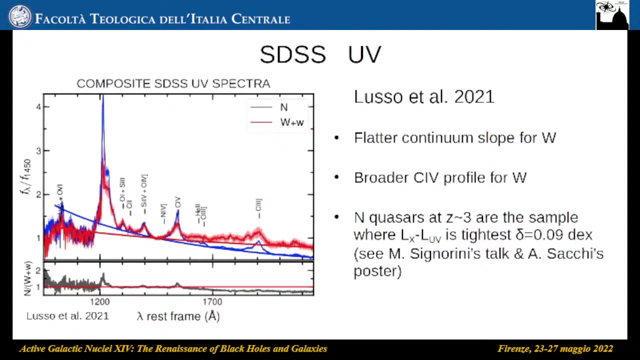 so it makes look like them if they were kind of standard candles and, moreover, we also find that x-ray absorption is never statistically very significant in the samples. we then moved on on the archival data of this low-end survey and we still found some differences because, for example, we find that weak quasars display 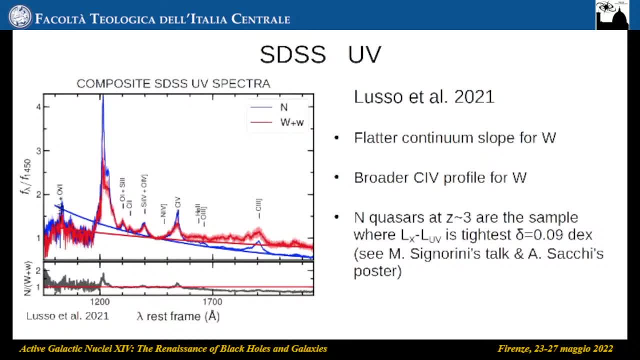 a flatter continuum, whereas and also a broader carbon 4 profile, whereas the normal ones behave very well in the sense that they have a very homogeneous properties and in fact they are part of a sample where the x-ray to uv luminosity relation it's very, very tight. and for other 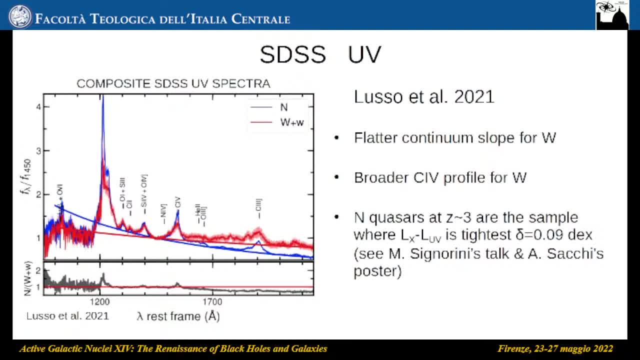 information i will point out in the next slide. so, uh, i will leave that for now and i will see you in the next slide. Please refer to Matilde Signorini's talk and Andrea Sacchi's poster, which are great for this topic. 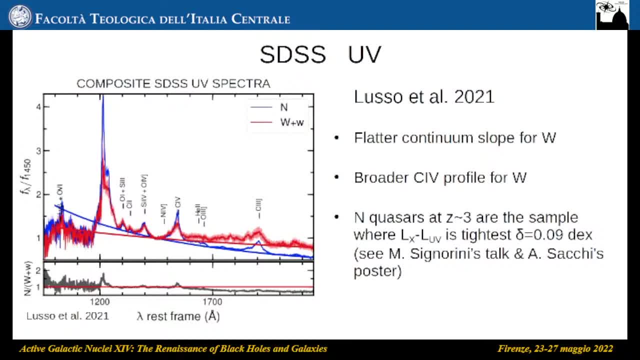 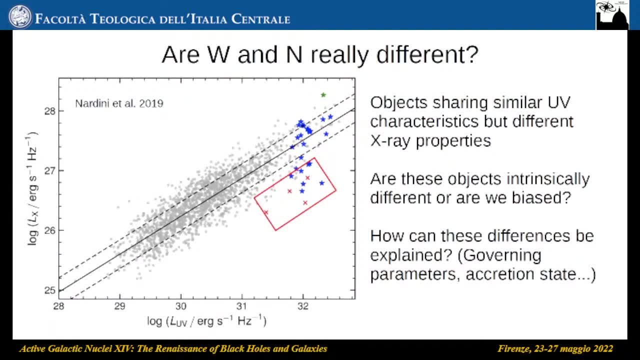 Okay now. what to do now? Okay, so the question I'm asking is: we see some differences between those objects, but are these differences real, So we find throughout all the spectra, or are we missing something? And in case this is real, as we believe, what's the driver behind these differences? 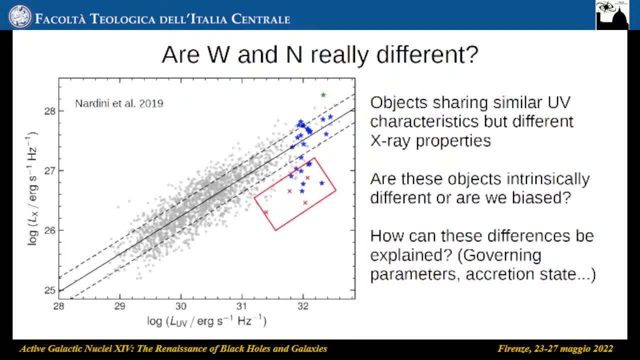 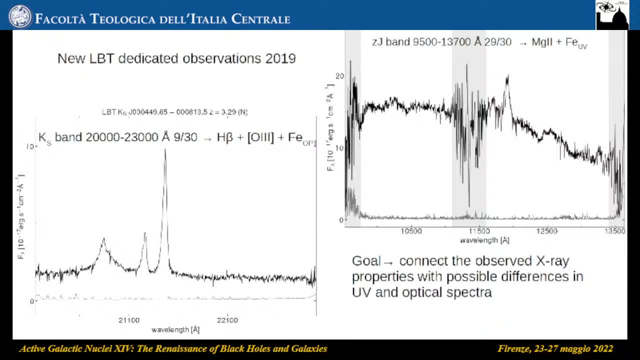 So it is about the governing parameters, it is about the accretion state. So, to this purpose, we embarked on, as I said before, LBTA-dedicated observations and we got some spectra- 29 out of 30, for the ZJ band, which corresponds to the rest frame mg second emission. 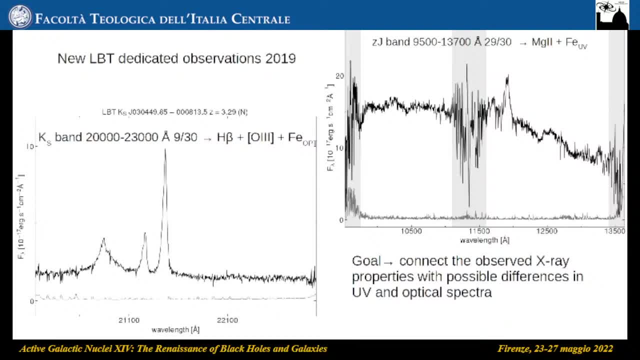 And also only unluckily, 9 out of 30 for the optical side of the emission, which includes the H-beta region and the oxygen third. So the goal is obviously trying to connect the observed differences in the X-ray properties. 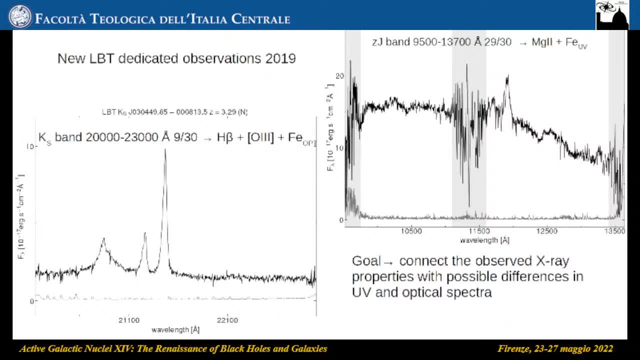 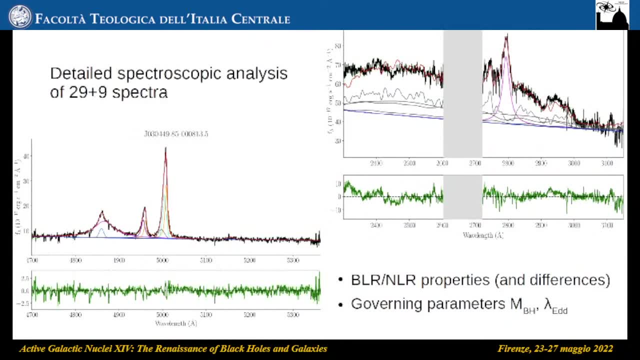 with some possible differences also in these sides of the spectra. To do this, what we did is just to perform a detailed spectroscopic analysis on each of the sources, the 29 plus 9 objects, in order to infer the broadline and also the narrowline region parameters. 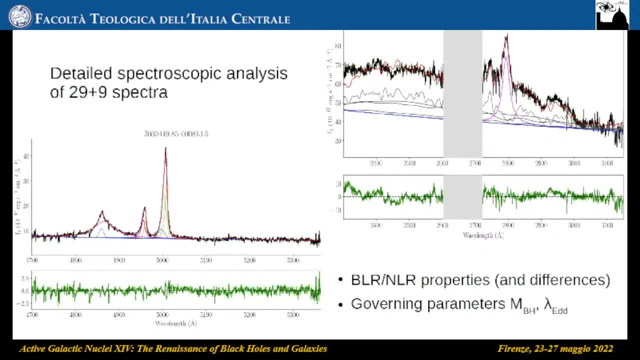 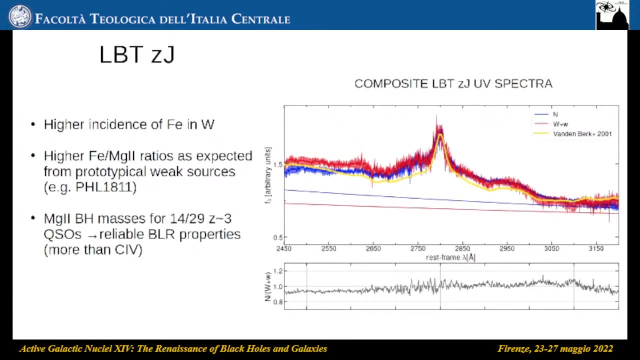 and also the governing parameters, such as the black hole masses and the Eddington ratio, in the most reliable possible way, which is not so easy. So skipping To the results, this is for what concerns the magnesium second region. We found that, on average, the continuum is still flatter for X-ray weak objects. 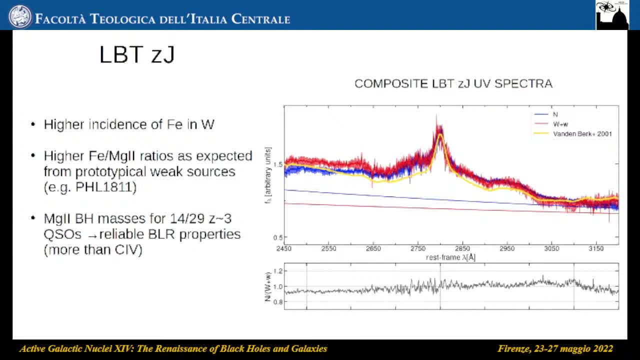 which leaves room for a higher incidence of iron emission, and also a higher incidence of iron over mg second line ratio, Which is what we would expect from some other prototypical X-ray weak sources, such as PHL 1811.. And, moreover, we also were able to derive 14 out of 29 black hole masses from mg second. 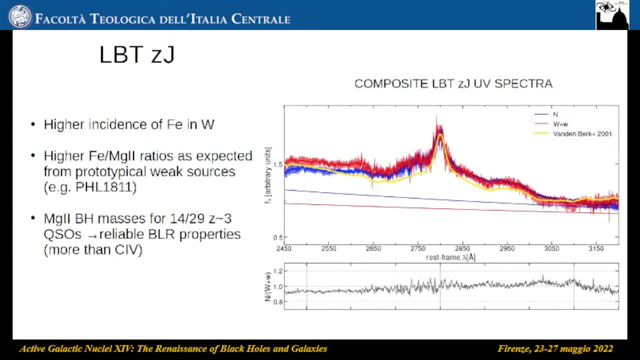 Unlikely other 15,. we were not able to get them because of some bad transmission region, just falling on the mg second line, Which is unlucky, And this is important because so far we only had at our disposal carbon 4 masses. 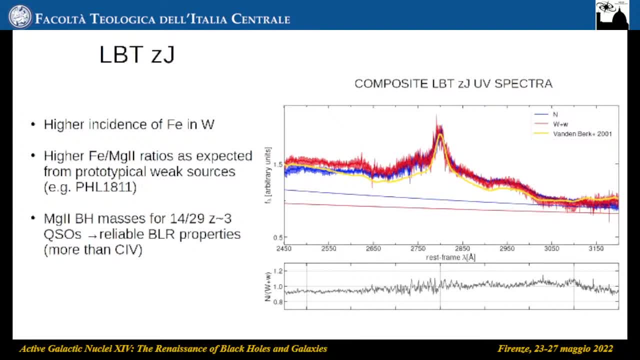 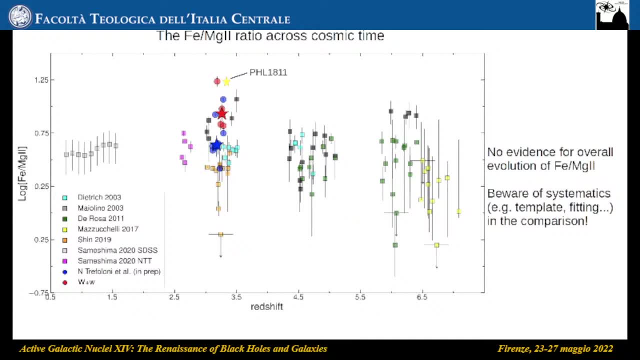 which are not so reliable. So if we look at the iron over mg second emission and we compare these with other literature samples, we see two things. The first is, as I was saying before, there is a difference between those two samples. 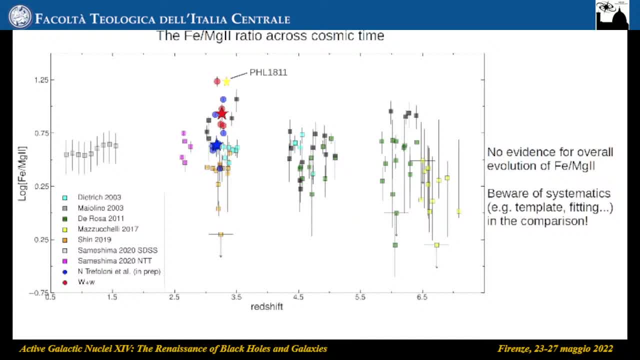 That here I have pointed as blue and red stars And here also with the PHL prototypical source, and I shifted it to a light redshift for the sake of the comparison And the other things that we find is that on average, 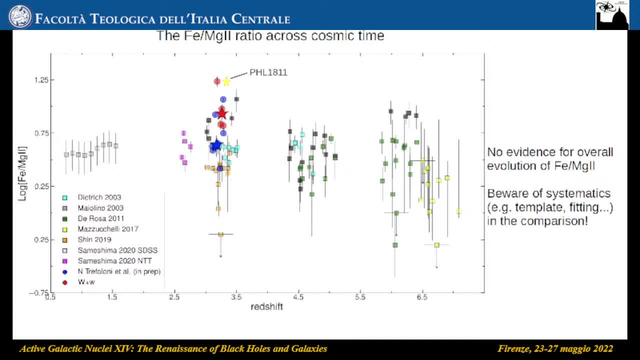 the X-ray normal quasars are in line with the expectations for such redshift quasars, And we don't find any strong evidence for any evolution of this ratio through cosmic times, Even though we must be aware of some systematics that could affect these kind of measurements. 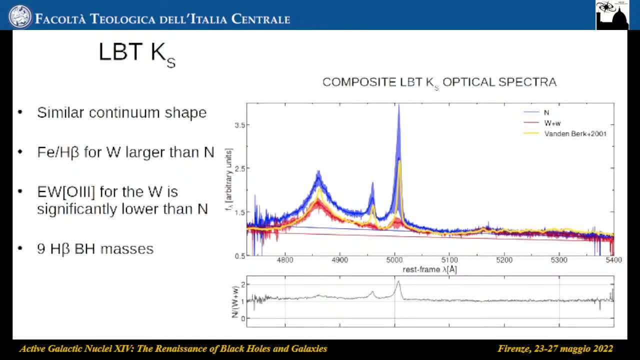 Moving on to the optical side, we found this time that on average the continua are much more similar than what we found on the UV side, And the optical iron over H-beta emission is slightly larger for the weak sample. but maybe the most striking feature is: 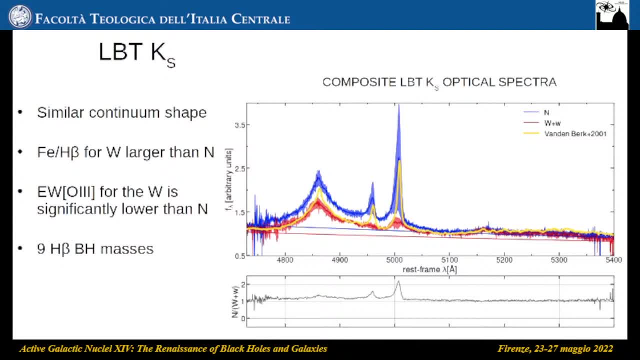 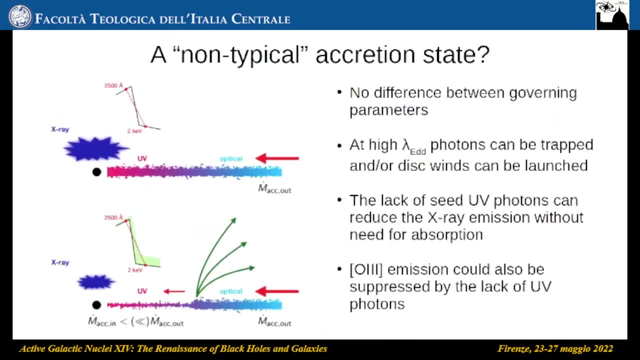 the lack, almost the complete lack, of the oxygen. third emission, which is kind of puzzling. Moreover, yes, we also derived some masses from H-beta which are still more reliable than carbon-4. This, oops, is very sensitive. 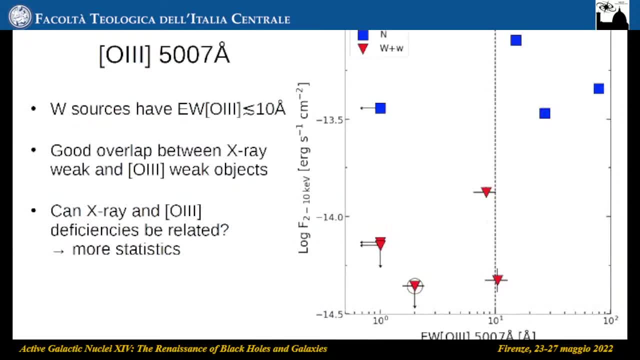 Okay, perfect. This puzzling thing of the oxygen third emission gets even more intriguing when we match the sample with the low oxygen third with the ones that are also X-ray weak. In fact, we get a good overlap if we watch here. 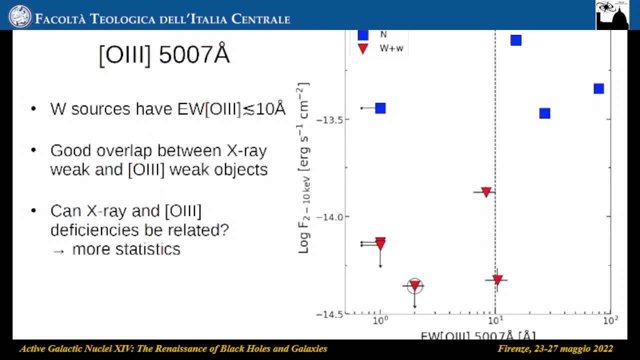 between the sample with low oxygen third emission and the ones with low X-ray weak. Obviously we are talking about just nine objects, so larger statistics is a key requirement for stronger claims. But this also leads us to think that maybe these two deficiencies could be related. 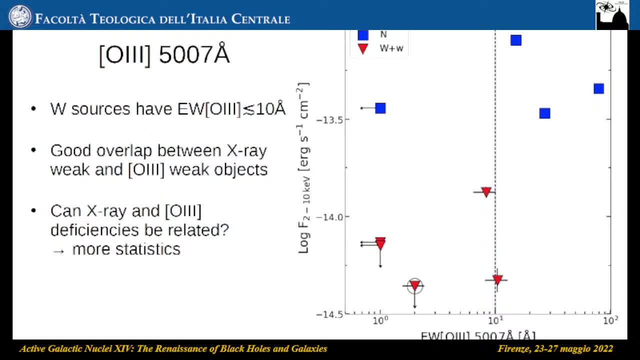 As I was saying before, we derived the black hole masses and we want them to be related in order to be as reliable as possible, in order to also try to get the key parameters for these objects, which are the black hole masses and add-in ratio. 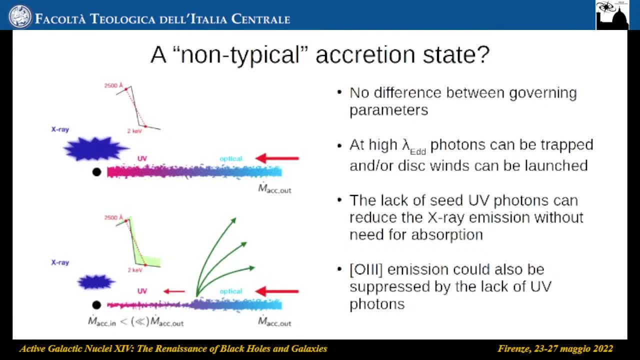 But we did not find any significant difference at all between the add-in ratio and the black hole masses for these two groups of objects, And so they are not likely the main driver of these differences. They all have very high add-in ratios. They all have very large black hole masses. 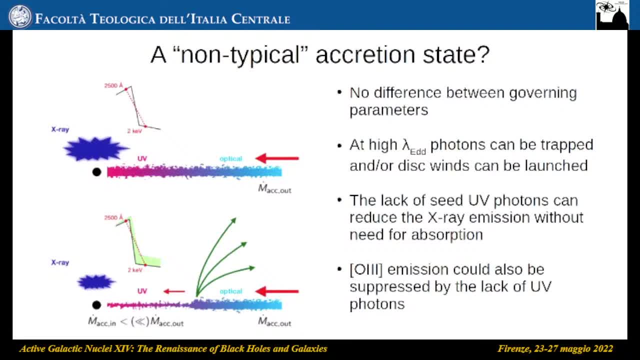 So what could account for this difference? Maybe one possible explanation is the lack of UV photon seeds. We know that for the X-ray emission, we need UV photon seeds in order to be upscattered by an inverse Compton effect to produce the observed power law. 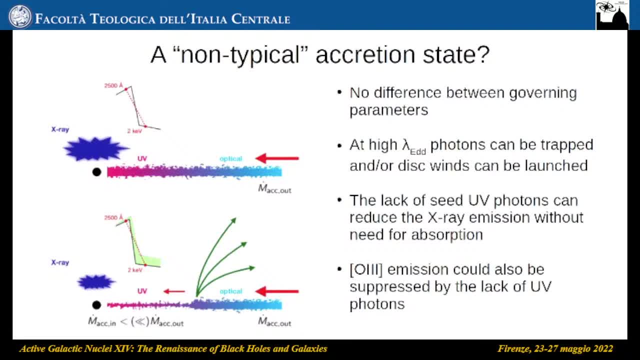 But if a substantial amount of seed photons is depleted, for example from outflowing phases, or they get trapped into the accretion disk when it is higher accretion, then this could explain the intrinsic lack of X-ray emission without needing to invoke 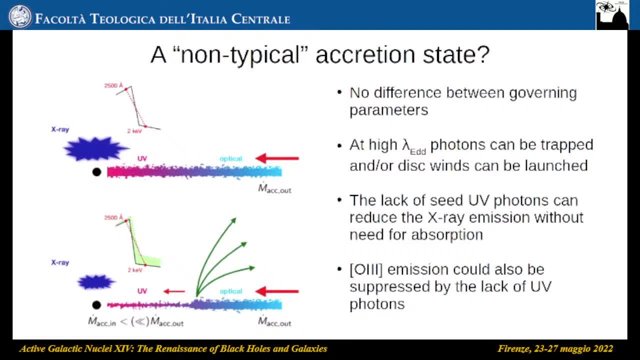 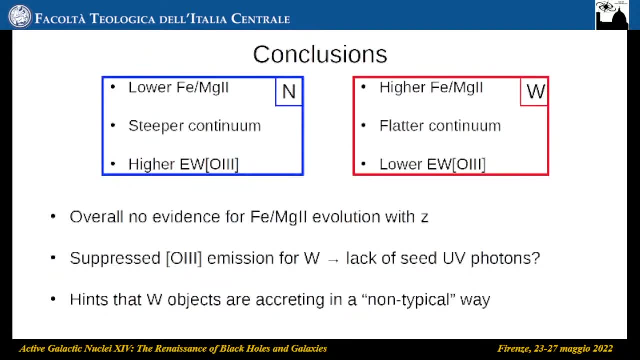 for example, absorption or some kind of shielding, And this could also explain and be important for the lack of the oxygen third emission. So I leave you here with the differences between the samples that we found in this work And thank you for your attention. 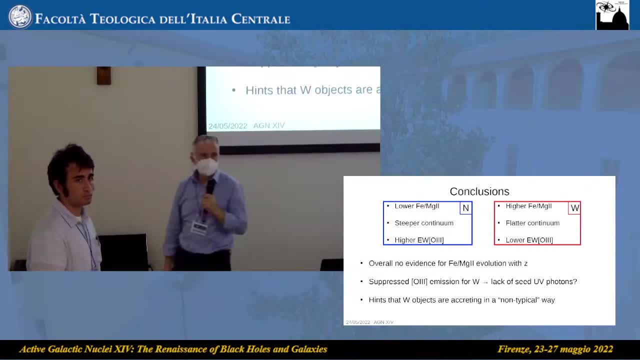 Thanks. Questions for Bartolomeo. Well, I'm a little bit surprised by your result, but I wanted to ask you whether you could measure the Fe2 intensity normalized to the H-beta flux in the optical, and which are the typical values. 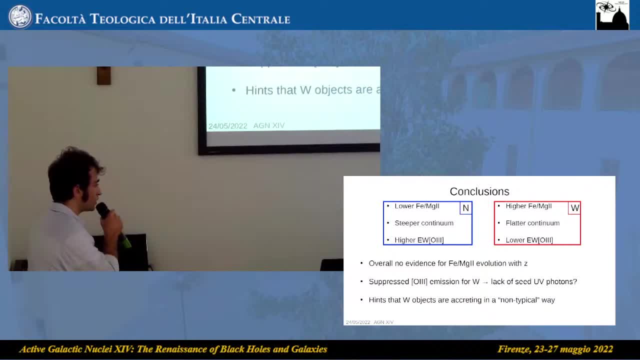 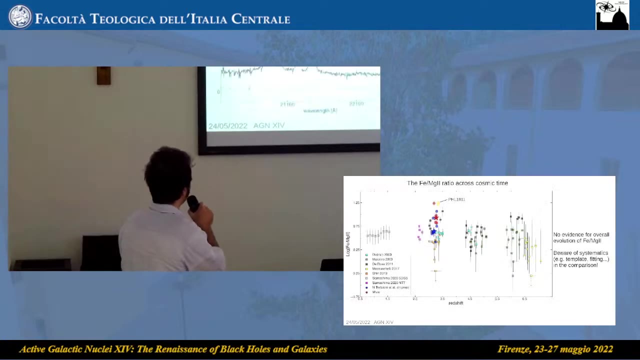 for the two groups of sources. Okay, thank you for this question, But before answering, I have to say that we were not able and the answer is here. Sorry, I go back for a while. Okay, This, Okay, The.